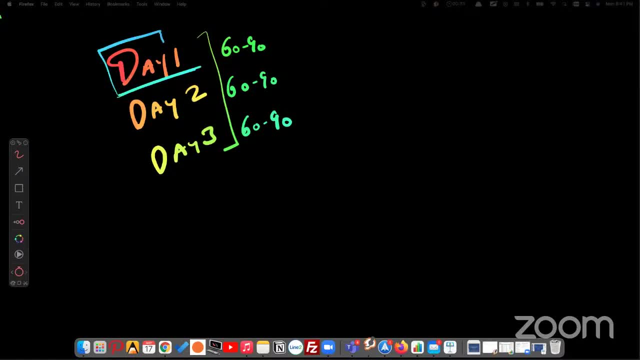 Okay, so this day one I am putting live on YouTube as well. Okay, but day two, day three, if you want, you have to join the zoom meeting which you will be getting after joining this workshop. The link already shared in the live chat: 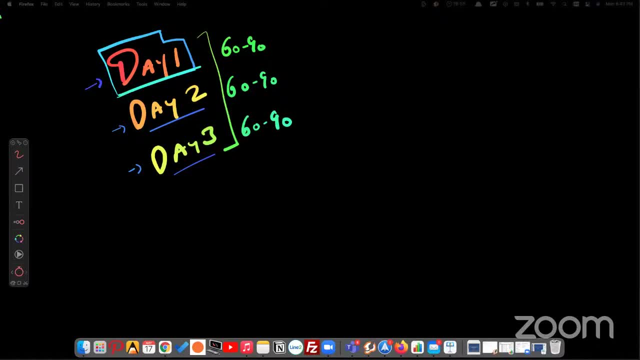 Okay, so let's check for day one today. So let's go. Okay, so we will not waste time. Let's learn the IP address. But before learning IP address, you should know how IP address like evolved or kisne usko banaya. 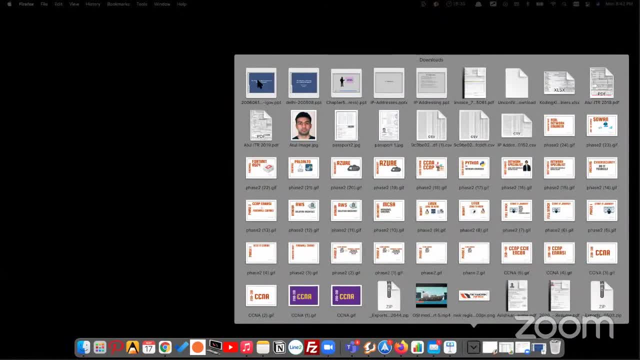 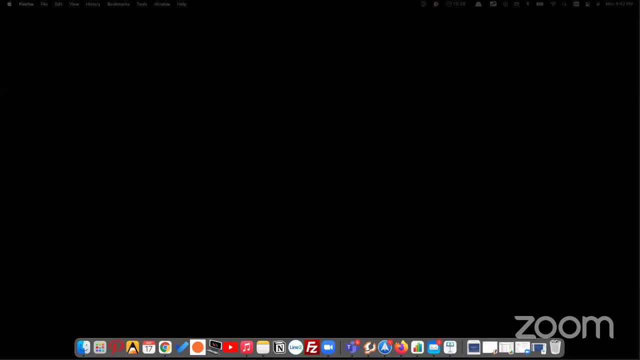 Okay, so this batch I'm going to take in mixed language. I'll going to like, don't worry, if you are, if you understand Hindi, definitely you can also understand this To Hindi: English main mix rakhunga, don't worry. Okay so guys. 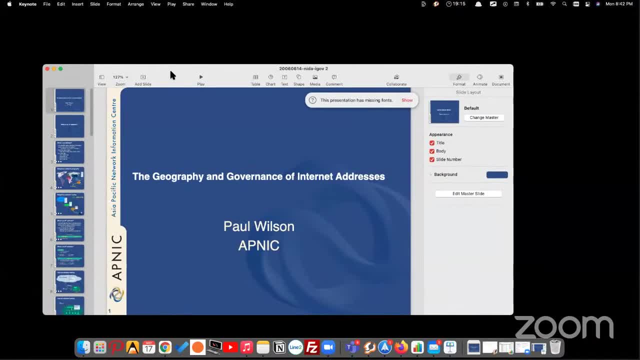 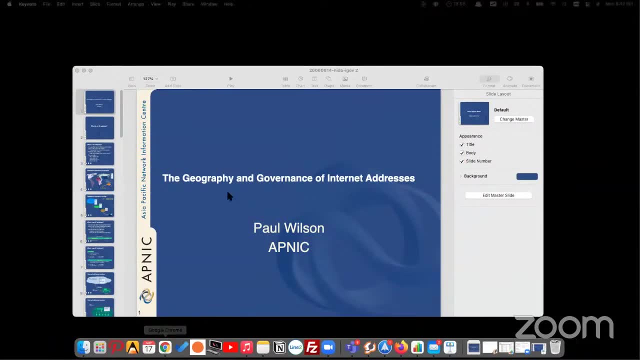 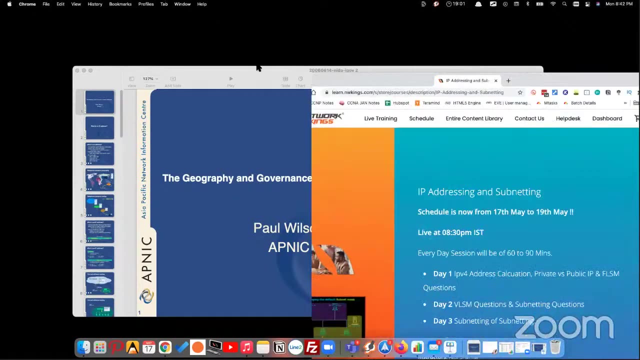 first of all, you need to learn about one company or organization that is called INA, Internet Assigned Number Authority. Okay, so do one thing: how to get the document, So just Okay. so this is the link You can join from here: IP addressing and submitting. 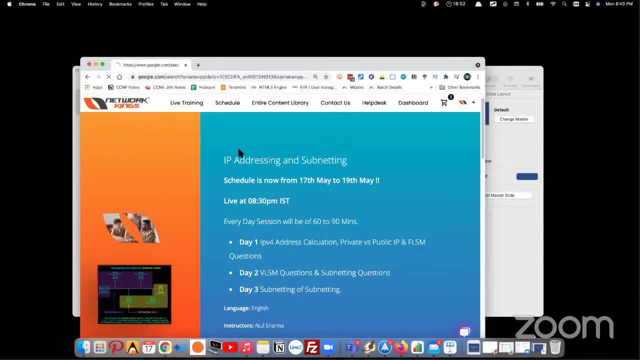 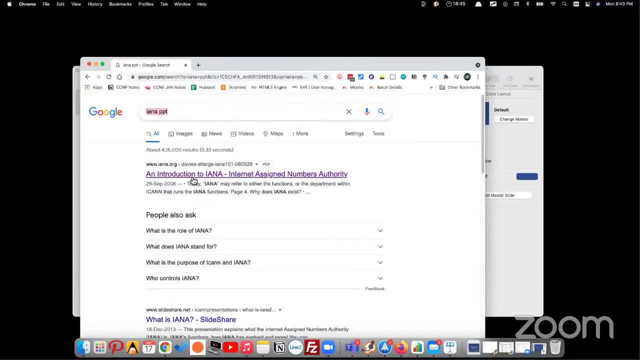 Okay, so I know PPT. Okay, just search this and you will be getting one PPT or PDF document. Just search IANA. What is IANA? Internet Assigned Number Authority. Okay, so I'm not directly, So starting submitting. 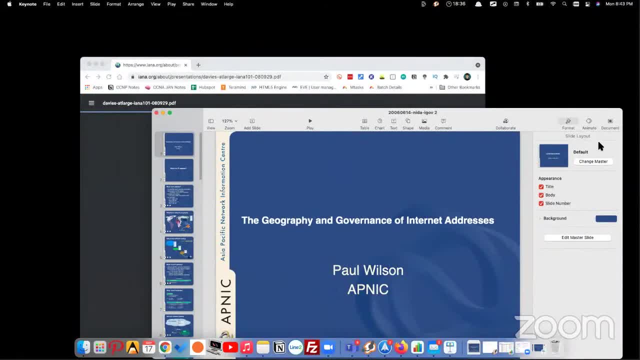 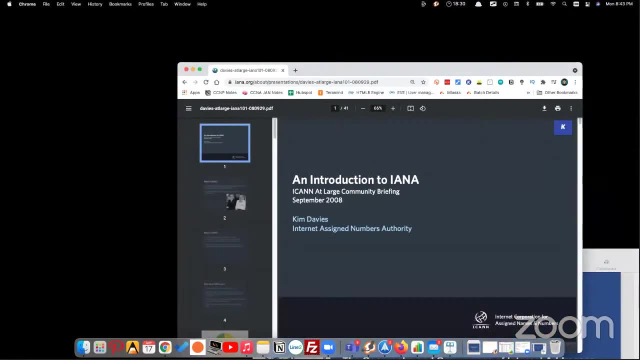 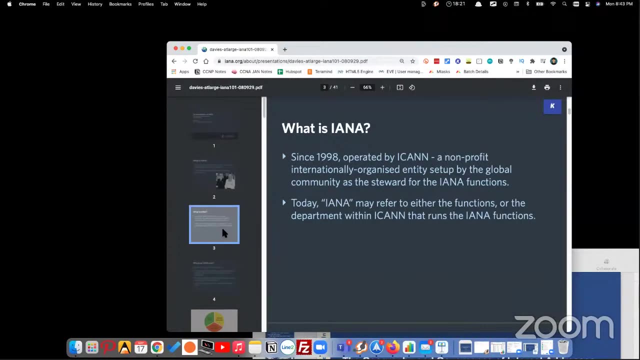 you should understand what is IANA and why. it is it like started IP addressing and all Okay, let's back to some the okay. So what is IANA? So it's Internet Assigned Number Authority, Very simple, Okay. so IANA is actually operated by ICANN. 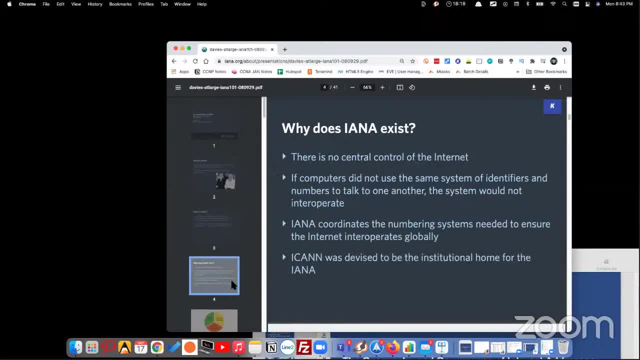 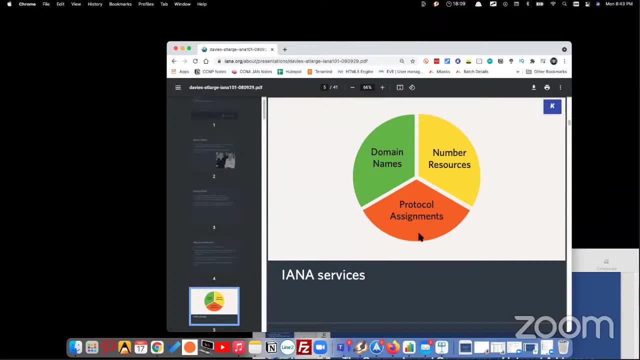 Okay, and this is another organization which is a non-profit organization and what IANA do. So IANA is taking control of three things: domain names, number, resources And protocol assignments. Okay so means all domain names, like, if you buy any domain name like googlecom, facebookcom, 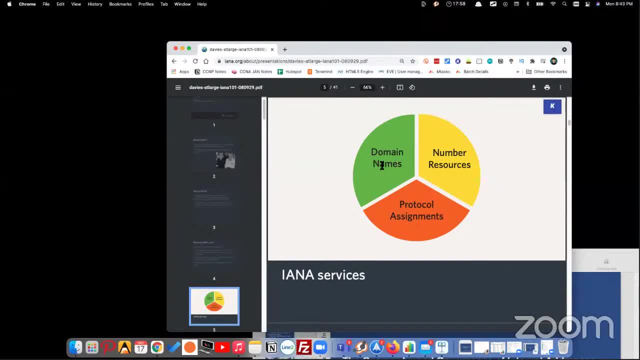 So the- this is called domain, and this all controlled by IANA. number resources, like IP addresses, will be also controlled by IANA, and the protocol number, like FTP port number 21, simple mail transfer protocol port number, is 25.. All this also controlled by IANA. 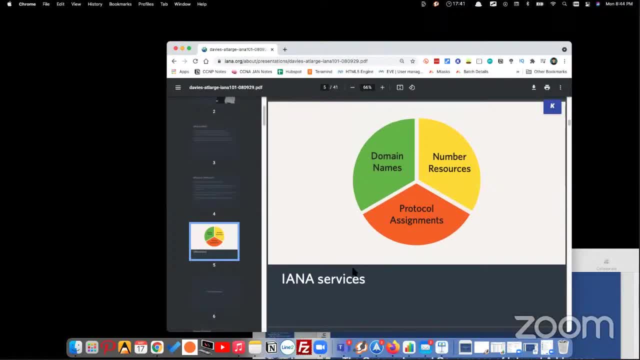 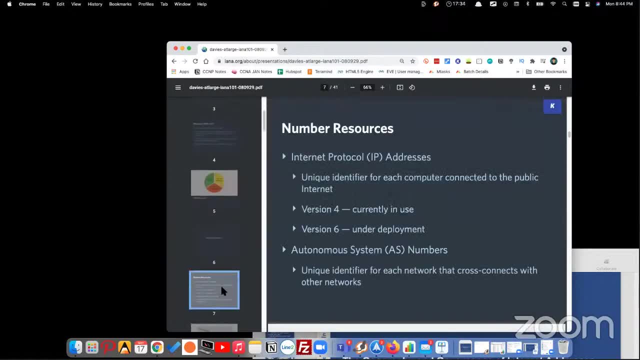 So please remember what is IANA. So IANA is a very big organization which controls Domain names, protocol number and number resources. Okay, so this you will not get in any book, definitely. So what is number resources like if IP address, if we talk about IP address to number resources, may IP 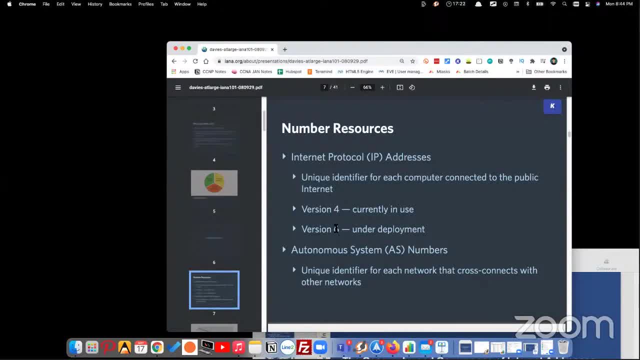 address at a. okay, So in IP all version 4, version 6.. So this is what we call IP address. right, and one another address comes: autonomous system number. If you learn BGP or some kind of these protocol, then you will able to understand. 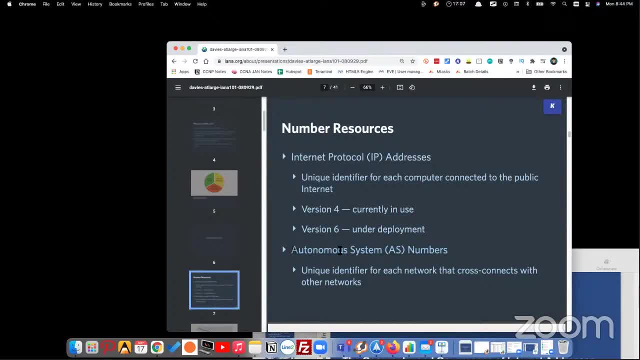 Okay, It's like advanced topic If you are beginner, like if you have not done even your CCN. So just, it's like a number where every company have their own number. Okay, It's like a company unique number, You can say that. and another is internet protocol address which is available in two address version. 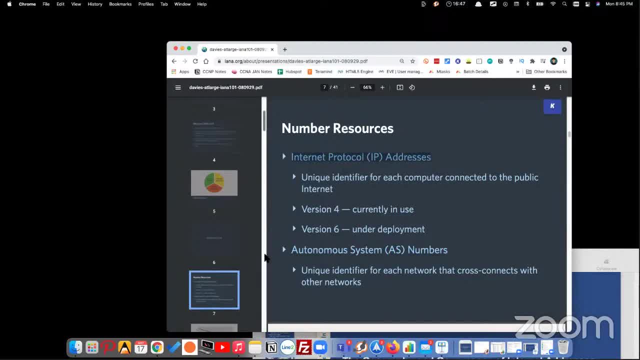 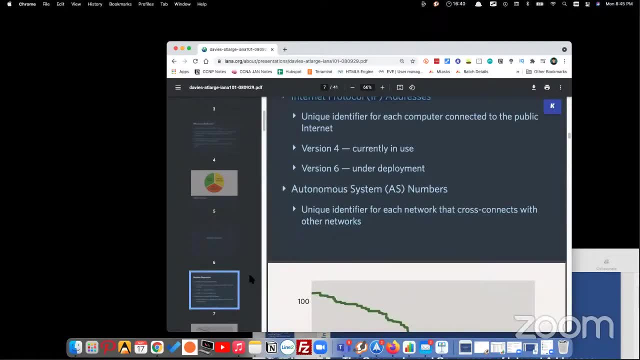 4 and version 6.. So, version 4 or version 6.. You must have heard that there are two types of IP addresses and one is autonomous number which companies use. Okay, So let's talk about. so, Dere, Dere, What, what is happening? 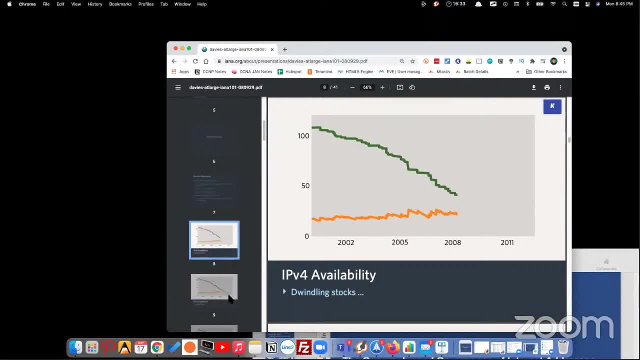 IP version 4 is actually like getting exhaust: matlab khatam ote, jare, Dere, Dere. So IP version 4 is getting exhaust. So this is why IPv6 is also in trend. Most of the big companies are using IPv6 also nowadays, like Jio, reliance Jio is using IPv6. 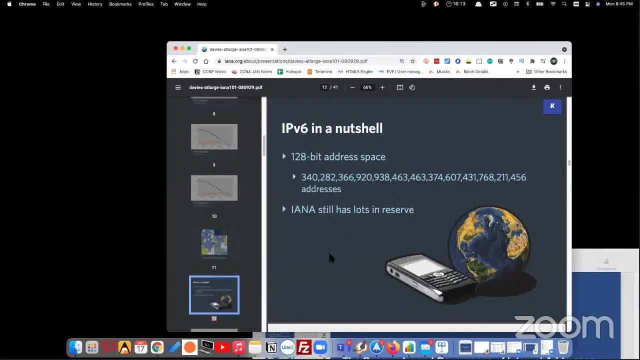 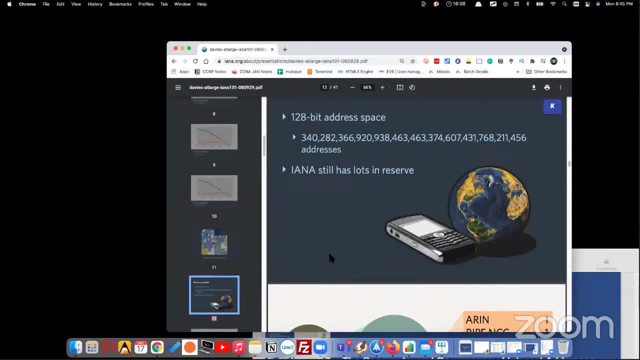 Okay, So IPv6 is a very big number, But here this workshop is for IP version 4, strictly because we need to learn the subnetting, because 80%, 90% companies are still using IP version 4. but I'm going to conduct another workshop. 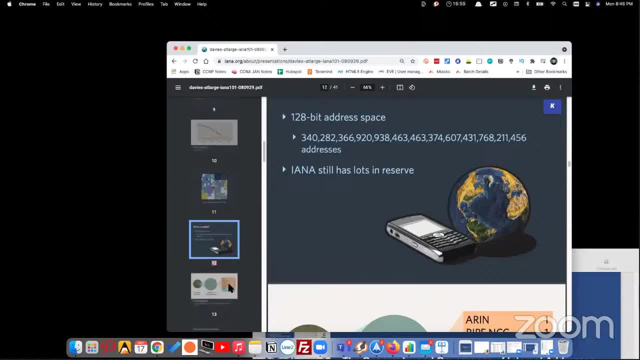 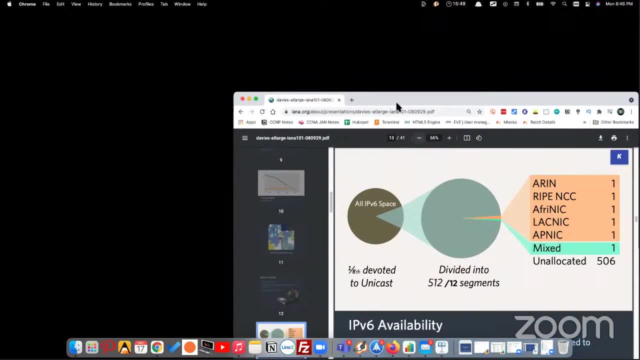 Maybe after a few days for IPv6.. Maybe I'm not sure, but let's complete this first. Okay, So now what is I know? So I told you I know is internet assigned number Authority right? So I know has five. or another organization which is called Erin. 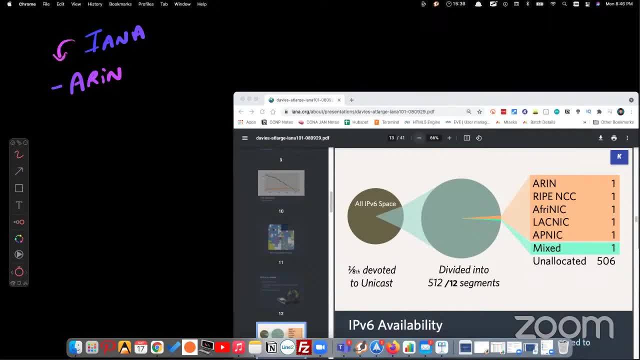 So these are called RIR. So I know K Chote Chote Department say so, just go home. RIR Get a. so I know has subdivisions called Erin, Ripe, Apneic, Latinic, One another. This is Latinic. 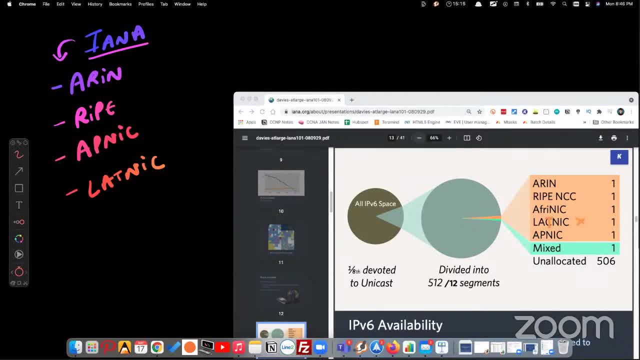 The PPT is wrong. See, I know PPTs are wrong. man, What is happening? So another is Erin Afrinic, Yeah, Afrinic. So what is this? So every big, big organizations means all countries. we, I know, can't handle. 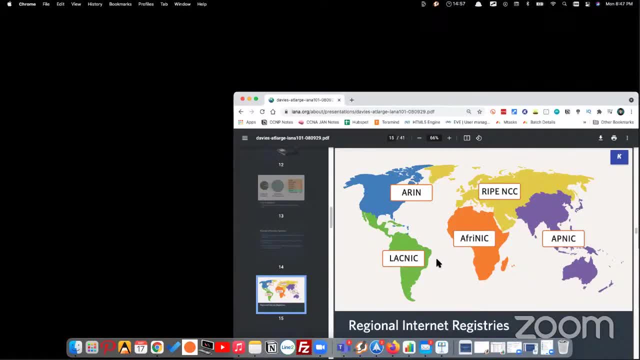 So this is why I know divided into different, different continents. Okay, so you can see apneic, that is Asia Pacific Network Information Center. If you want to buy IP address, you will not buy a forum directly, I know. Okay, so I told you who manages. I IP addresses, all DNS entries. 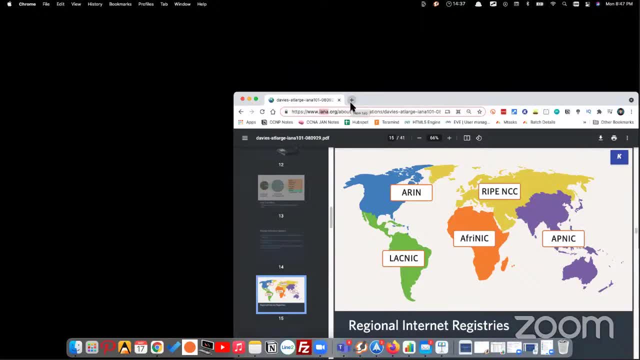 All protocol number and all IP addresses managed by. I know. Okay, clear everyone. Please say yes in the chat. If anyone has any doubt, you can ask me. Yes, everyone, clear, all going good. Yes, Abhishek Ajit, Robin Deep, all okay. 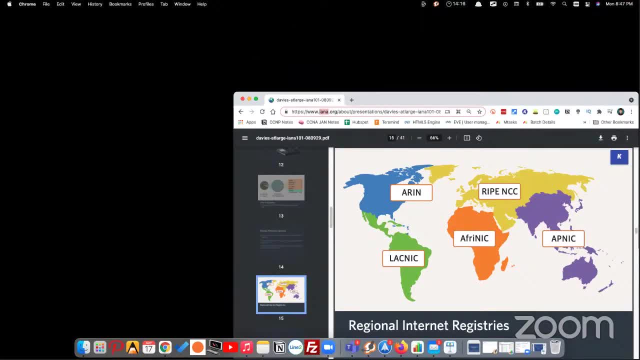 Hey, tell me, Are you writing in the chat? Yes, sir, Okay, any doubt. No sir, All good, All good. Thank you, Okay. Okay, So Erin Lack, Nick Afrinic: ripe apneic- Okay, 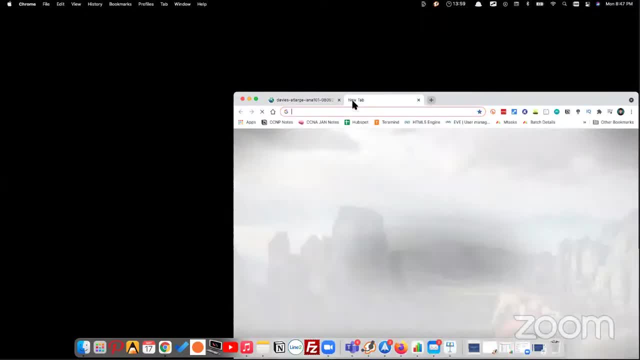 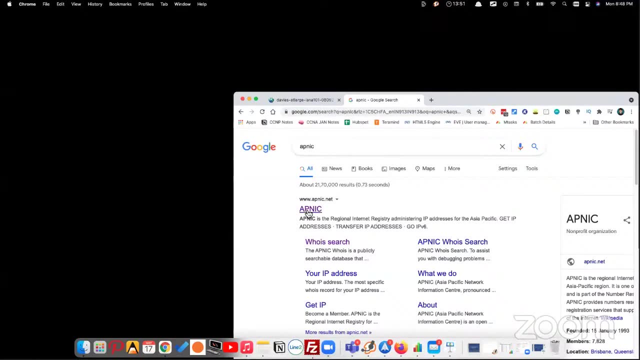 So this is Asia Pacific Network Information Center. You can check one by one apneic. So if you are from India or from any other Asia country, you have to buy the IP address directly from apneic. So you can see apneic, Asia Pacific Network Information Center. 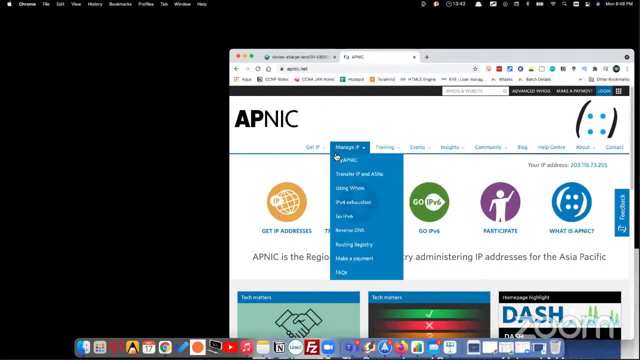 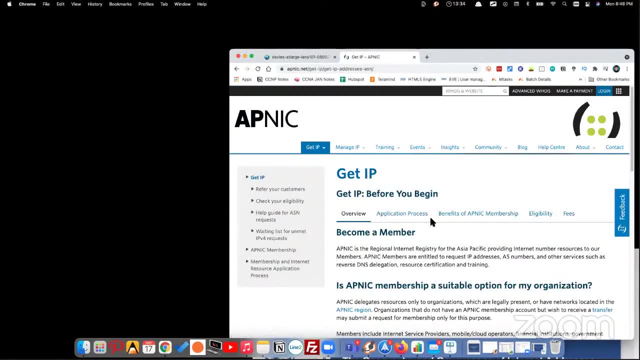 So this is in Australia, So they have office in Australia. So now, if you want IP, you can see: make a payment, get IP. Okay, So when you get a broadband connection, when you get internet connection, you don't pay to apneic. 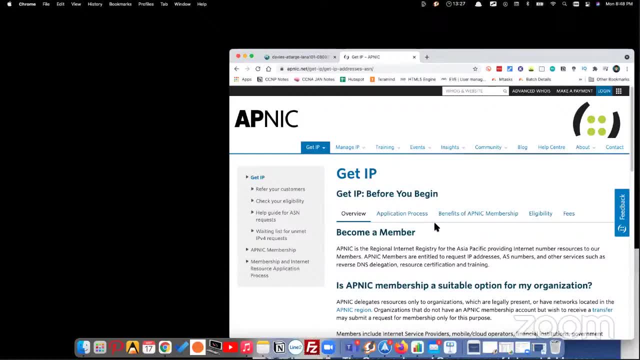 Why? Because your service provider is already paid the fees. So when you put broadband at home, you don't pay for IP Right, Because ISP is giving you its own IP. So ISP is giving your his IP addresses to you. This is why you don't have to. Get from apneic. But if you are a very big organization, if you are a very big organization, if you are a very big organization, you need more than 256 IP address. If you need more than 250, 256 public IP address, then obviously you have to buy it from apneic. Clear. Yes, If you want more than 250 IP, then you have to buy from apneic. You need 10,, 20, 50.. So if you want 10, 20, 50 IP address, you will buy from apneic. 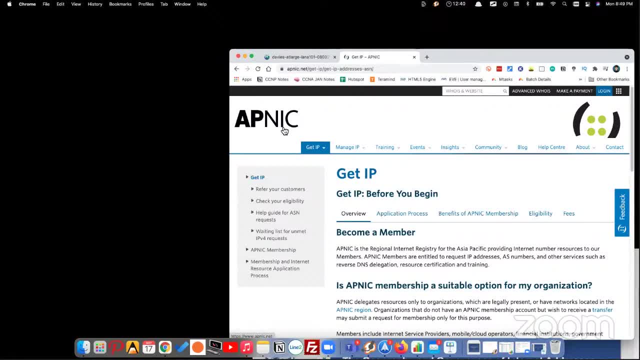 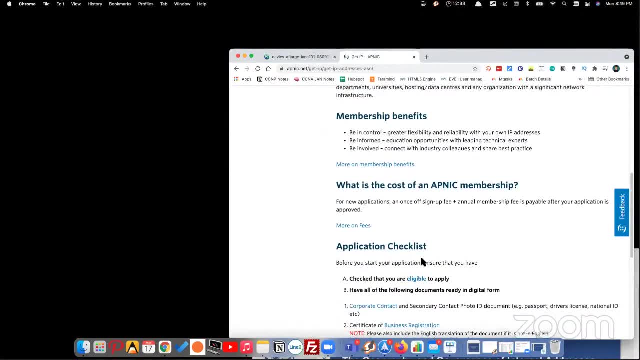 Okay, You will buy from apneic Clear. Yes, sir, Yeah Yeah, Clear. Okay, So you have to be a member. Then, like there is a fees, It's not free. Okay, So start your application now. 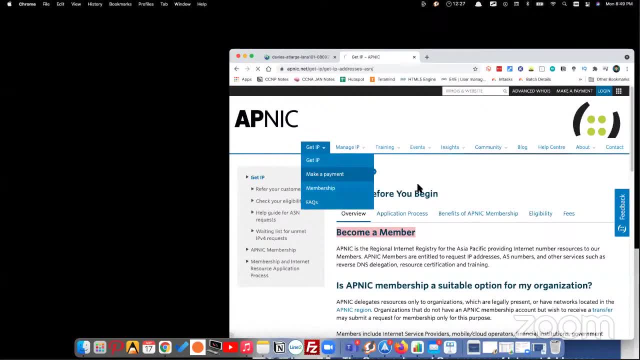 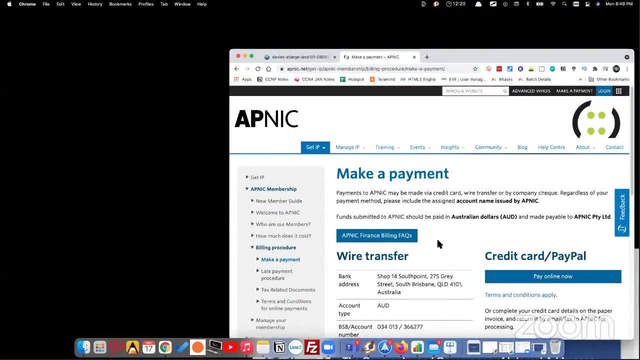 So there is a fee So you can check what is the payment mode, how to get IP address and all So you can see all the details here. So generally 250 IP addresses, approximately 500 Australian dollars every year, So $500, $600 every year. 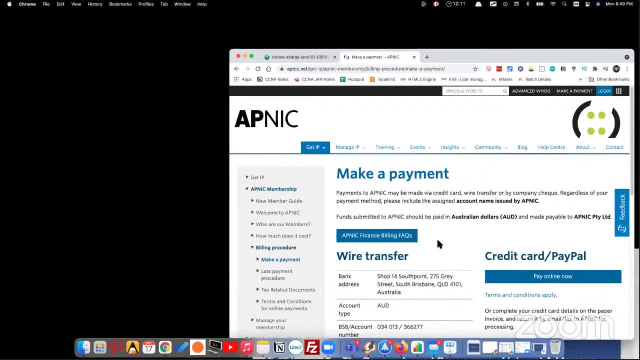 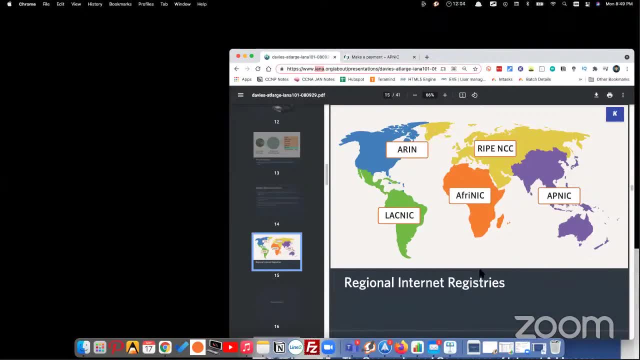 You have to pay every year IP address if you want 256 or some IP like that. Okay, So that is overview. So this is called regional internet registries. If you are from America you will buy from America registry internet numbers. 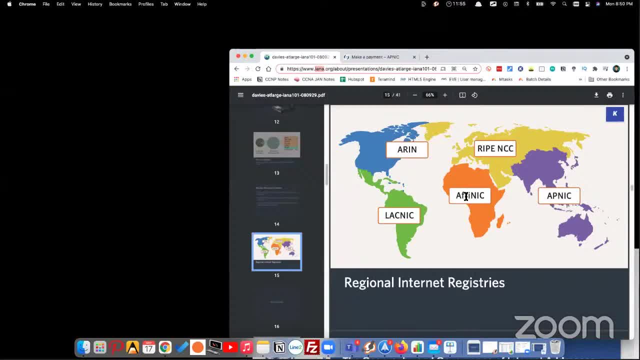 If you are from Africa, that is Latin America. Sorry, Afrinic is for Africa, This is for Latin America And this is for Europe. Okay, So you can check one by one on Google and you will come to know If you want IP from Africa. 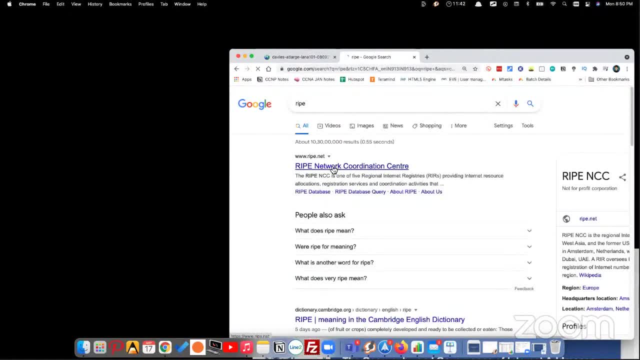 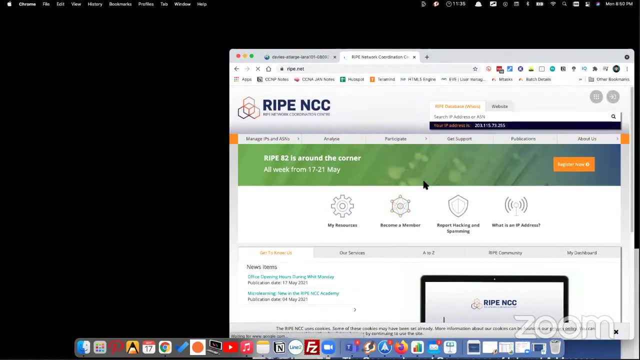 If you want IP from RIPE, then definitely you have to go to RIPE network coordination center. So if you are from Europe or any country in Europe, you have to buy it from here. Okay, So all, all are five RIR. 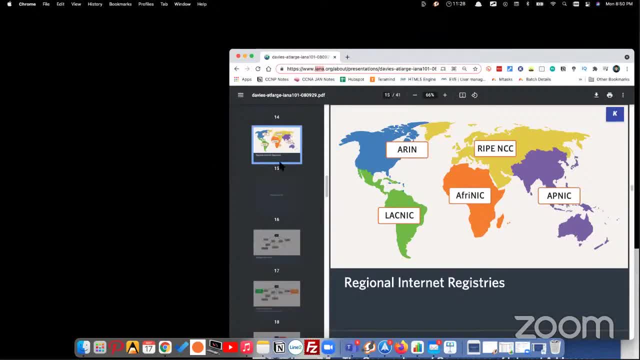 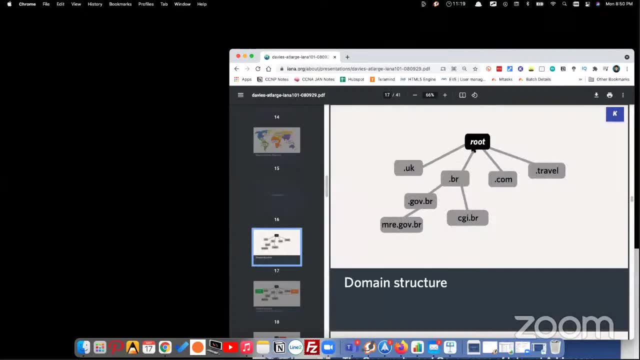 So let's move on. Okay, So IP address, And after that I now also maintain the DNS numbers. So the main, the domain structure, is like that: root Root. All the big numbers are inside this root something. So you can see there are two numbers, which is called CCTLD- country based top level domain. 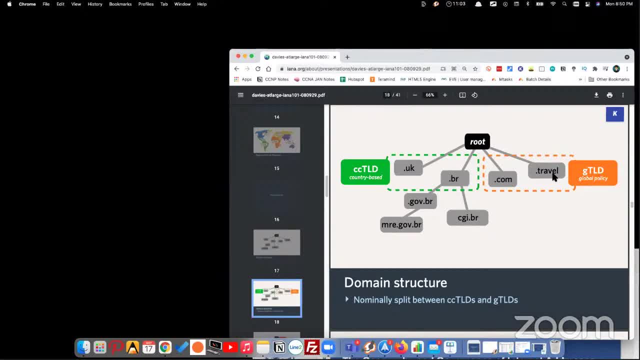 TLD means top level domain and comtravel This is for global policy. Okay, Suppose you buy com, This comes under global policy. And if you buy ukingovernmenteducation? So these are like country based specific. 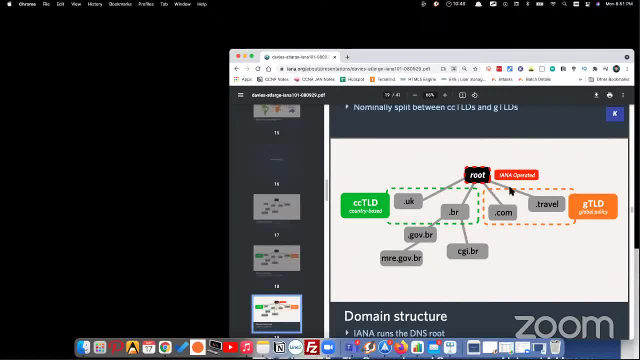 Okay. So who operates? Aina operates this global policy numbers like comtravelnet. So all these domains are operated by Aina, managed by Aina, But all ukbrazil or in all are controlled by countries. Okay, 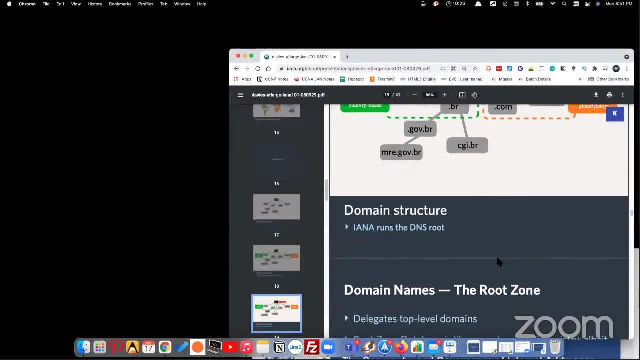 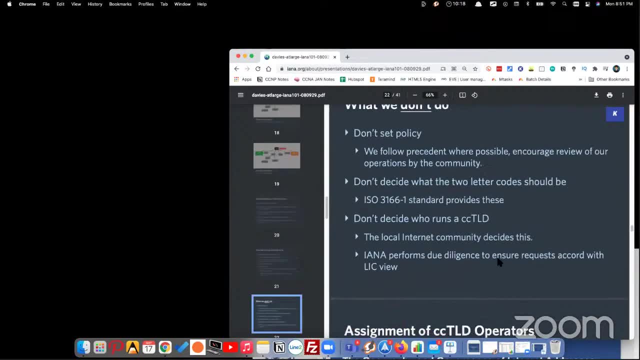 All are controlled by country DNS servers, not by Aina. So Aina is a very big organization again. Okay, So this is all basics. Six things I am telling you might be. you will not get directly. I am showing you from the Aina. 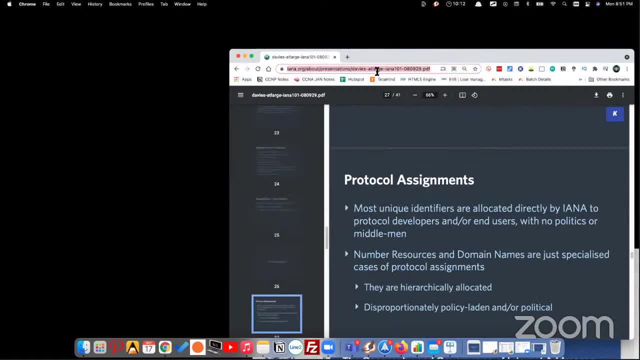 Okay, It's like very big organization And you can still download this PPT also, So I will put a link in the chat for those who want to understand. Okay, Yeah, So we will definitely come to submitting, Don't worry. 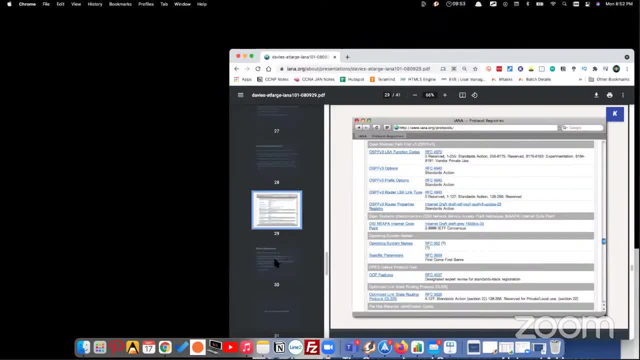 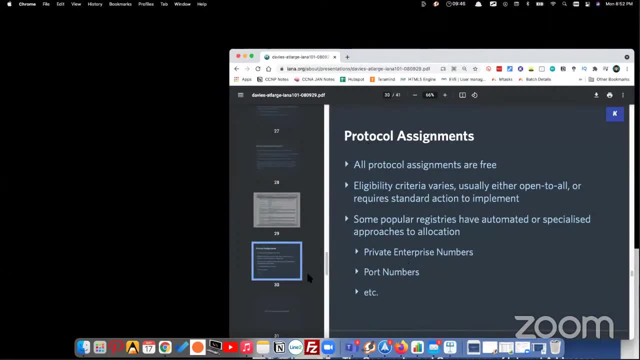 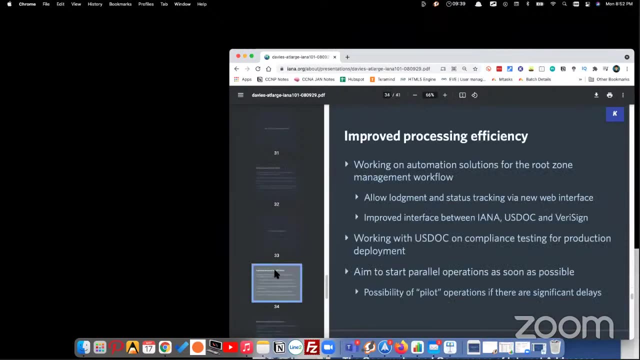 Okay, And protocol numbers, like the protocol number, FTP and all these protocol numbers are also assigned by Aina Okay. Port numbers or these numbers also assigned by internet assigned number authority. Sir, registered port number is also assigned by Aina Yeah. 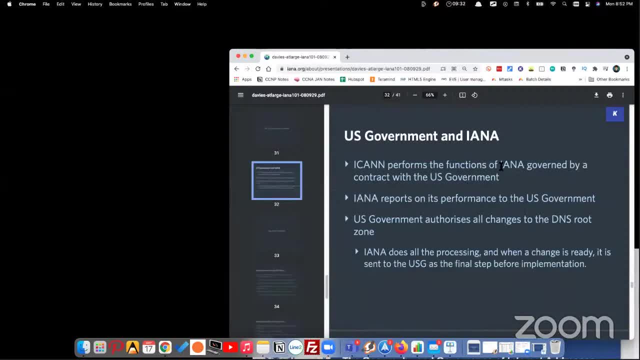 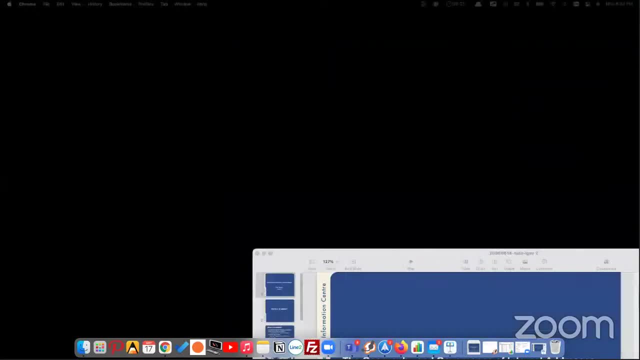 Yeah, Yeah, All registered ports are registered by Aina only. Okay, sir, Okay, Yeah, Okay. So this is all. Now you come to know, like, what is Aina? Okay, Did you understand, sir? Yes, sir. 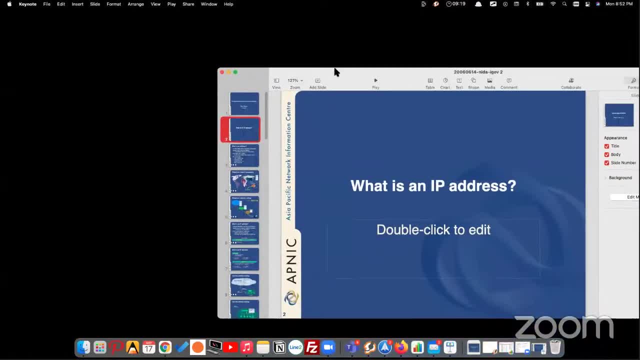 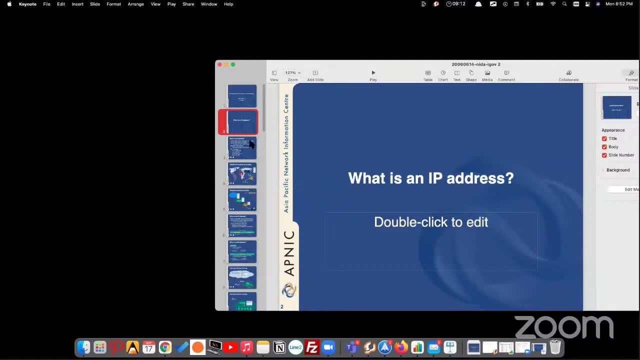 Yes, Yes. So let's talk about IP address now, because IP address is managed by Aina. Okay, So that's when I told you about Aina, because IP address is all managed by Aina. This is why you should understand what is Aina and when you will be going to join any 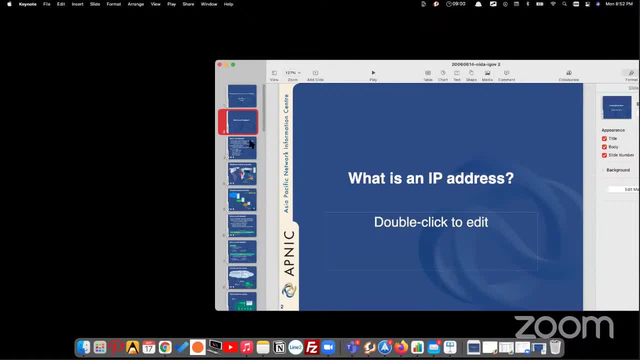 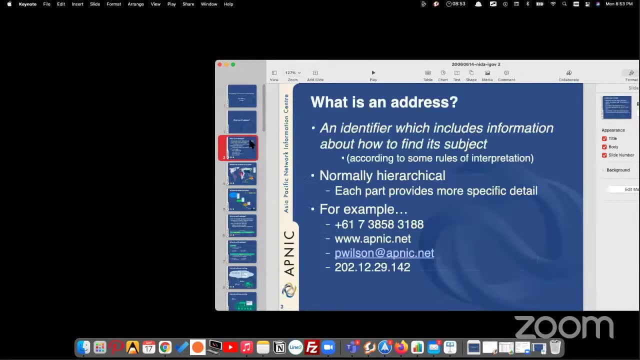 company as a network engineer, cloud engineer, system engineer, Linux, whatever. So you should know, like, how to get IP address, how IP address works. This is why I have explained you. Okay, So this is IP address now. So IP address is a unique identifier. 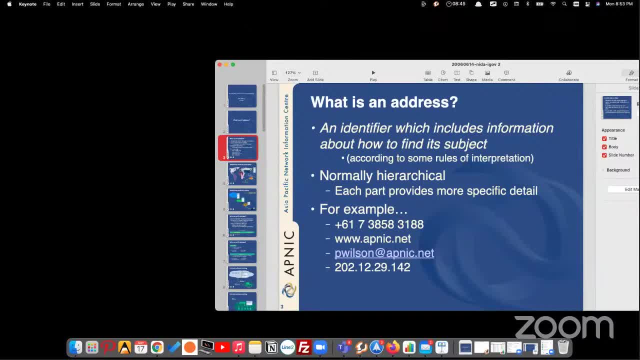 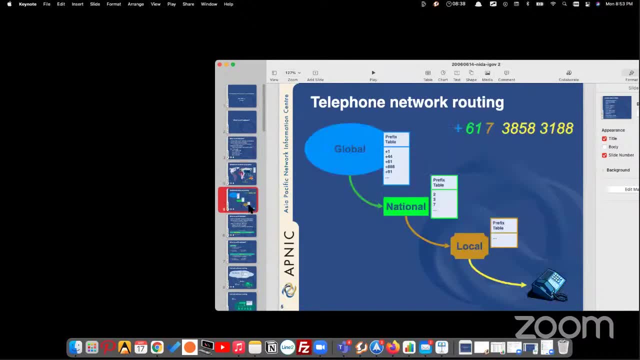 It means there is unique ID of every device, So it's like a unique identifier. Every device in this world needs IP address to talk with another device. Okay, So like, if you call someone, suppose you are calling from India to Australia. Okay. 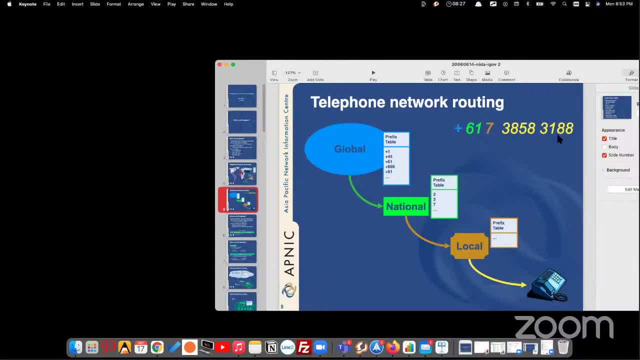 You need a country code, then again a national code, then you type the number. So same like you dial someone and another person gets dialed. Okay, a dialed ring, right, so uh, so that you guys can talk to each other. so same like: ip address is a. 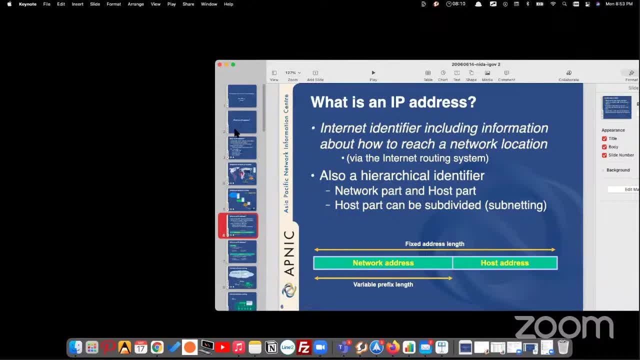 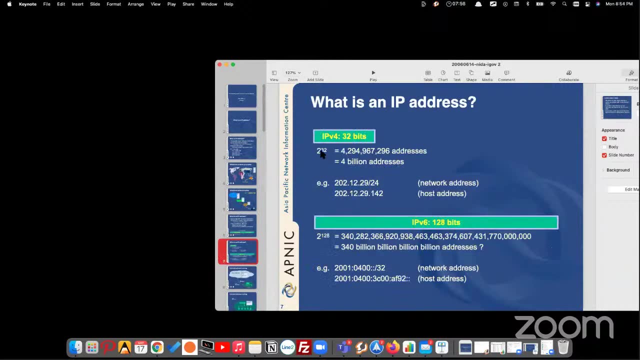 unique identifier, like internet identifier, but full form is ip address. okay, ip address, okay. so all internet routing system, all internet devices, works on ip address. so let's talk about in short. so what is ip address? it's a very big number, so it is available in two variants: ip version. 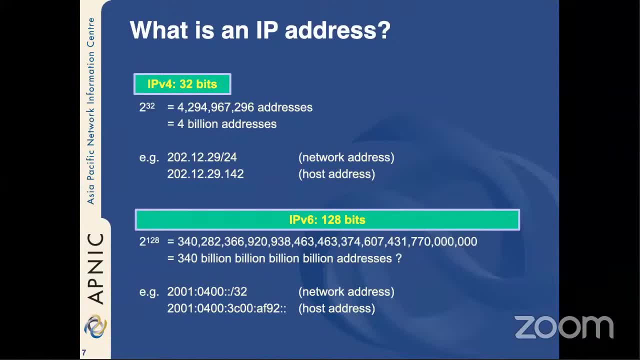 so, and guys, i don't actually read ppt, this is not my style, but still it's very good, informative ppt, so let's understand. so now you can see: ip version 4 is 32 bit, which comes around 4 billion addresses, but this is almost exhausted and now ipv6 have almost 3. 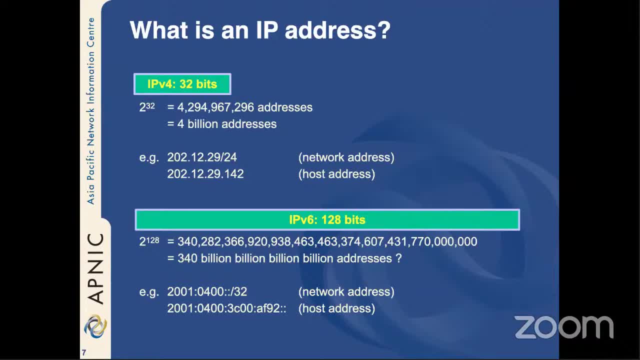 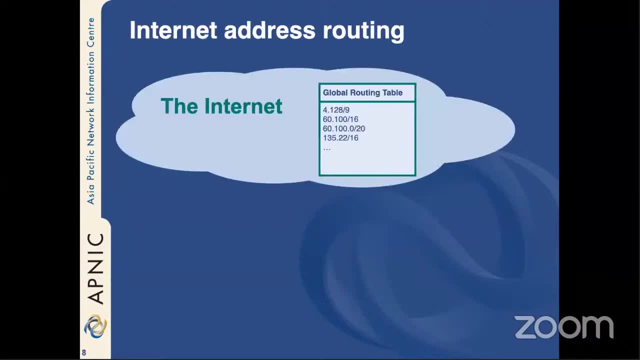 billion, billion, billion ip address. you can't even count that. it's a very big number. some people call this undeclian also and and declian because. so now what is happening? internet has very, very big, big routers. okay, all internet has a very big routing table. 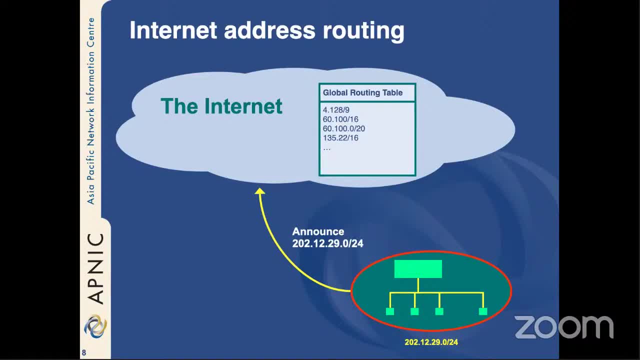 why we need ip address. all internet has a table called global routing table. it is also known as bgp table. there is a protocol which is very famous- bgp border gateway protocol. so you can understand in a very simple language. internet has a table called global routing table and when you announce 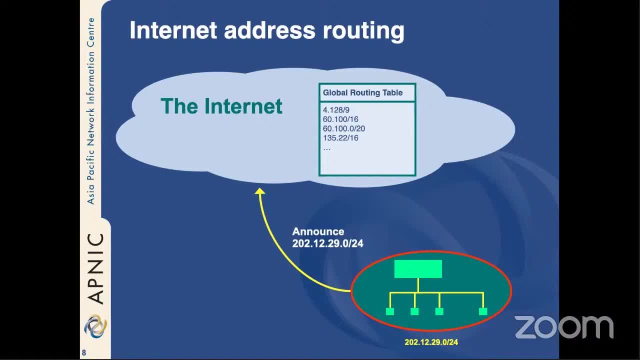 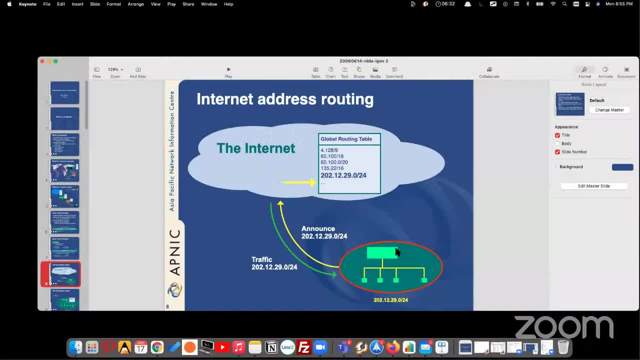 your routes what is announced. you can see there is a small green color circle with red line border. just see the downside so you can see here. suppose this is your company and you have few servers, like you have a. you are a company like facebook or any company, or maybe you are yatracom or railwaycom. 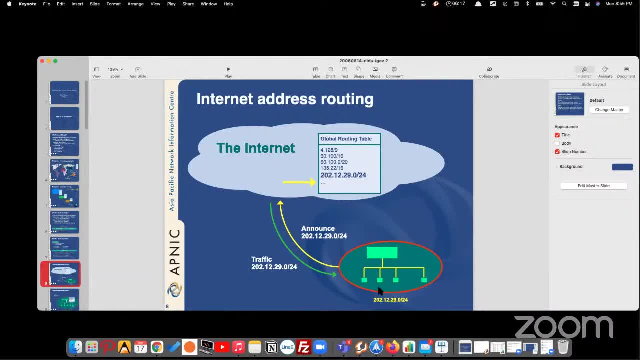 or any website you name. it suppose you have your servers so you have to share your ip address. you are, you get this ip address from where apnic, so from where you bought this apnic and you are going to announce you are going to share your ip addresses with global routing table. why, when you 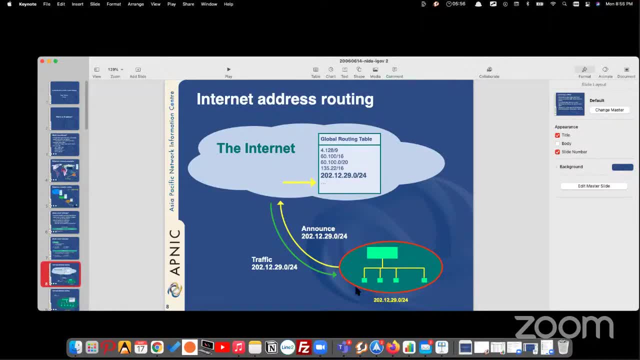 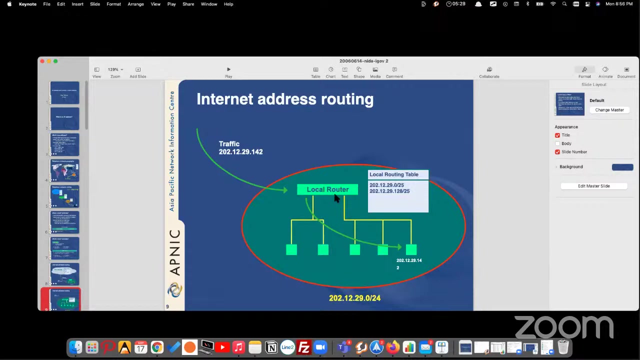 announce this: 2, 0, 2, 1, 2, so this is ip address. when you announce, then whole internet will come. some servers, okay, you have some servers. global routing table, routing to a router: okay. so in short, you are going to push your information to a router, then router is going to share your information to the global. 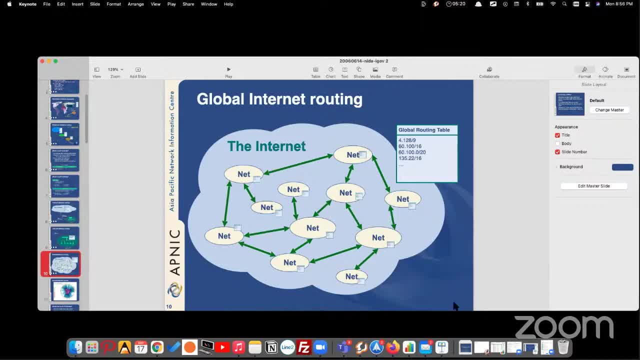 internet. so you can understand like this: so you push from one router and it will go, because internet is a network of network. so what is internet? internet is network of networks which are managing global routing table. all big companies, routers, have global routing table. this is why, if you sit, if you take atl connection, if you take geo connection, you can open. 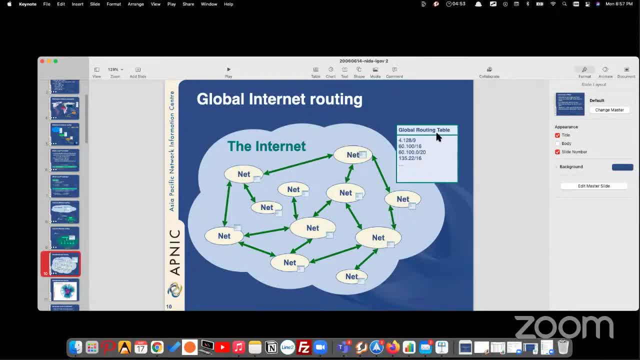 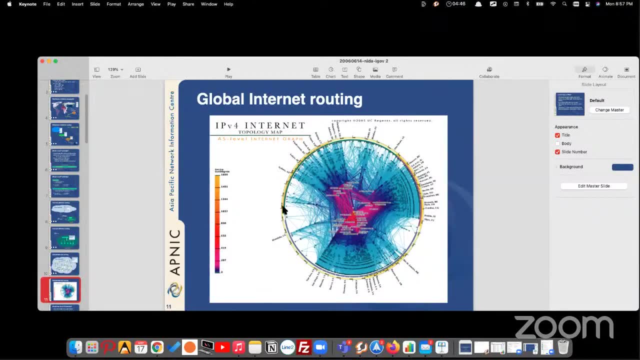 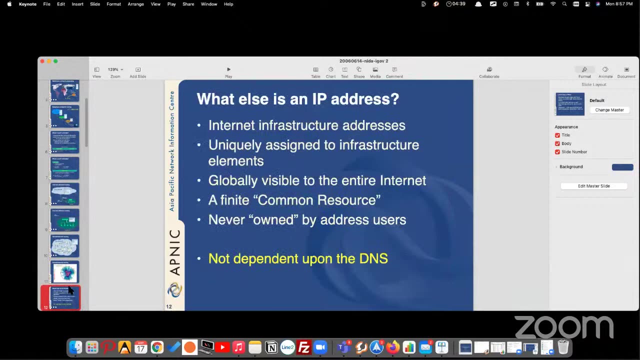 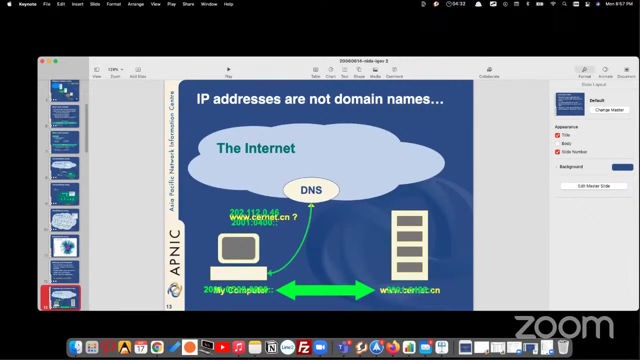 googlecom, facebookcom. so few sites are blocked because they have their own internal firewalls. so this is ip version 4 internet map. almost it is exhausted and it is a old ppt, so still, you can understand the boss of exhaust coach, okay, okay. so remember, ip addresses are not domain names, so domain name is your website name, like googlecom. 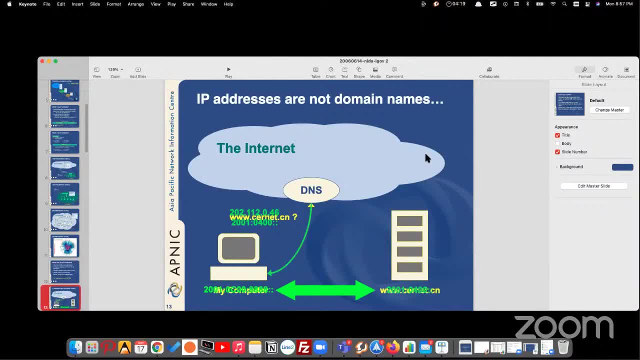 facebookcom, that is domain name and ip address is your. like 202, any number is called ip addresses, right, 101.. any four decimal number. if you have seen somewhere like 192, 168, and when you see 192, 168, um, yeah, you see any website like googlecom, facebookcom, that is domain name. okay, so that's all, so you can. 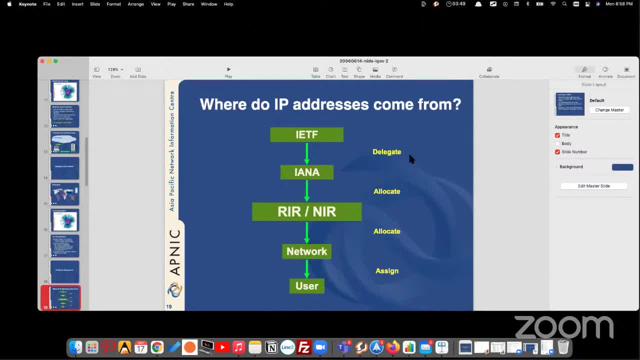 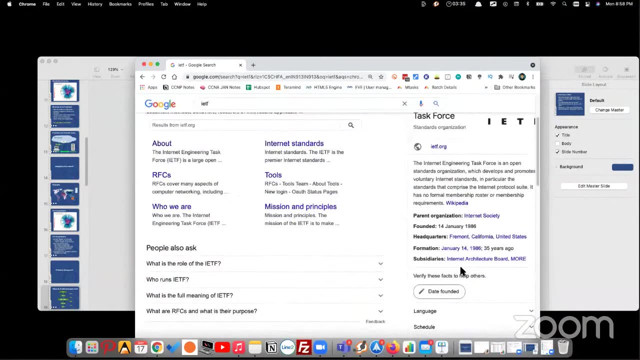 see where do ip addresses come from. ietf- internet engineering task force. what is ietf? you can just google it also and i'll show you also. ietf stand for internet engineering task force, which is founded in 1986. it is, like, mainly made for its open standard organization which develops and 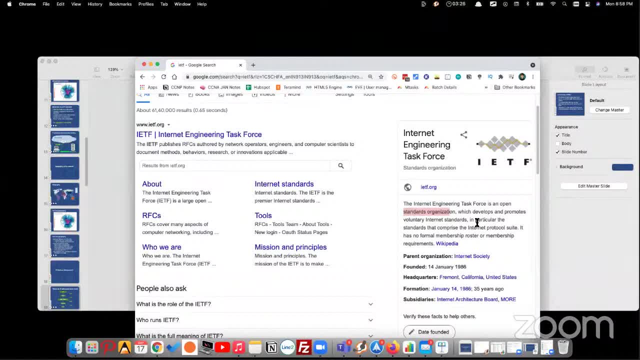 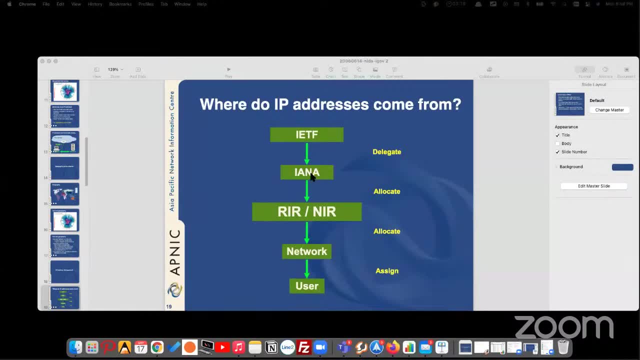 promote internet standard. so it is a big organization which promotes internet protocols. okay, so that is ietf. then they give to aina. so then, after that i have explained, aina gives to regional internet registry, then it gives to service providers or any company and then user. 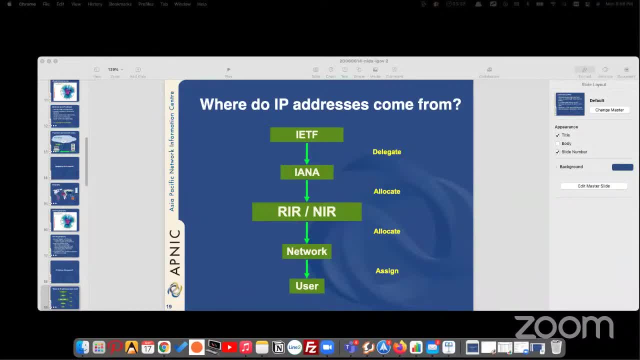 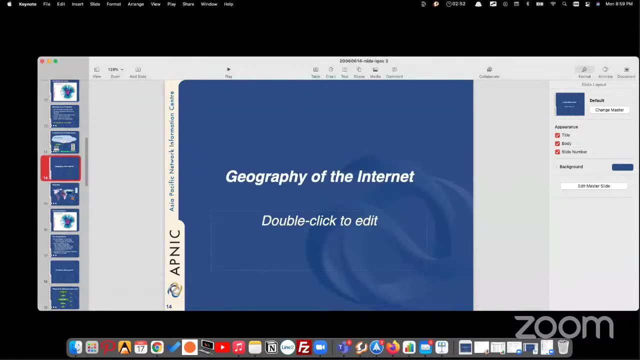 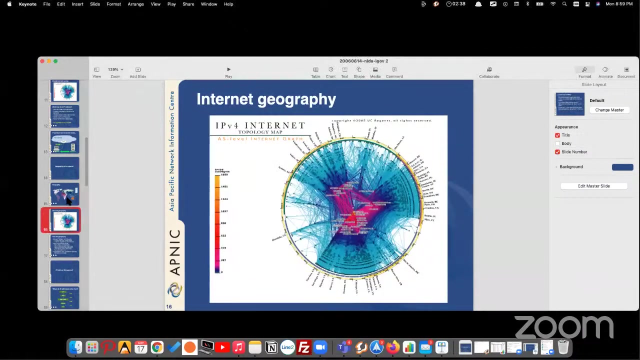 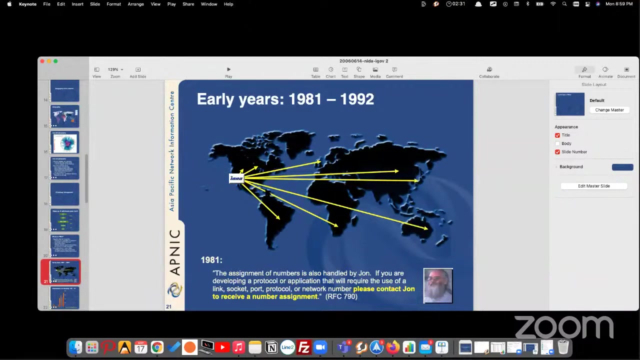 gets the ip address you, yes, everyone, any question? yes, all good, thank you. yes, i got it, okay, good, okay, let's move on. okay, so, when aina started, right, so just, it's like a funny story, only one guy used to manage the ip addresses. if in 1981, if you want to get any ip address, port number, protocol, then on the. 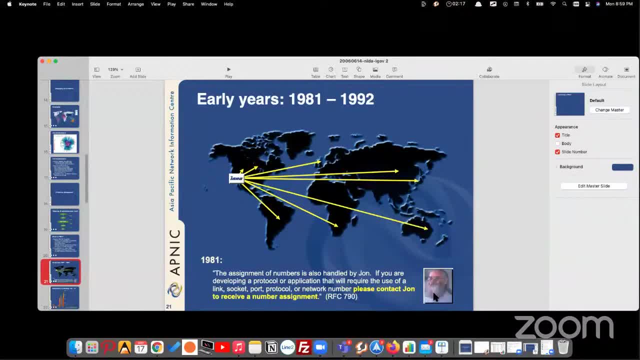 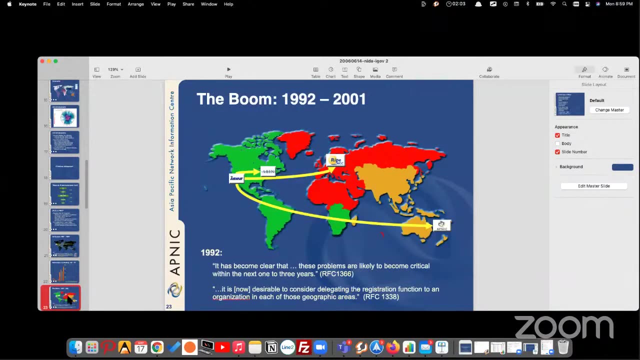 website. it's like: please contact john to receive a number assignment. so that is like long back, 30 years back, 30, 40 years back, almost okay. so only one person who used to manage the ip and protocol numbers. then, slowly, slowly, users are increased, routing tables are increased. this is why. 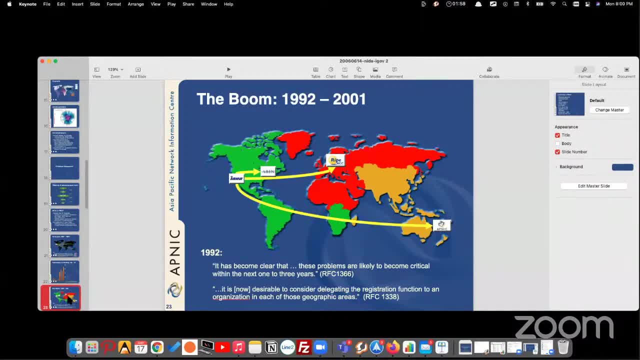 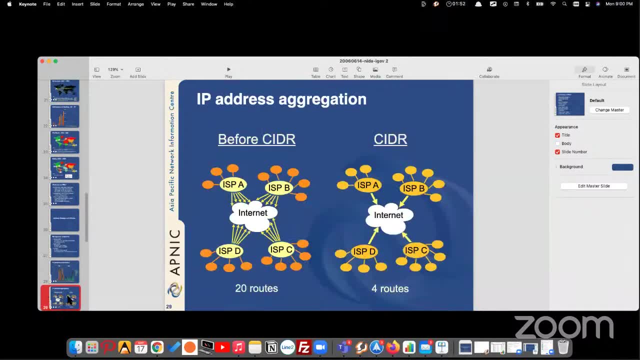 they have divided the network into different, different regional internet registries, and this is how this is what we call internet now. okay, so i now, so you have, like many service providers are getting a lot of routes. okay, this is also called cidr. i'll explain that. cidr is the name of 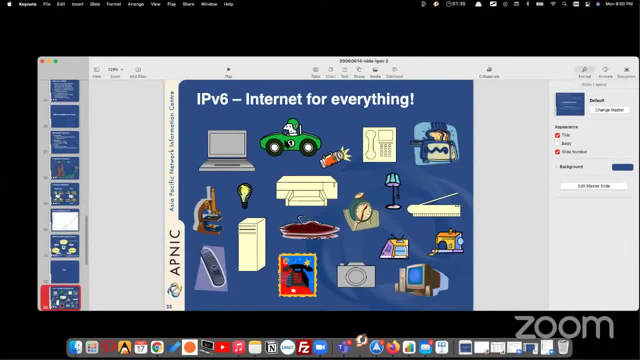 the one that cidr uses in this system. cidr so uh, so let's start. it's better. let's start the ip address now. so ipv6 is a very big number. you can assign ip address to. just hold on, guys, let me, yeah, yeah, so ipv6 is a very big number. like you can give ip addresses to any object in this world, so you will be able to use ipv6 every object in the world. 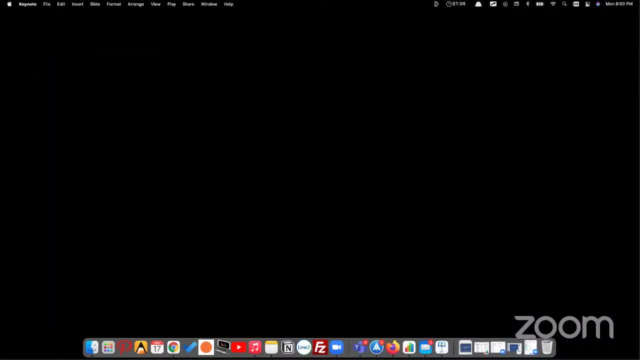 ipv6 is very big number. okay, thanks, okay, so this i was discussing aina, so now, now let's understand how aina divided the number, okay, so first of all, guys, please open your notebooks. please open your notebooks. decimal to binary: let's understand what is decimal to binary. 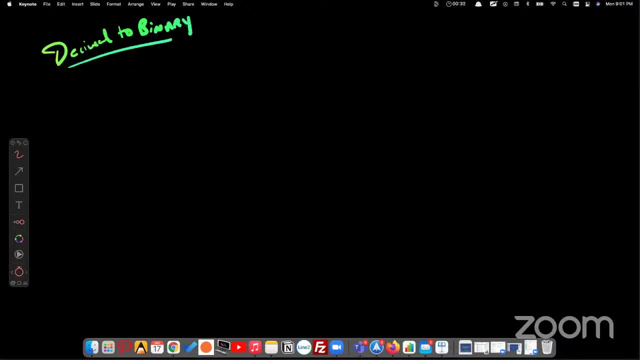 okay, just complete these three days workshop. you will be mastering submitting, i'm sure. so, decimal to binary, okay, so what is a decimal number and what is binary? so, whenever you get, when you, whenever you see ip address like this: so this is a decimal format, so this is a decimal. 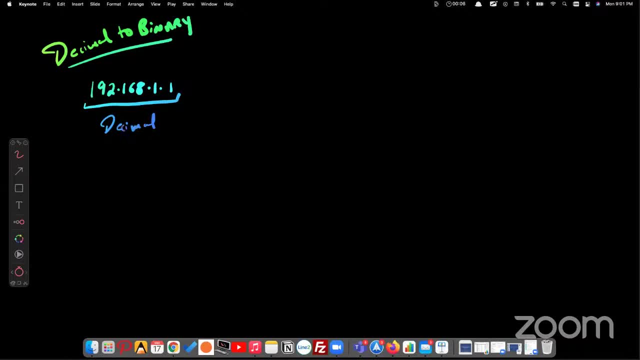 decimal format and when you see any number like 10110110, something like this, so this is called binary number, so this is called binary number. so tell me, your computer understand decimal or binary? so obviously binary, binary, right good. so now we have to understand first how computer 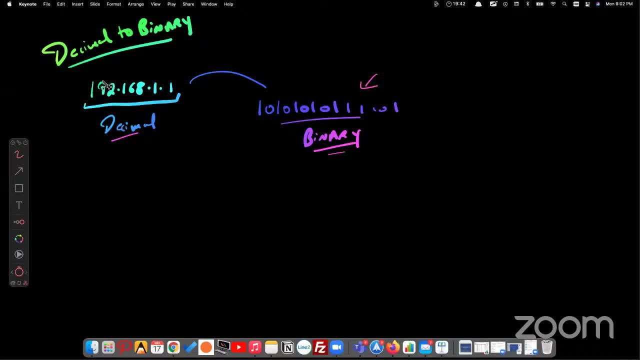 understand your ip address. ip address, so to understand this. so everyone knows that from school days also that so you have two digits, zero, and one in binary, yes or no. so 0 or 1 is binary, so this is also called machine language or something like that. so it's like binary. so now so 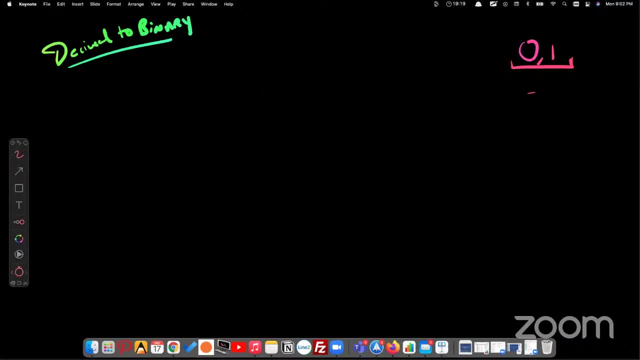 these are two numbers. so this is why in ip address we we always use power or base of two. we always use base of two, power of two, we always use base of 2.. ok, so we just 무슨 vampire? we can also f1 a kind ofrai from our Fernando te term. i don't know how to put here, but we can. you can type any other number, in case you do. you can type it. okay, i think i can type it. yes, and then, if anything, comment, please, please, email me. 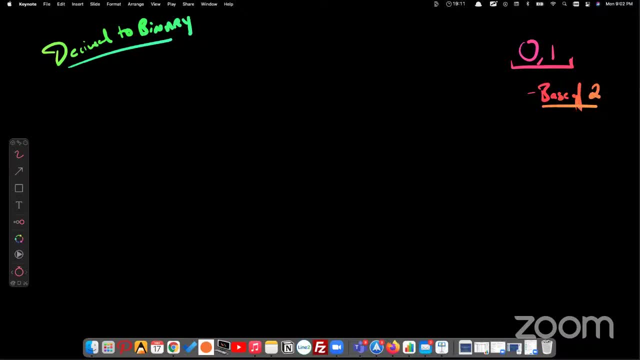 because these are two numbers, so this is why we always take two number. so now you can understand. so this is ip version 4. it is divided into four parts. so ip version 4 is how many bits? 32 bits. what is bits 0 and 1 is known as bits, so it means your ip version 4 is a combination of how many. 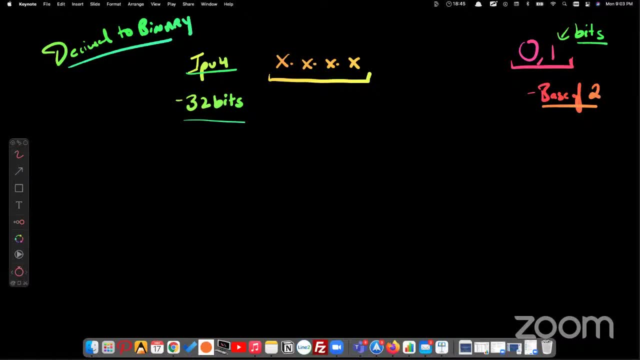 bits 32, 0 and 1s. okay, so now an ip address is divided into four parts. so ip version 4, 32 bit, 32 bit and it has four parts. okay, ip version 4 is 32 bits. it has four parts, which is called octet. 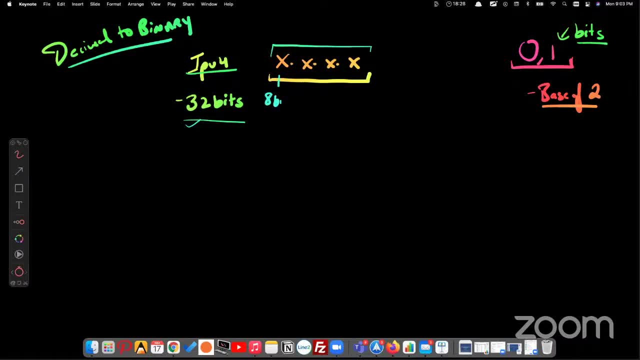 because every block is of 8 bit, 8 bit bits. you can say that 8 bits, 8 bits, 8 bits, and if you calculate 8 into 4 you get 32. okay, so now to understand decimal. to binary. okay. so first of all, you should know why we are learning, because we should know how to get the 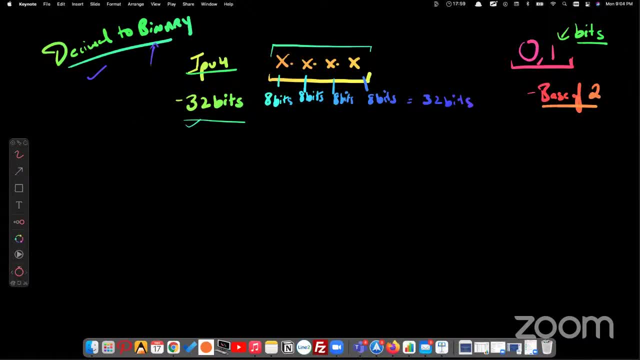 binary. okay, then we will be able to understand how aina divided the number. so 8 bits. so how we represent 8 bits. so we represent 8 bits with the power of 2, because your 0 and 1 is 2, so we always use power of 2s. so how to represent 8 bits. 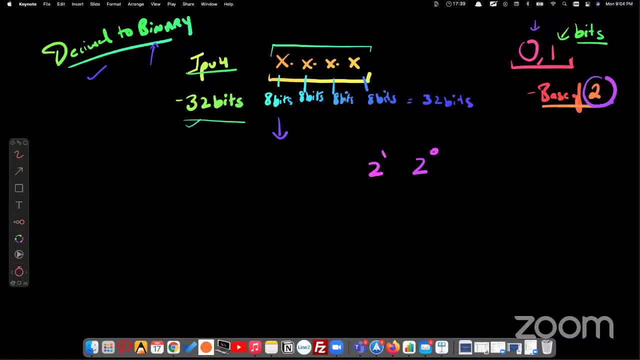 so, to the power of 0, to the power of 1, to the power of 2, to the power of 3, to the power of 4, 5, 6 and 7, we will not write to the power of 8, why? because we started with the. to the power of 0. 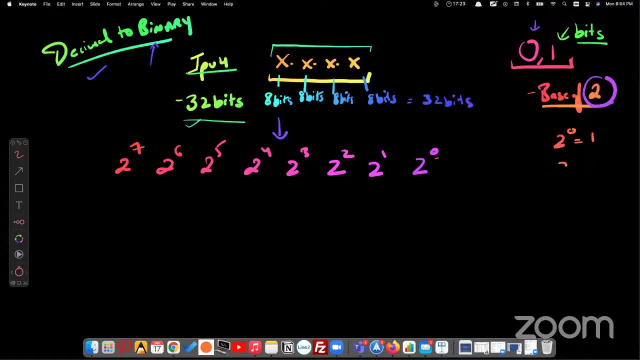 right. and if you check the table, to the power of 0 is 1, 2 to the power of 2, just double the, the value 8. to the power of 4 is 16, to the power of 5 is 32, to the power of 6 is 64 and to the: 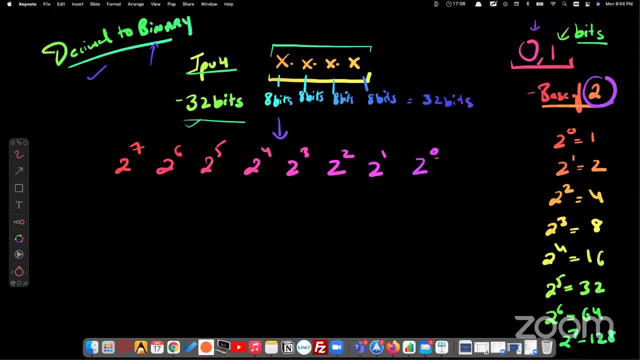 power of 7 is 128 and to the power of 8 is 255. okay, to the power of 8 is 255, so you can write these values here like it's 128. you can write on top also: 128, 64, 32, 8, 4, sorry, 16. 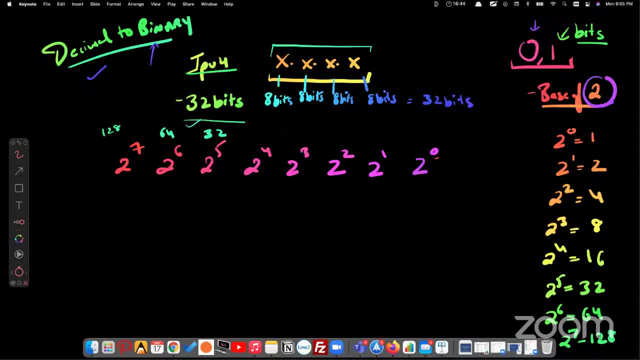 16, 8, 4, 2, 1. okay. so please remember, to the power of any number, power of 0 is called 1. okay, so now how to calculate the number. suppose you want to get the binary number of 192. so how to get the binary of 192? so 192. 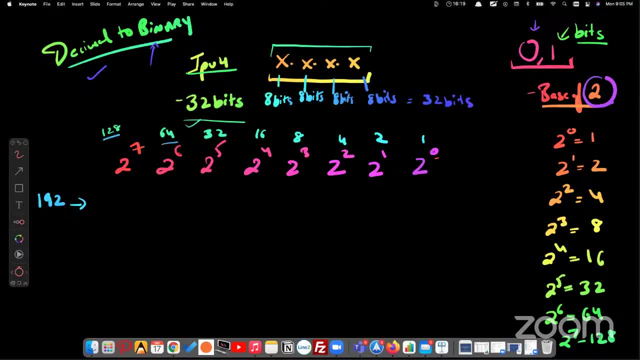 so you can just count: 128 plus 64 is 192. so you just have to on the bit which is called 1. so you have to on the bit on means 1 and rest values will be 0 and this will be binary means. your computer understand 192 in this format. okay, in this format. 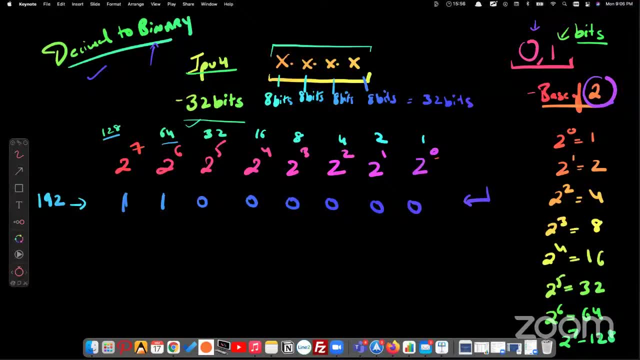 so you can just count: 128 plus 64 is 192, so you just have to on the bit which is called 1, and after that, if i calculate for, suppose, uh, 192, after that let's calculate for 168. so 168 would be 128 plus 32. 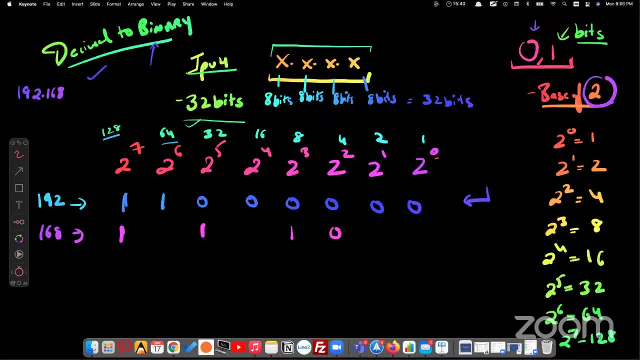 is 160, 160 plus 8, 168 and rest value 0. okay, so guys tell me what will be the value for 10 and then after that, uh, please write in the chat what will be the binary value of 10 and after that give me binary value of 7.. suppose this is ip address. so the binary value for 192 is: 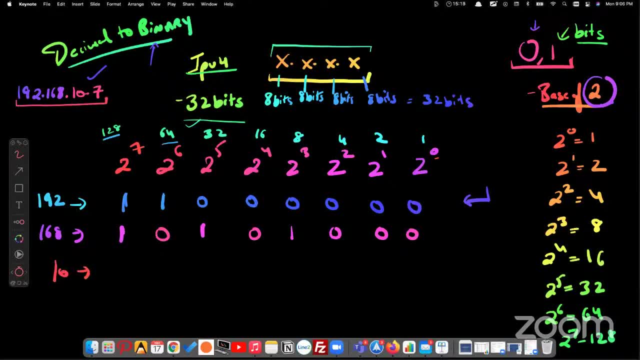 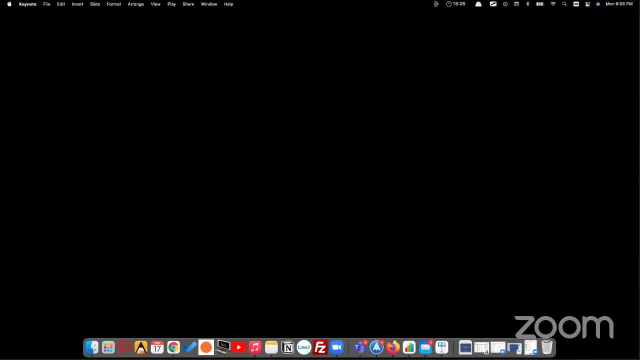 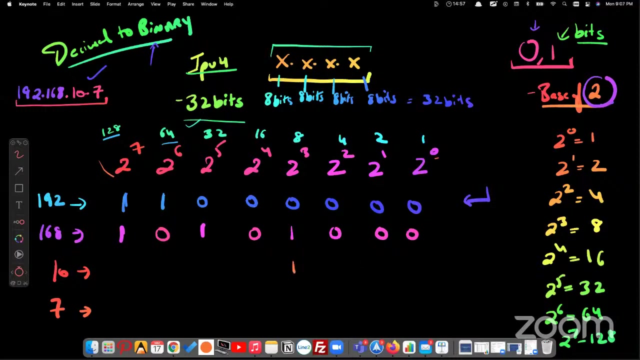 this 168. this tell me the binary value for 10 and then for 7.. just do it, you have two minutes, okay? yes, So we are going to plus 8, plus 2, 8, just see the number here: 8,, 2,, 8 and 2 is 10 and rest value is 0. 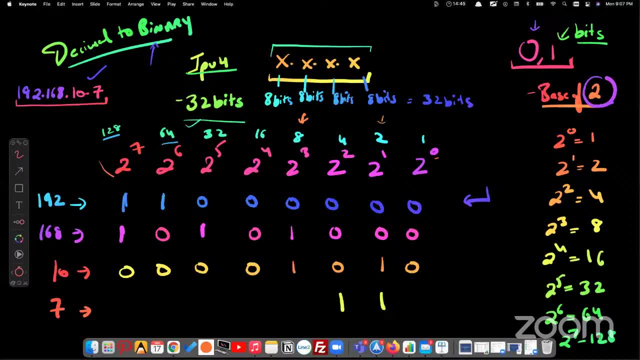 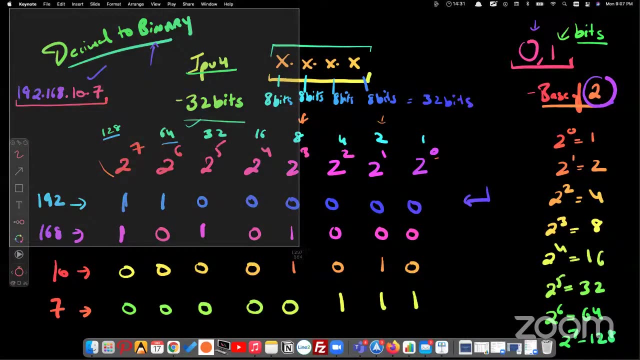 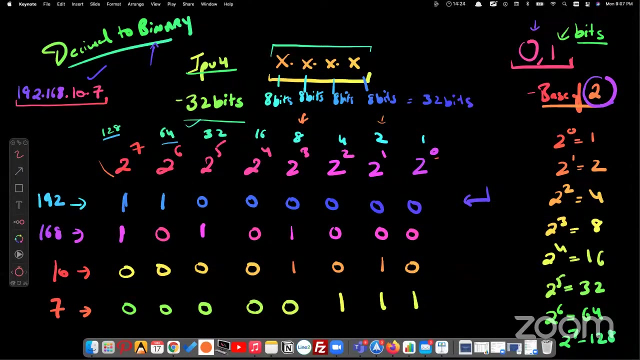 Very simple. What about 7?? 4 plus 2 plus 1 is 7, rest value is 0.. Clear, Yes sir. Okay, good, Okay. so this is a decimal to binary. Now the good story. let's understand how Aina divided this number. 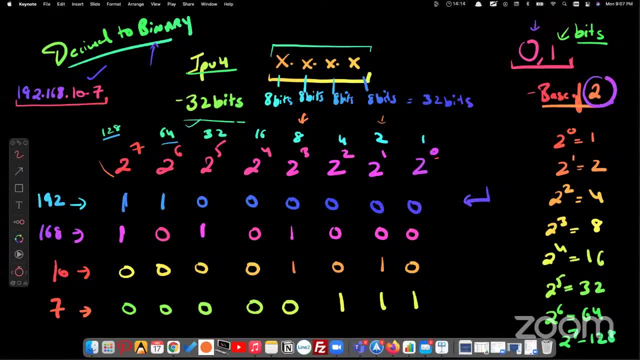 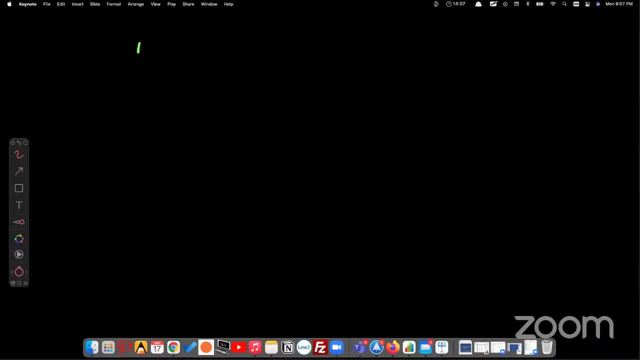 Okay, In every live session we just write: hi, sir. Okay, So how Aina divided the number So you can just write down the gain values. 2 to the power of 7 is, So you can write down the number again. 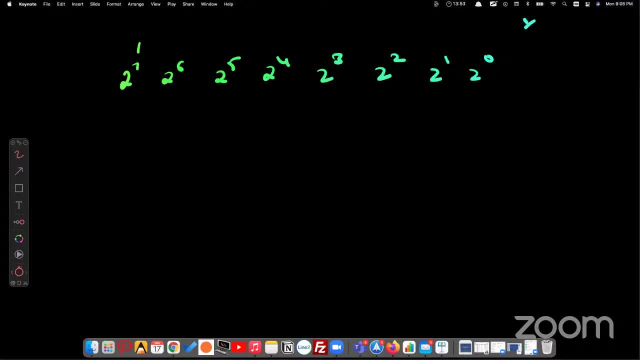 So just take into consideration one subnet, one octet. So you have 4 octet. So each every octet is like this, not just one octet. So in all four this is what happens. All four octets are like this: 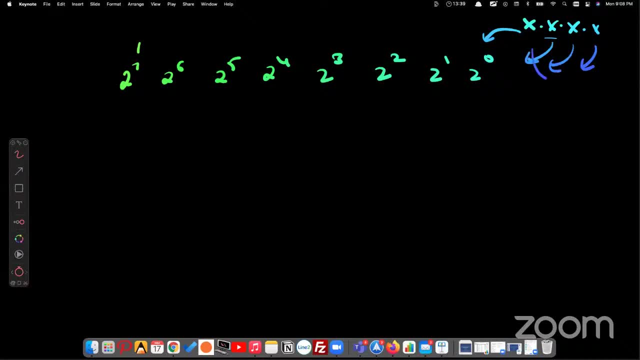 This is the calculation. Okay, So all four octets have similar calculation. So now you can see 2 to the power of 7, how Aina divided the number system, which is called IP address range. So I have delivered it in some batches first, 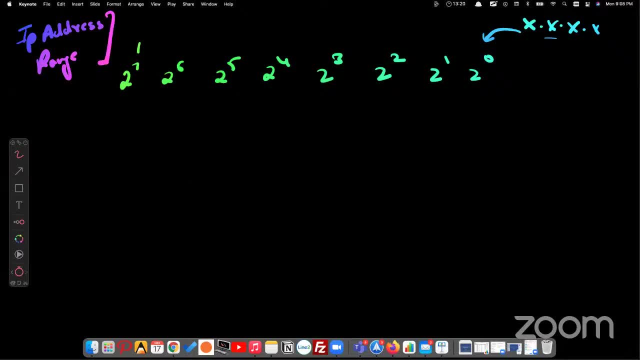 So IP address range. how Aina divided the IP address range? So 2 to the power of 7 is obviously 128.. You can write down 64,, 32,, 16,, 8,, 4,, 2, 1, right. 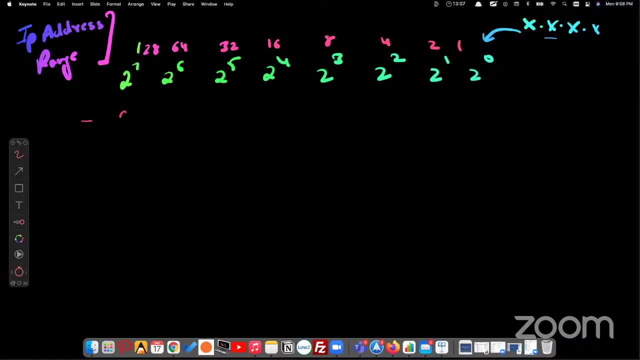 So this is the value. So in the first octet, in the first part, you take all 0. And tell me what will be the value? Obviously 0. In the second time you have to take 1 here. 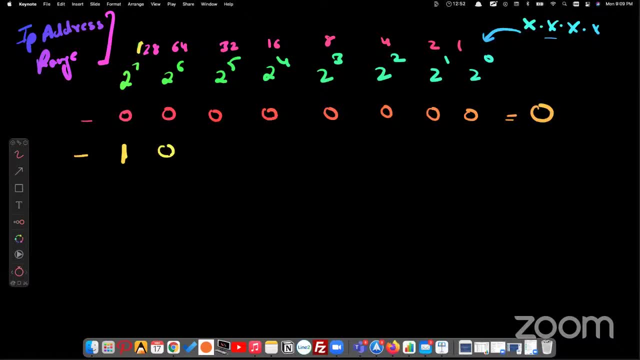 And on 1, you can see there is 128.. So rest value is 0.. So see what is 1 above. So you can see there is 128 if you take this 1 only. So the binary of this value, the decimal value for this, is 128. 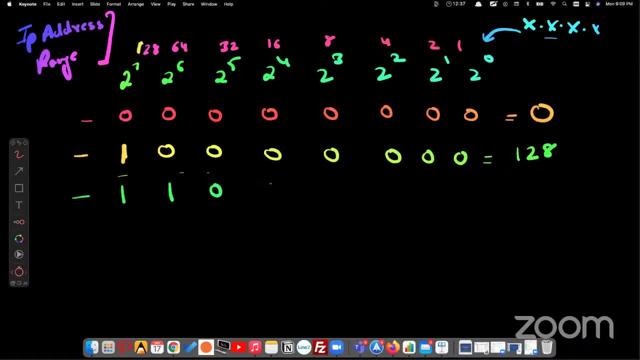 And if you take 2 1s, what will be the value? Just plus 128, plus 64.. 192.. Okay, Just plus 3. 192.. You will be getting 224.. 224. Okay, And then you take 4.. 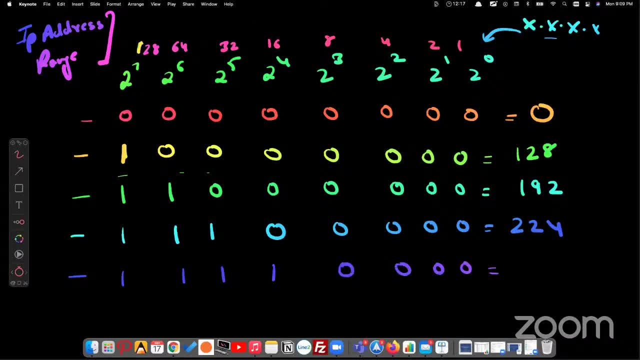 And then Aina thought it's enough. I think we should not go, because the maximum we can go up to 250.. 25. And before 240, we get 239.. Right Before 224, we get 223.. 192,, 191.. 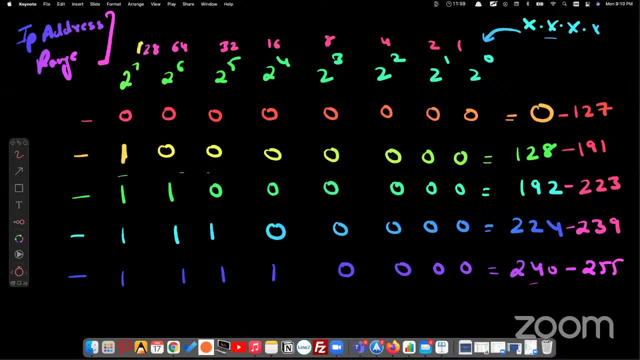 And before 128, we got 127.. So this is A-class, B-class, C-class, D-class, E-class. Tell me who was beating the drum. Great, great sir, Great Okay, Got it now. 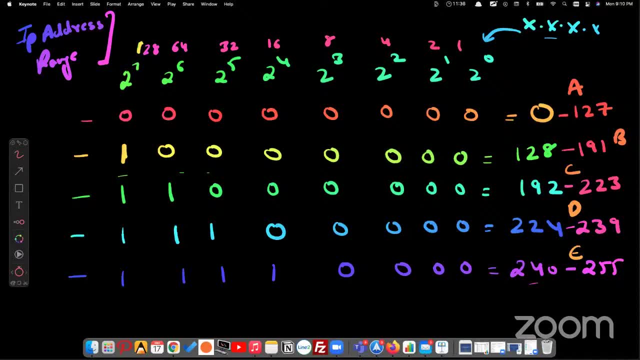 So this is how Aina divided the classes And this is how actually we got the ranges. So this is cool. Let me show you how we did it. Okay, Cool, Got it. Yes sir, Yes sir. 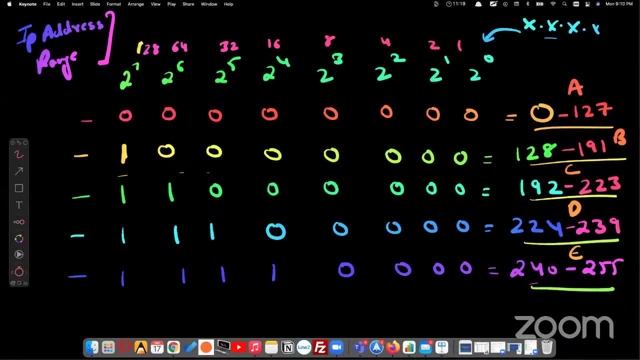 Any doubt? No, sir, No, Okay, good, So let's go further. Now you know how IP addresses evolved. Okay, Tell me quiz time, Like: what is the first step to get the IP address? Who starts the IP address? 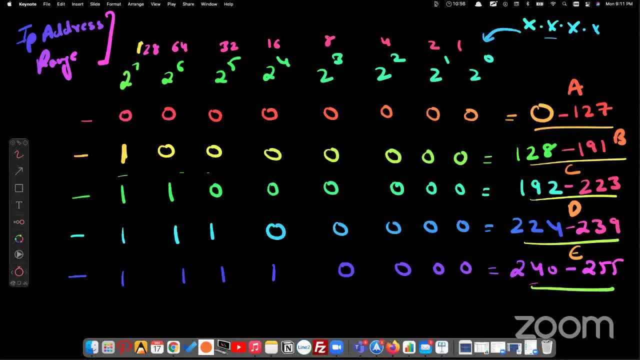 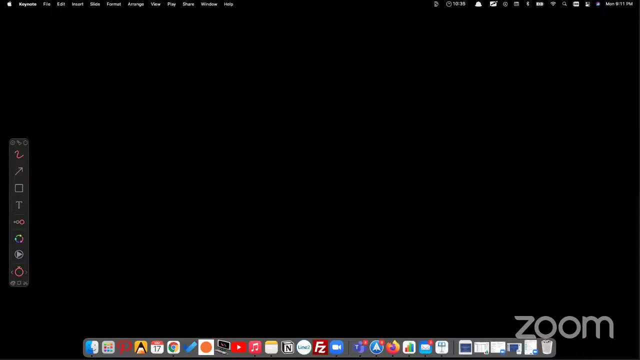 what's the IP address, IETF, Internet Engineering Task Force, then INA, then RIR, right. Then you get in companies or any network, then user gets right. So I'll share that PPT with you, Don't worry, You can just check on that, Okay. So now let's go to another thing. Now. 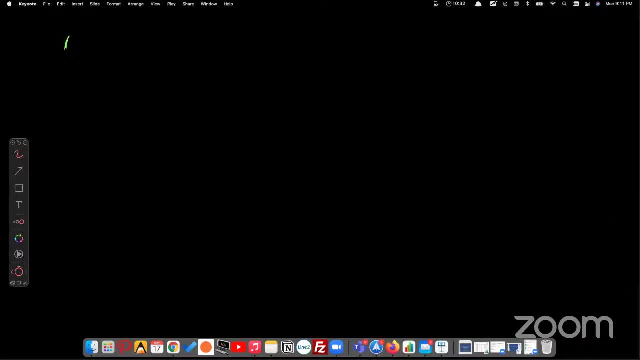 if we talk about A class, B class, C class, okay, this is mostly we use. We don't use D and E class because your computer does not support D and E. D class is used for multicasting like routers using some like. if you have done CCNA or not, I don't know, But if a router 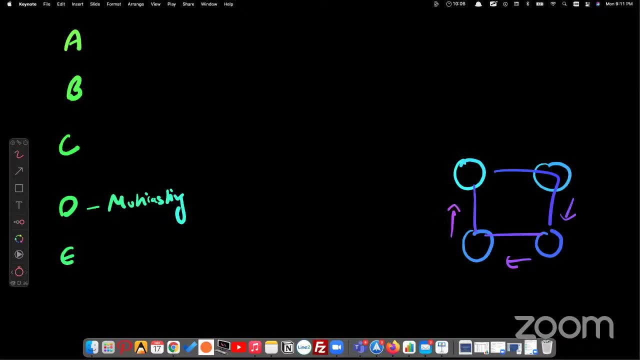 wants to share their information with each other. mostly routers uses multicasting. Like there is a protocol called RIP. It uses 22400009, something Okay. EIGRP uses 2240010.. So what is this? This is the IP address of some protocols which are which you learn. 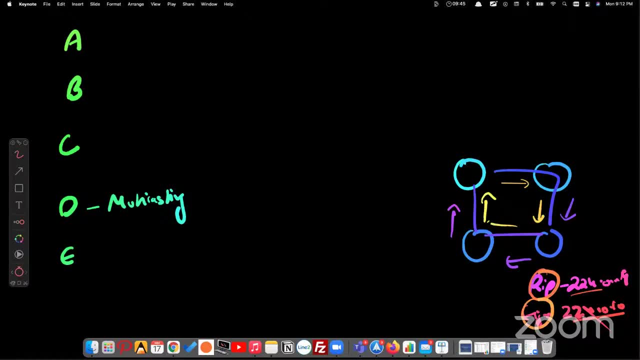 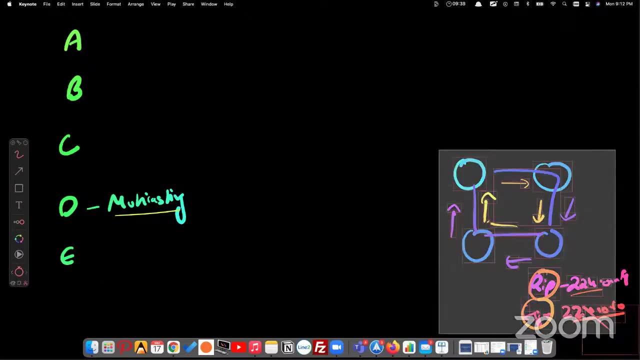 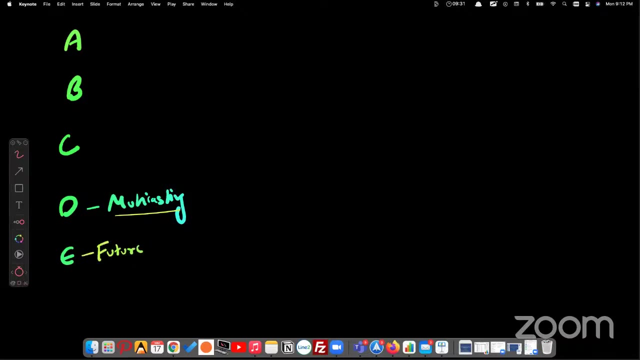 in CCNA or CCNP so that routers can share information with each other. So this is called multicasting. So your computer don't understand this language, So this is called a multicasting. and E D is used for some in most of the books. you will see future use, but from last 20 years. 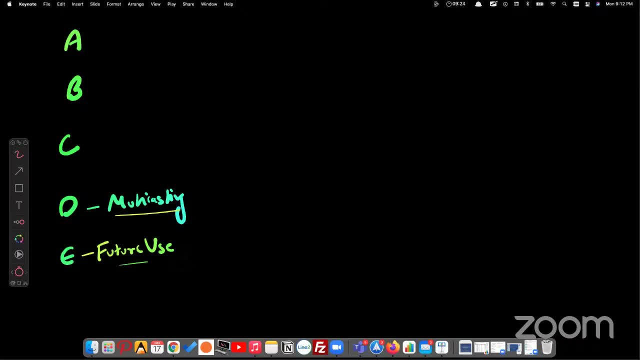 all books are saying future, So what future they are talking about? Actually, there is no future use. It is actually wasted. Why? Because not even a single computer or operating system like Windows machines. If you try to give any IP address above 223, Windows is going to give you a warning that. 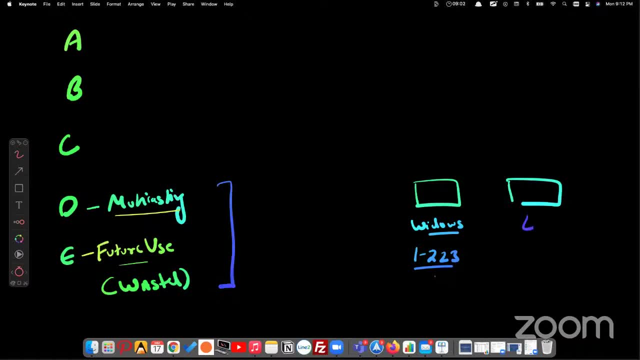 you can't use D And E in Windows, Also in Linux Also. you can't use a D and E. You can't use in Android phones, You can't use in iPhones, mostly like all hundred percent devices, Like you can't. 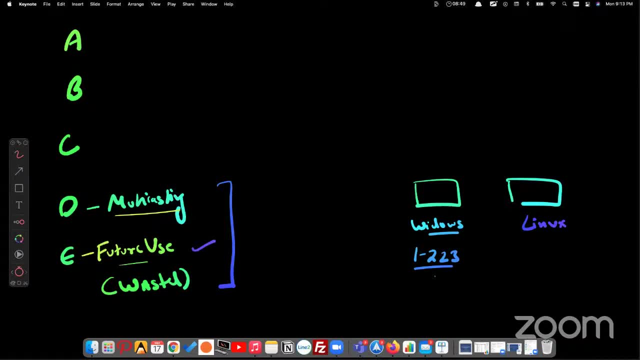 use D and E. Now tell me, even if we have an E class, how we are going to implement, because not even the old machines, not even the new machines, can't understand E class. Hello, Yes, guys, yes sir, Got it. Yes sir, Okay Wasted. No operating system is supporting. 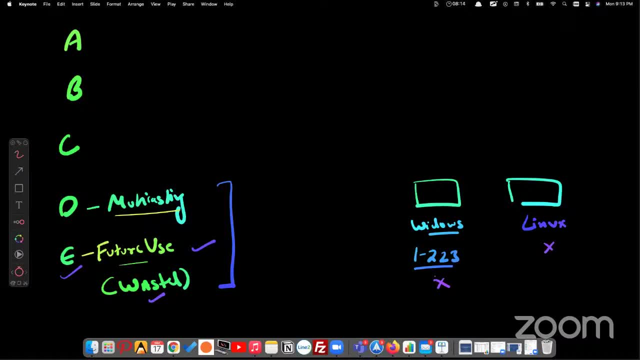 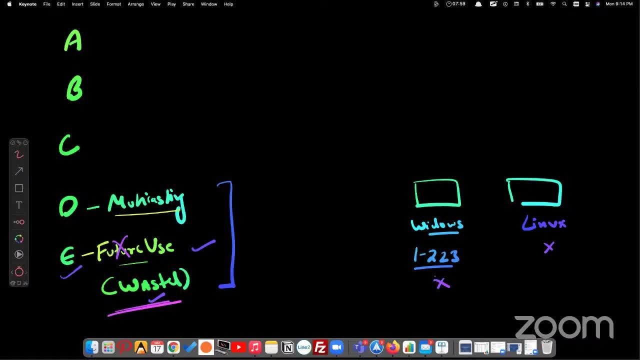 Okay, So this is why we can't use E class And D obviously is reserved for routing and all. So we can only use A, B and C. Okay, So let's understand ABC, Why we have ABC. So in all IP address, in IP address version four, even in version six, you have two components, or two components. 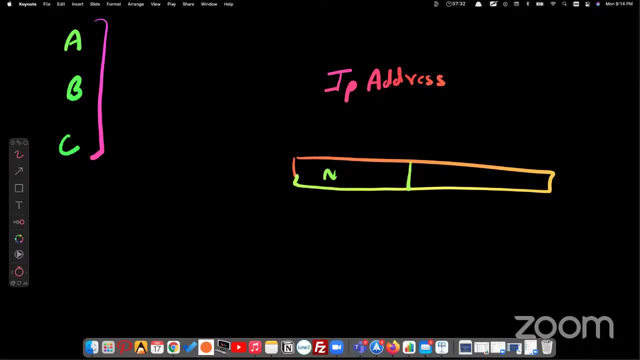 two parts. every ip address divided into two parts. one is called the network and one is called host. so if two machines wants to speak with or want to communicate with each other, your network portion should match. then only they will able to share the information if your network is not matching. 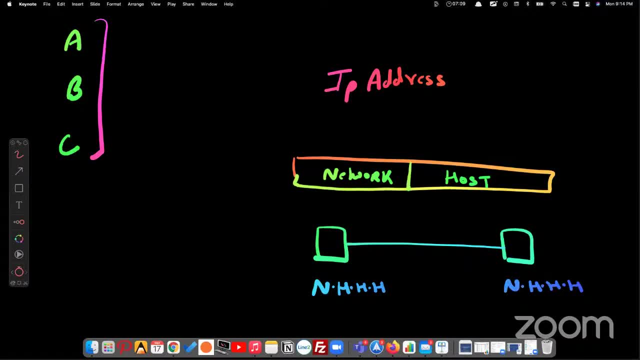 it means the computer want able to communicate. so for example, like your class a has one octet network and rest part is host. so what does it mean? so if you use a class a which is like the range is like 1 to 126, 0 and 127 is reserved. so if we give ip address like 1.1.1.1. 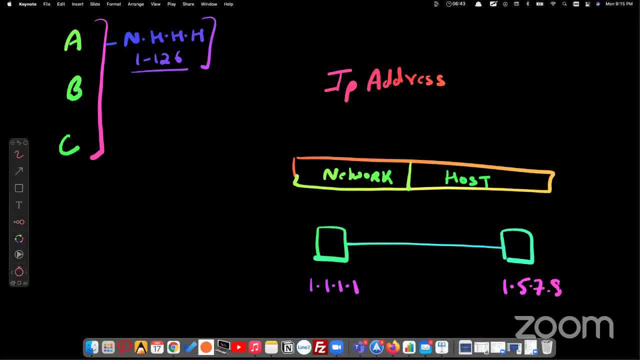 and if you give ip 1.5.7.8, so tell me if they will be able to communicate with each other. yes, sir, yes, because class a only checks the first portion. this is network and you can see both. the network is matching, yes or no? the 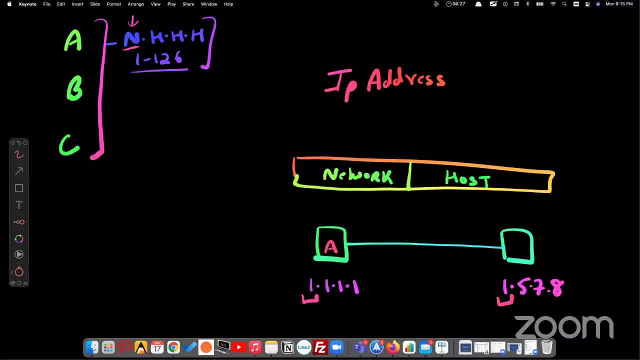 same digit. both the end, yes, sir, yes or no, yes side, same digit. so it means it is in the same network. but now you understand, right, because you are human, you can understand my language. you are able to understand my hindi, english, whatever i am saying, right? but how computer. 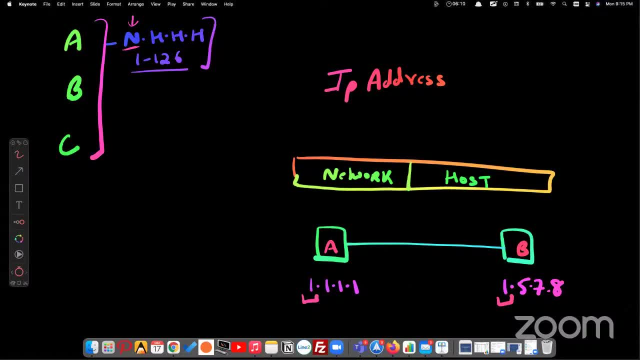 will able to understand that this is my network. so we call, we use a subnet mask, so there is a number called subnet mask so that we can inform our computer that what is your network part? okay, so if you write two, five, five, dot zero, dot, zero, dot zero. two, five, five, dot, zero, dot zero. 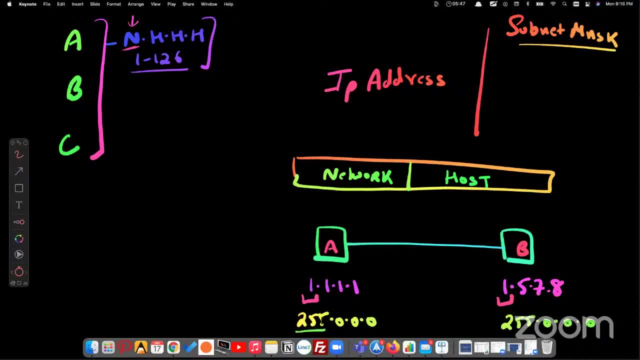 so what does it mean? so it means just two, five. five means, uh like, first eight bits, is it you have to match. so first octet 255 means you have to match the first octet. you have to match the first octet. this is how you give ip address to a computer. okay. 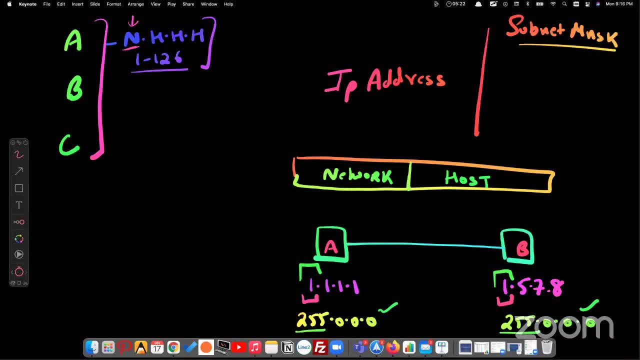 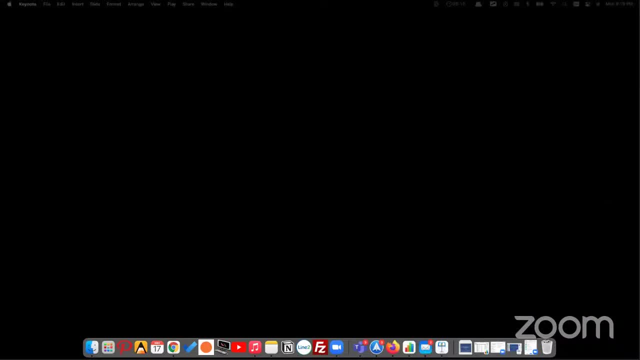 so let's understand how to give ip address to a computer. let me share. just hold on. it's very simple. i'm sure most of you are advanced learners, but still i don't want to hi. okay, so just hold on. okay, so i just started a windows machine here, so it's very basic how to assign ip. 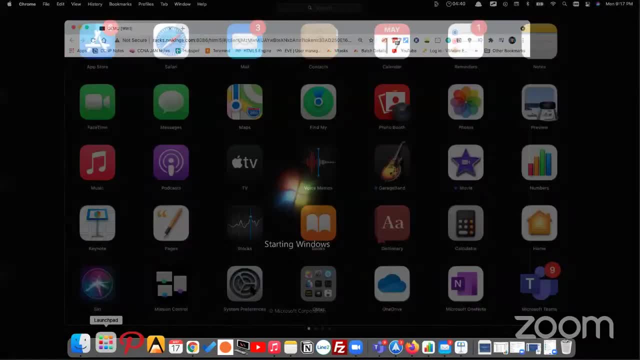 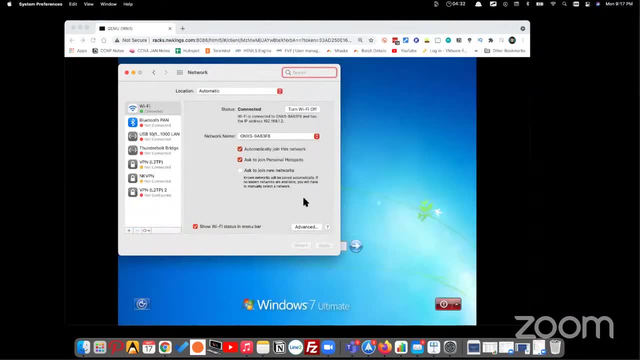 to a computer. okay, so in macbook also you can assign in, go to system and there is a network and you can see on the advanced part and it go to tcp ip and here you can give the ip address. you can use the manually ip and you can assign all your ip, whatever ip you have. so you can see. 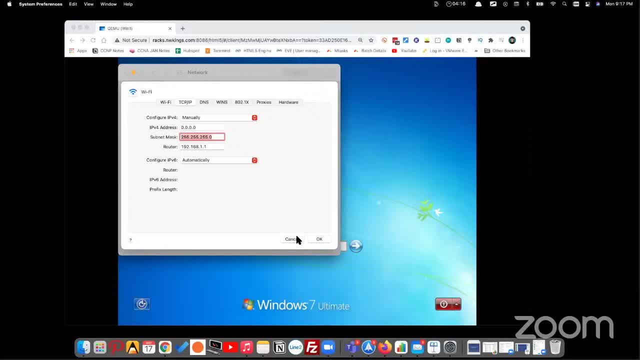 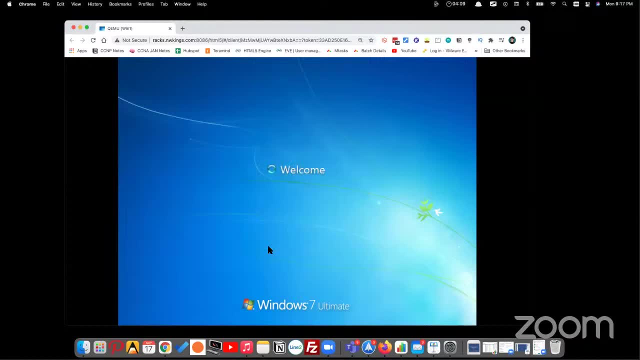 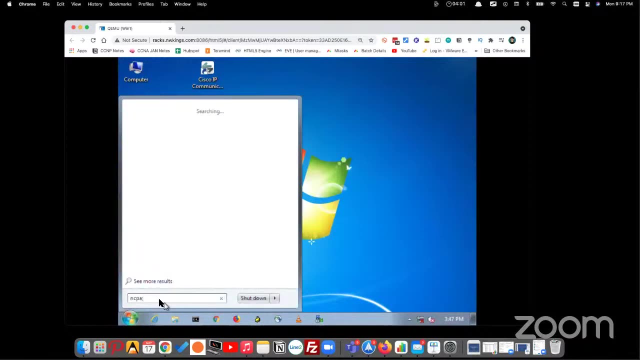 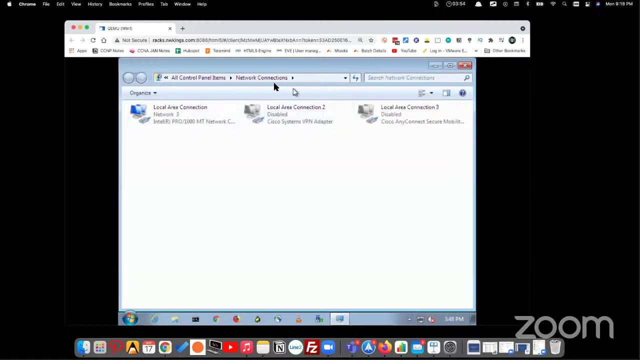 there is a subnet mask here, so this actually tells what is your network part, network part. so let's just see the windows, because most of you are using windows. so there is a shortcut: directly go to ncpacpl. okay, so you can go to ncpacpl, or you can go to control plane. control plane, sorry, control panel. 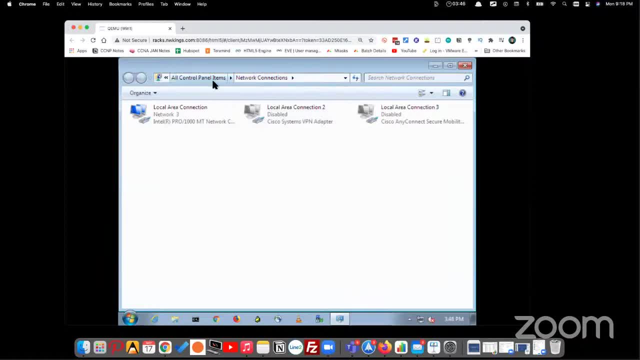 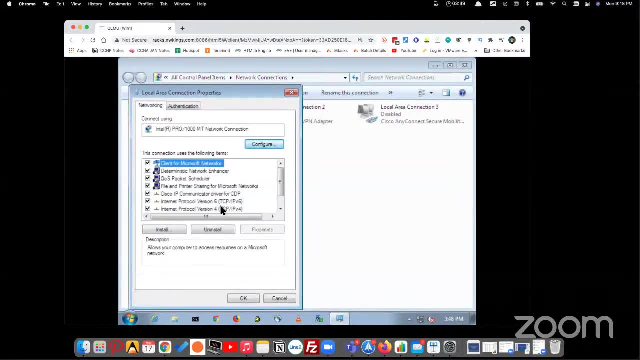 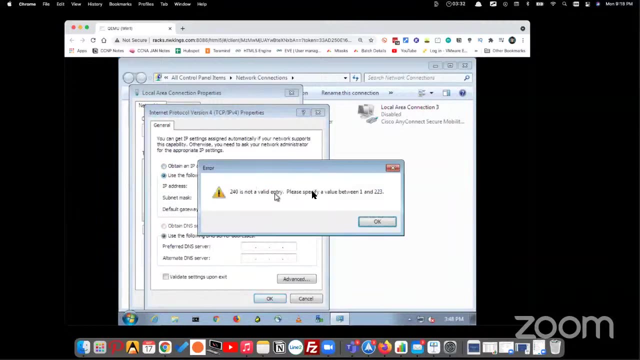 so control plane is like we have in routers, so control panel network connection. so this is the my ethernet adapter properties. click on ip version 4, go to properties and you can see. so whenever you give, try to give any ip like 240 so you can see the system is giving you a warning. 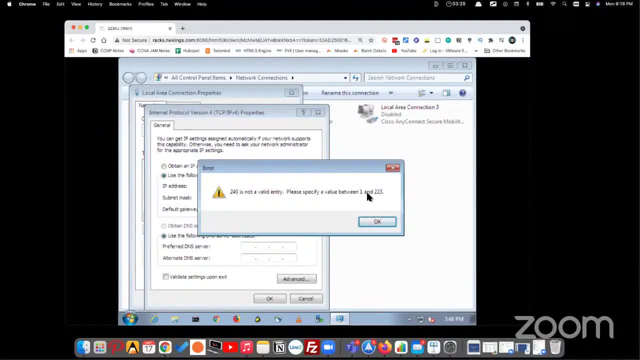 that you can only assign ip from 1 to 2 to 3.. it means you can only use a, b and c. okay, suppose, if i am going to give 1.1.1.1 and if you click here, automatically system is taking. 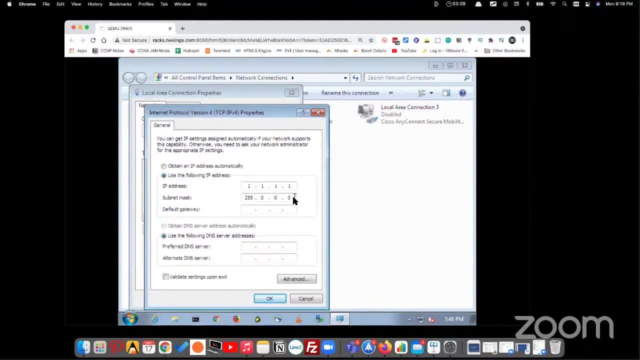 5.0.0.0. so this is called by default a subnet mask. so somewhere might be- you have seen 255 here also- or maybe like this: even this is class a might be you guys have seen some different subnet mask, or maybe like 128.. so what is this? this is what we call subnetting, which we are going to learn. 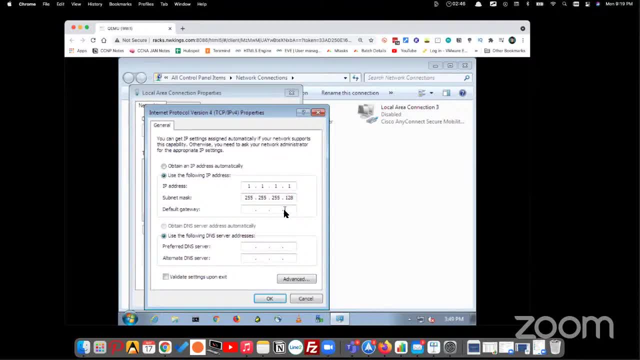 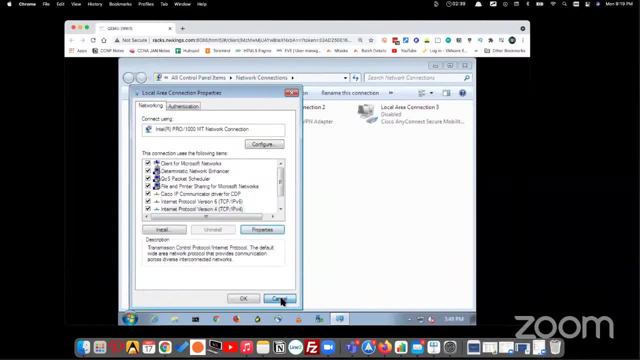 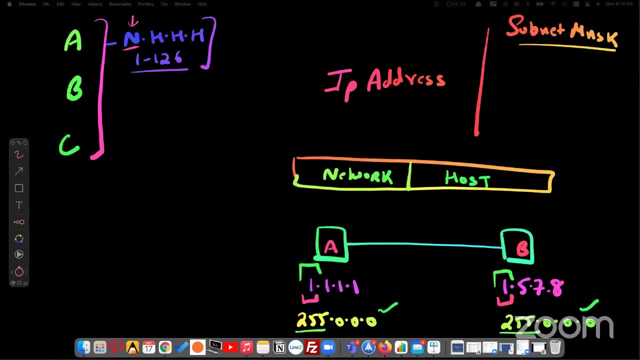 and this is why we have conducted this workshop. okay, So what do we need to know now? what is this subnet mask? i'll explain that subnet mask, but you can also understand this. first of all, we need to understand, like: what is the difference between a, b and c? 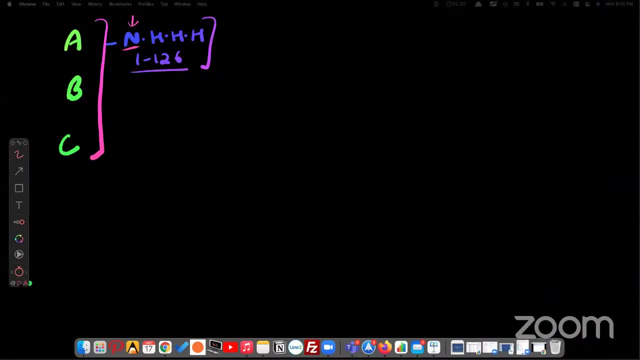 okay so let's take one example of class a. okay so, if you have two computers or two servers or some any device? okay so let's take example of class a, if you are also a manager and you have two cyberten at a one where you can have ip. i have already given example. 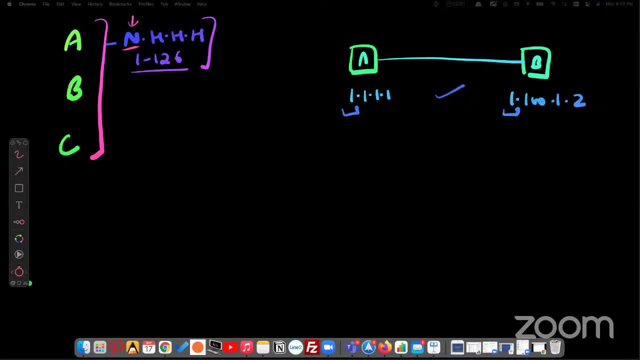 1.1.1.1 and you you have 1.100.1.. any ip but a computer only checks the first part and it means they will be able to communicate with each other. if they use class a with this subnet mask, right, okay, tell me the same ik address, but if i'm going to use 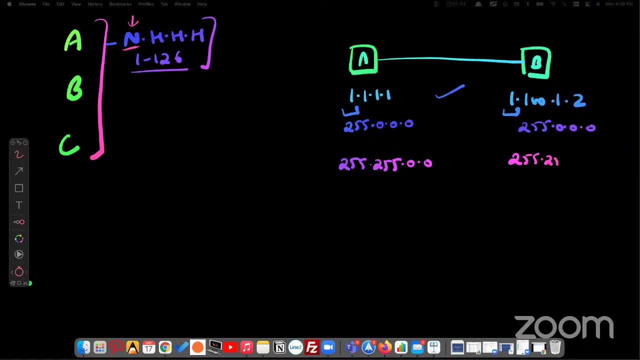 it means you have to match two subnets, so will they able to communicate? in this case, check karo, kya do part match ho rahe hai. so two parts are matching. no, sir, it means they will not able to communicate. if we will be putting this subnet mask, so this is called. so this by default. 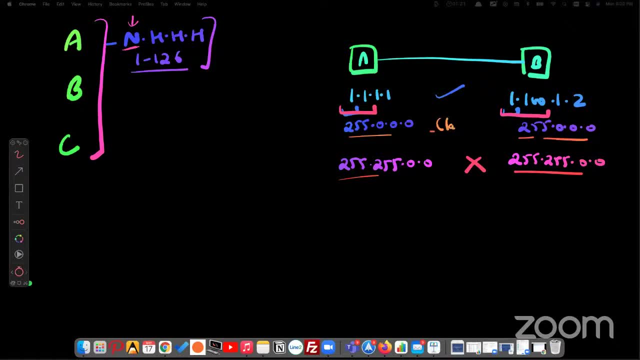 this is called by default. so in networking we call this class full. this is called class full because this is by default. okay, and whenever you change the subnet mask, because this is class. a by default is 25500, but if you use some different one which is not default, this is called classless. 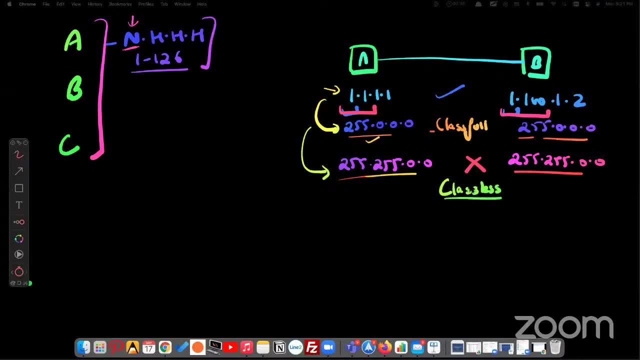 what is this class classless? yeah, got it. yes, sir, yes sir, clear everyone. any question? no, sir, okay, so let's talk about b class. now. if you have two another computers, but here we are going to assign one b class ip, where we have two network part and two host part. remember, we have two. 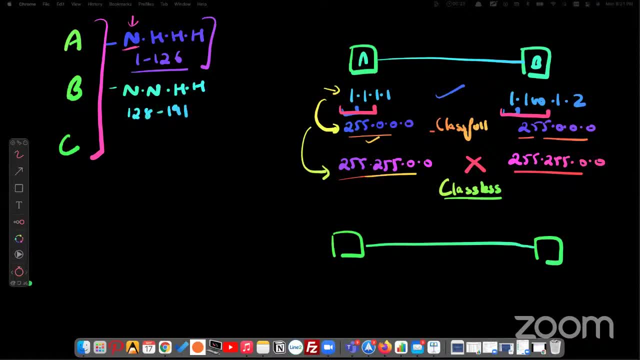 network part. so range is 128 to 191. so any ip address start from this range. suppose you have 150 ip and you have 150.1.2.3. so tell me with by default a subnet mask. by default subnet mask is 255.0, because you have one network part, so you have two network parts. so 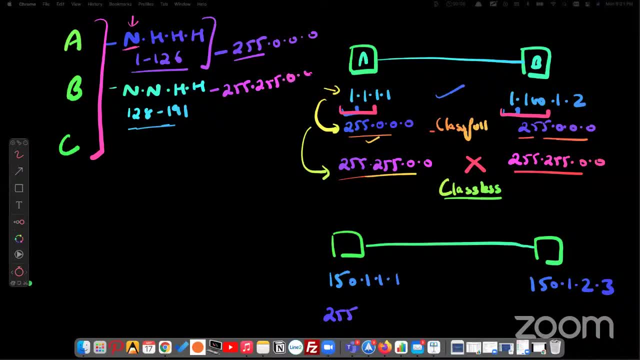 by default subnet mask will be two times 255 and c will be 3n and one h, sorry, okay. so the 3n means three, two, five, five. so this is by default subnet mask. okay, so, remember guys, a class ip, a class ip address. by default is this, but when you go in your production networks, or maybe you go for 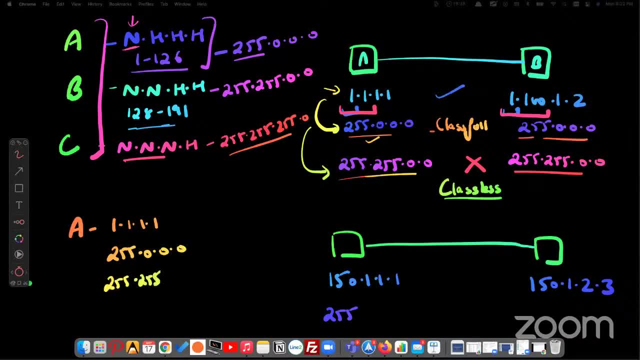 any company maybe have this subnet mask, okay, so this is not wrong, this is also correct. but they have divided their network into some different parts, so this is not b class. so i have seen people ask me, or student ask me, this question: sir, this is class a, why you have given this b class? 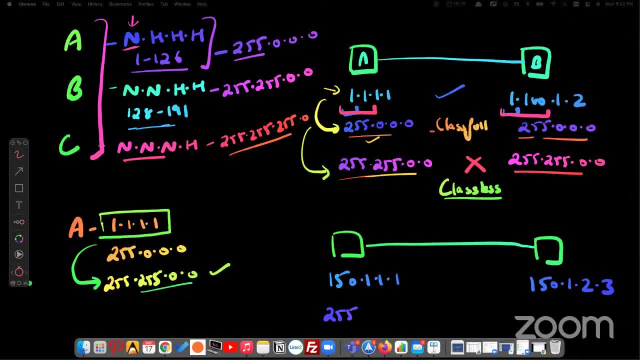 subnet mask. so remember, guys, this is not b b register. okay, so this is not b class. so this is default of b but this does not belong to b. all classes we check with the first ip address. we check all classes with the number, with, not subnet mask. okay, don't do this mistake. we always check. 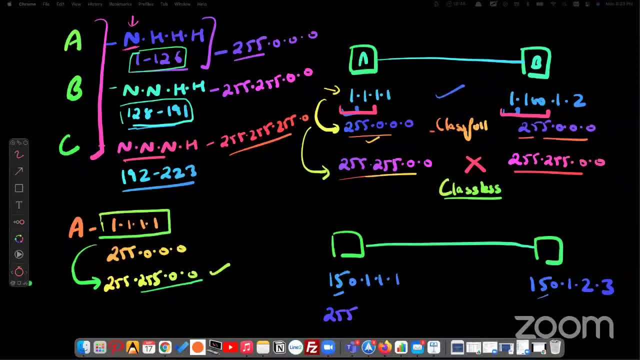 the number to check. this is class b, this is class b. but whenever you see subnet mask, it can be of class a, it can be of this can be of anyone. okay, when we will study subnetting, even you might have three times 255. and remember, this is not class c, this is class c default. but when you give this ip address to 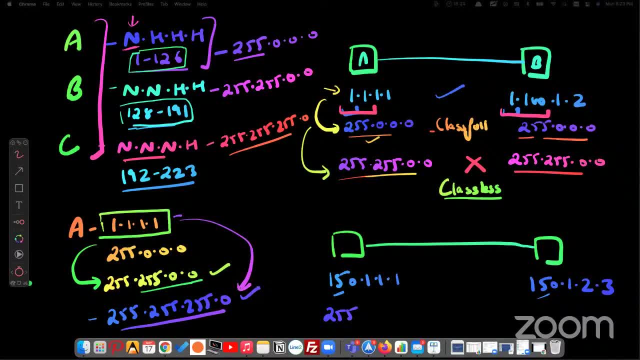 class a, ip, so it does not make this ip address class c. it is still class a. if it is not on your or for, say, goblet, i'm all the students, our students know we are going to our débate on it. they are very radicalish, excuse me. 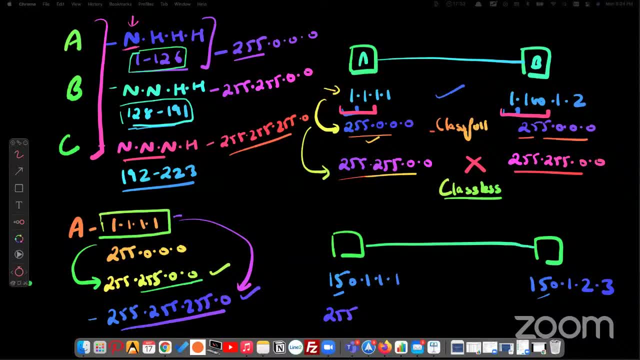 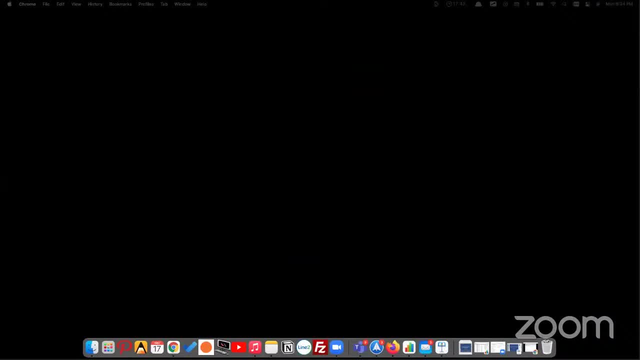 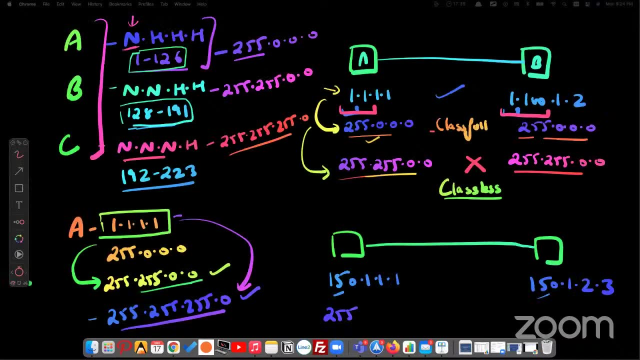 yes, sir, will anyone repeat from me? or what have i said? how did i say yes, anyone? yeah, anyone, why? how you are going to face interviews, man? yes, yeah, tell me, yeah, tell me what I explained. there is a class. there are three types of IP address we are using. 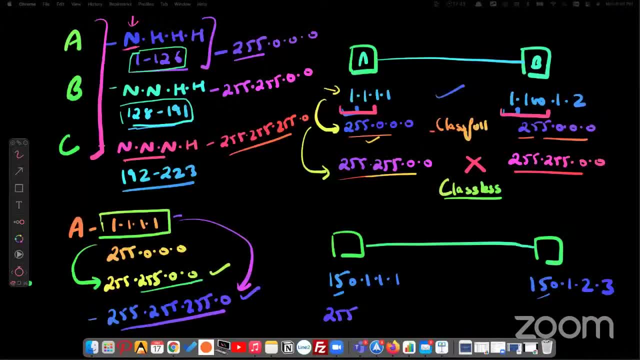 so there is A, B and C. so IP address will be the define on the network, what we check from network portion. they are able to communicate or not? yes, ok, now if I put 255, 255.0, zero, this is by default. so definitely they are. 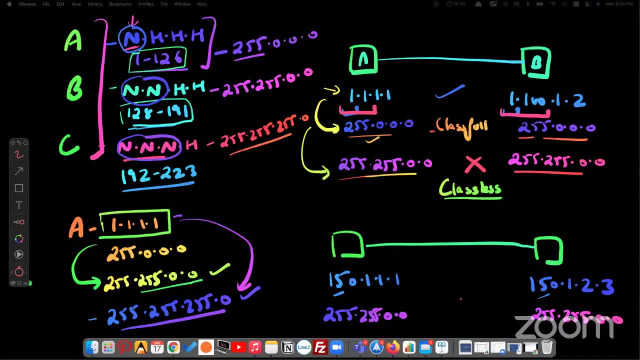 going to be able to convey or not? they are going to complete that or cannot communicate? are going to communicate with each other, yes or no? right, because you have two, two, five, five, two, two, five five and both 150.1. same in both the cases, right? so it means they will communicate. 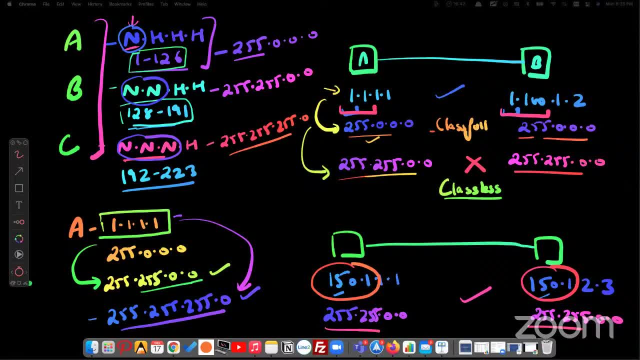 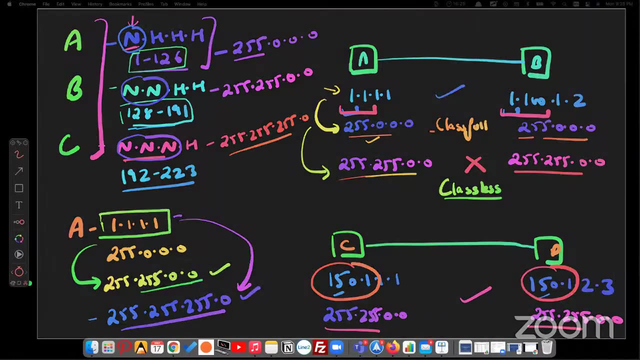 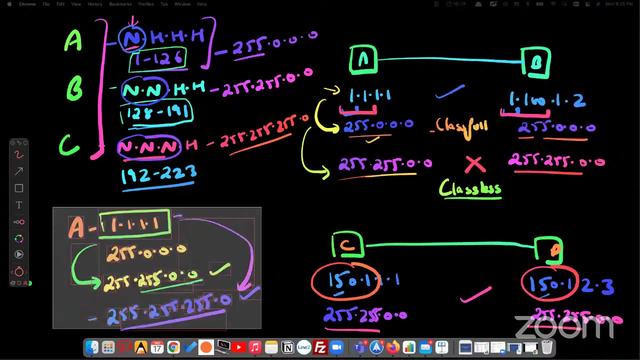 but if you put different subnet mask, then accordingly they are going to communicate. okay, so let's take example of a last computer class, what we call C class. so I shall remove this. okay, so let's talk about C now. if you have two machines and one IP address, 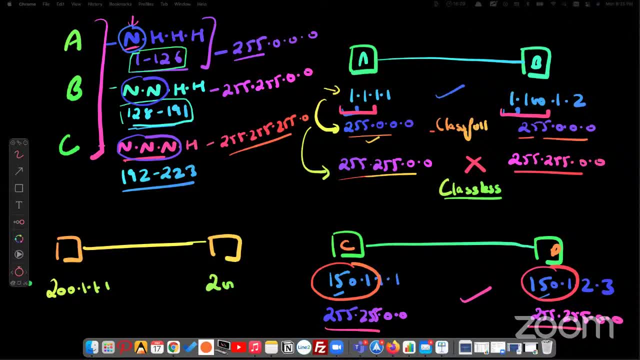 is 200.1.1.1 and 200.1.1.3, so tell me if they are able to communicate. yes, I have not given the subnet, so without subnet mask you can't say yes. okay, so three times two, five, five. now you can check. this is by default, so I'm going to check. 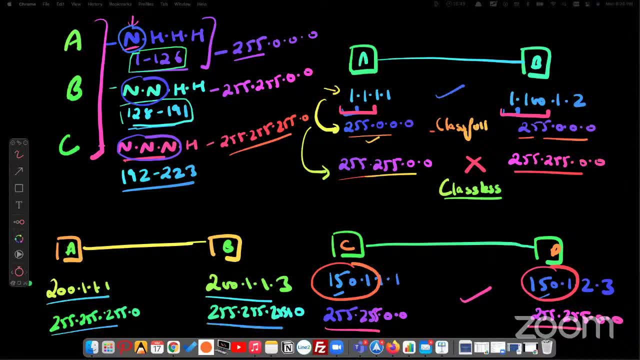 my first three digits because I have three, two, five, five. so your subnet mask represent Network bits what I said. your subnet mask represent Network bits, subnet Masky, network bits. because Amit here is able to understand, because this is normal language we can understand. okay. it how computers understand like this ip belongs to which network. so just count the 255 ip address. 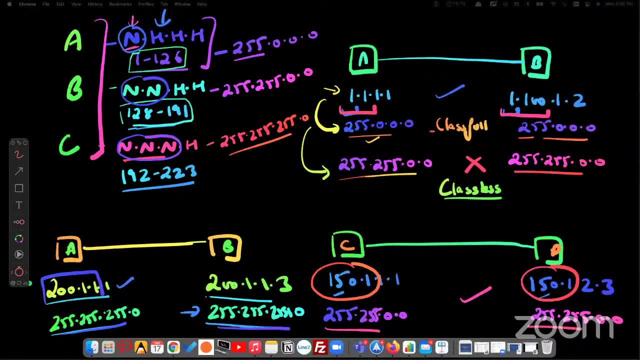 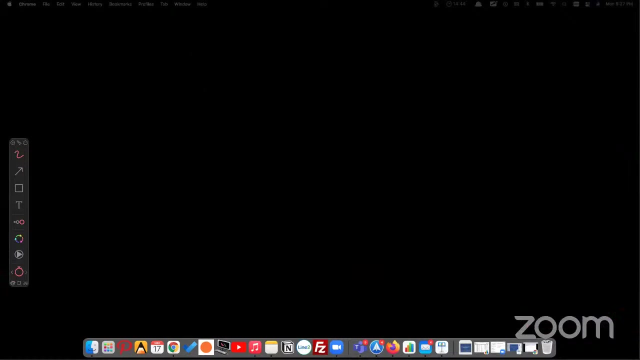 belong to this network and here also three type 255, so you can see network. is this? now you can check and compare? yes, our network is matching. it means we will be able to communicate. yes, everyone, yes, yes, clear, yes, yes, okay, okay. so so let's discuss about why we divide our network. 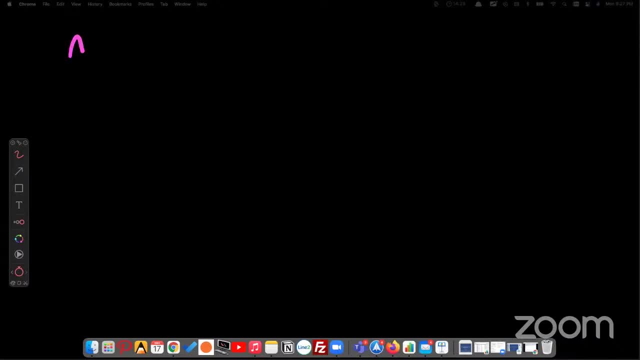 right, so this is normal ip address and a class, b class, c class, so you should understand. network part was n and host was very three parts. so every octet is how many bits a cocktail? okay, so you have eight plus eight plus eight. it means to the power of 24, right? so you know. 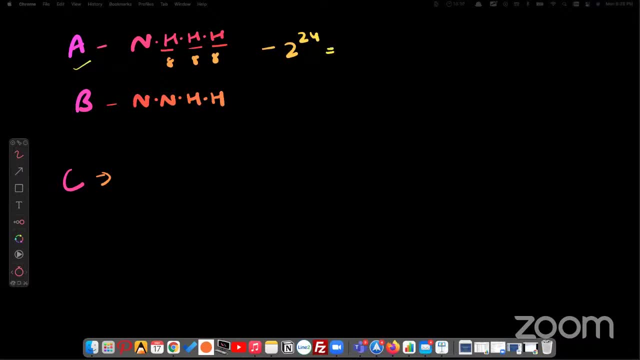 when you give ip address with class a, how many ips you get? one, six, triple seven, two, one, six. so it's a very big number, 16 million ips you can assign from class a. it means if your ip address start from one dot, zero, dot, zero. this is. 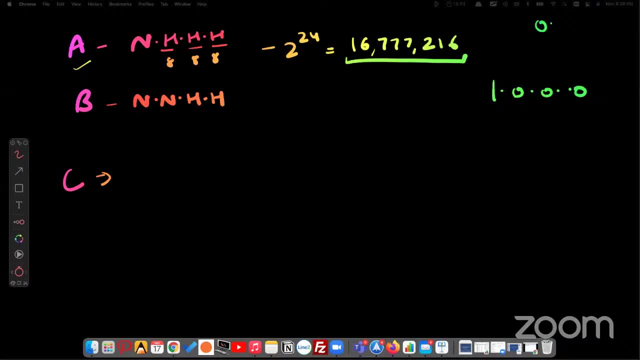 the starting ip address. so, like your timer starts with zero, zero, zero, zero, right, so it's like one, zero, zero, zero, because this is class, a network is same and network will remain same at the end. but this host would be maximum value is will be two, five, five, so your maximum value is two. 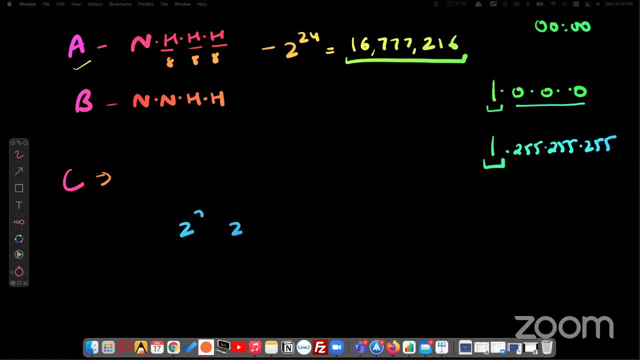 five, five. why? because you remember the table right, yeah, table, yes, yes, yes. so if you calculate all the values like one, twenty eight, sixty four, thirty two, sixteen, eight, four, two, one right, two, fifty five, yes. so if you get so, you get 255, and if you make all values 0, you get 0. so this is why all groups. 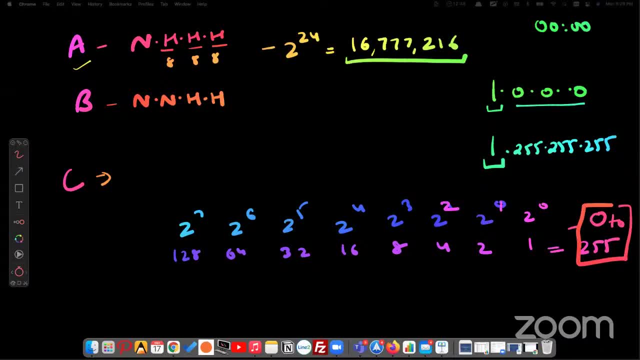 are from 0 to 255. so 0 to 255, remember now understand. so 0 say 25. this is the minimum, this is the maximum and all. so this is the range. so how many computers or how many ip you can assign this much, got it. so now, if you check b class, you have 8 plus 8, 16 to the power. 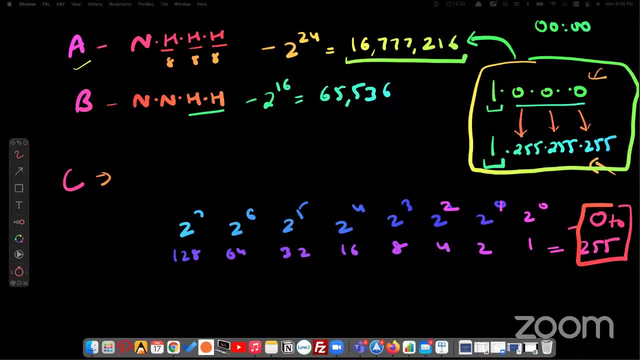 of 16 is 65 536 ips. so if your company is around 50, 60 000 or maybe that much team members, you can use class b, but if you are a home user you don't need a very big number. so to the power of 8 is. 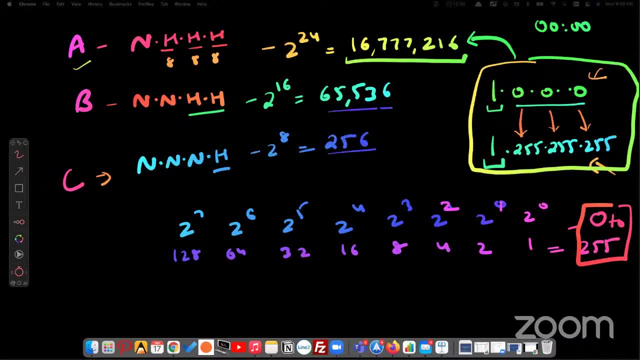 256. so now your ip addresses belong according to users. okay, suppose i have 500 users, so i'm going to use b class or maybe a class, but i can't use c class because it only gives me 256 address. you have to jump on 65 000 maybe if, like, if you have done your college. so mostly. 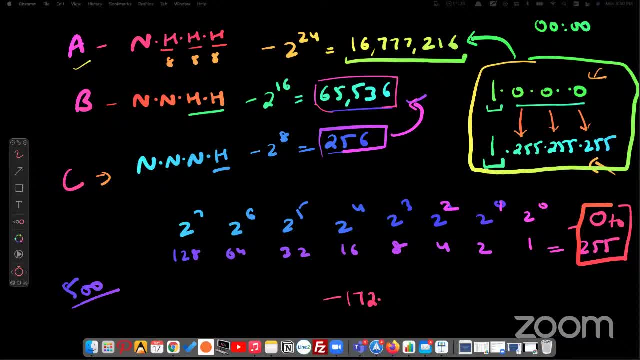 might be. you guys have seen 172 in colleges, campus mostly, but when you join any big companies they mostly use a 10 series something like that. okay, totally depends, company to company, clear: yes, everyone, yes, sir, yeah, yeah, yeah, okay good, any doubt, no, yes, no, oh, okay good. 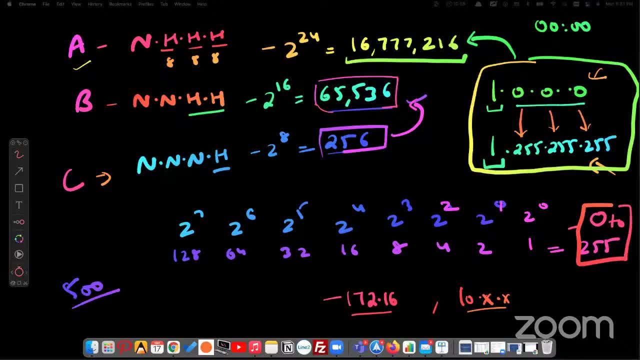 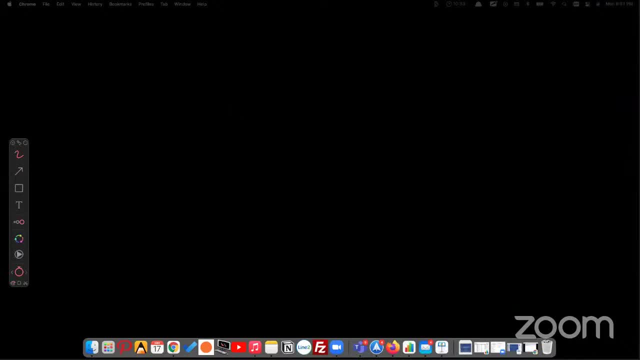 okay, this is basics. okay, so, some scenarios i'm going to tell you okay, so, uh, even though it's not a router class, but still i'm telling you, see, there is a company. okay, so generally we use a router. so why we use a router? so that your computers will be able to use a router, so that you can use a router, so that you can use a router. 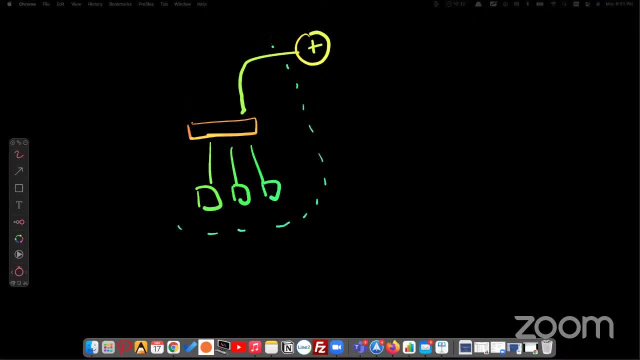 will be. suppose this area is your branch office in delhi or delhi. okay so 192 168 dot 1.0 slash 24.. so what is 24? we generally use? class a has one network part, so we call him slash eight. so b has two network parts. so what we are going to say? slash 16, yes, so c has three network part. 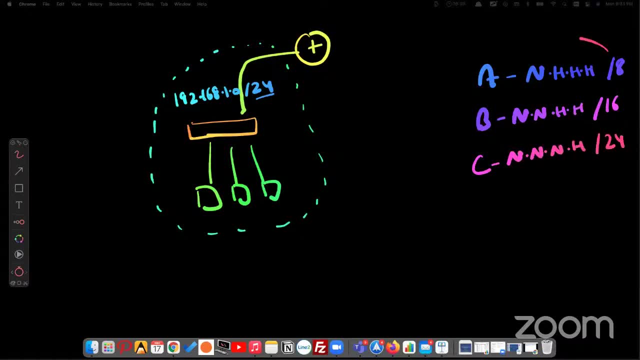 thank you, so we call 24. so this is also called cidr- classless inter domain routing. okay, so this is just a fancy name. you can call this slash value. that's it. so you can call this cidr also. okay. so now, if this is slash 24, obviously this is class c. 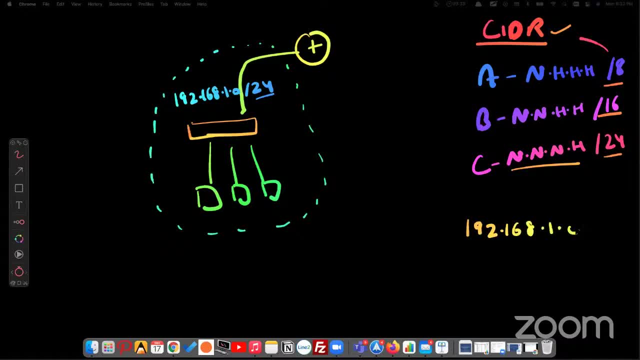 so if ip address, tell me if ip address start from 1.0, so your network will not be changed, yes or no, the network change yoga, right, so the ip will go from 0 to 254, 5 right, so the total ip address you get is 256. right, so you have another office, maybe somewhere in a different location? so might be this. 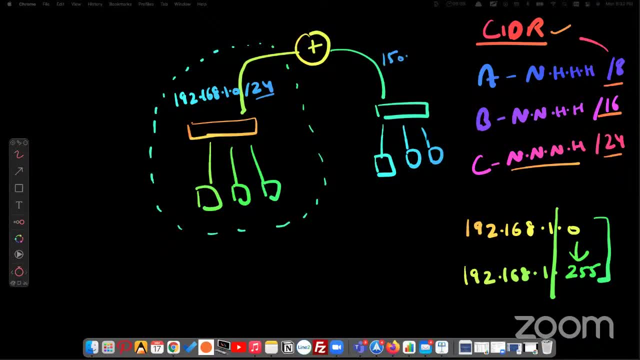 side you are using some 150 because it's a very big office, it has many user, or maybe thousands of, and here you are using slash 16.. okay, so it means this is a different network. this is also different network, so we use router device. we use router so that you will be able to communicate with. 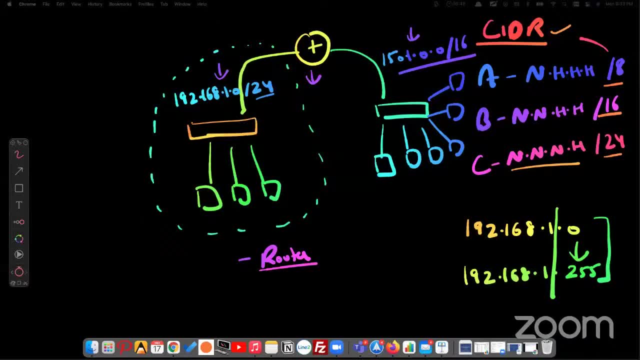 the different networks. so why we made router, why internet has a lot of big, big routers? because router is a device which is used to connect, to connect two or more different network. okay, so, guys, now you understand why internet big routing, internet table, like, why we have routers everywhere. when you get internet connection at your home, when you get 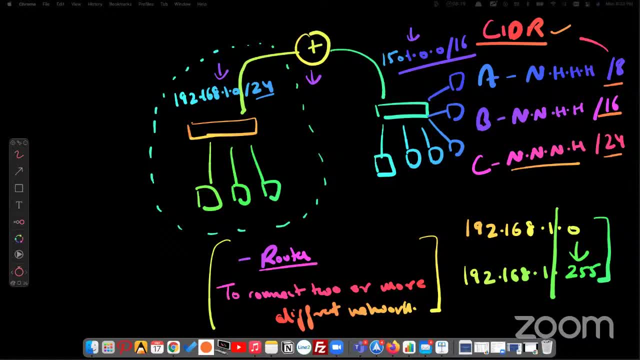 internet at your office when you get anywhere, you need router device. mostly why? because you are having different network and internet is on different network. all, all networks are different and network of networks is known as internet. okay, so tell me, if this is class, which class is this? c, c class and this is class. 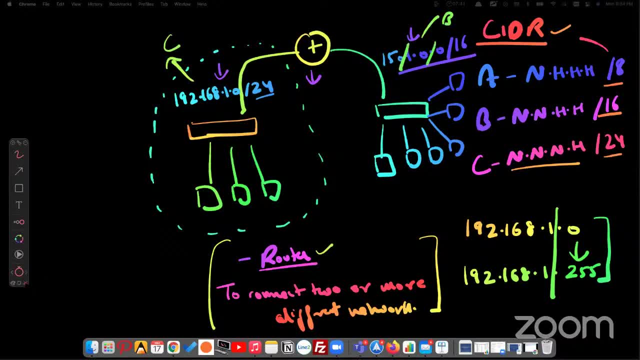 so class c and b if we use c class here. so router is required. no, oh no, sir. no, network not needed. network is needed, sir. so 190 to 168 5.0. now you can compare 190 to 168 1.0. so i told you to match three networks. so if you match three, 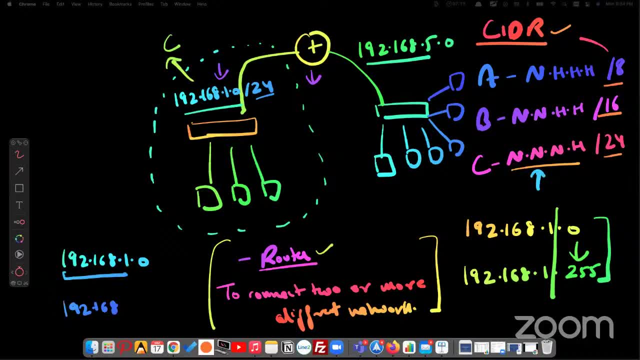 network with another ip 190 to 168, 5.0, so we can able to match. no, sir, no, when we will not able to match, it means we need a device which is called router. got it, yes. so this is why router is more popular and this is why network engineers learn. 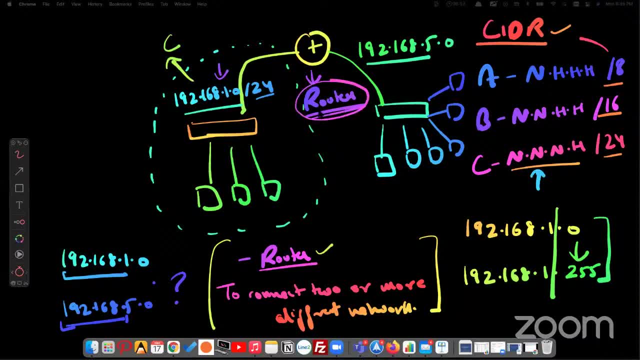 routing, router routing, okay, whatever we do on router. so every network engineer should learn about routing and router configurations, because most companies hire network engineers so that they can able to configure router. okay, clear, yes, sir, okay sir, yeah sir. i have a question one, sir, they hear abc difference classes, okay. 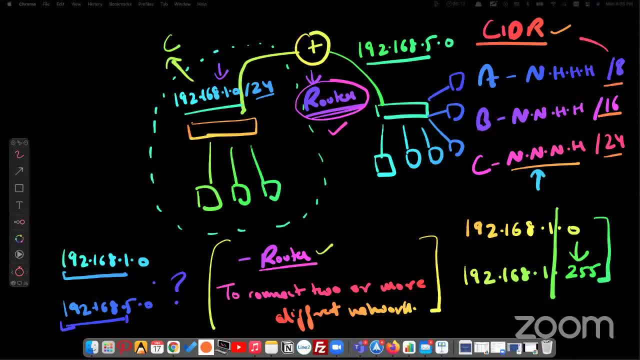 their network part is first one and another host three. okay, sir, then host means the computers are mainly nodes, and network means what? network means that you belong to my network or not. that is like a particular area. this is my network router is going to share all the network information to all other routers. it's like your. 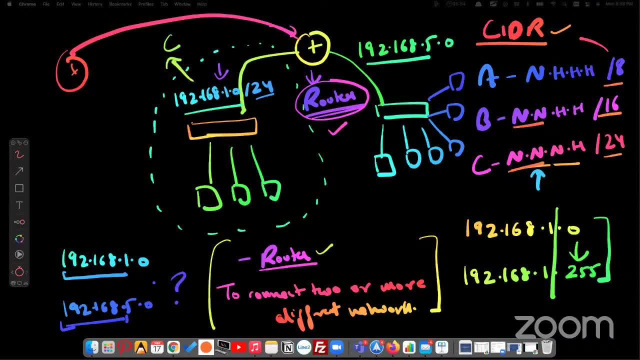 home address. your network portion is like your home address, okay. or maybe you can say that it's like your street address and host is your home address. what do you mean? uh, home address or network means- i'm just giving example. don't say this interview, no, no, sir, okay. so just understand. network means your city address or like your. 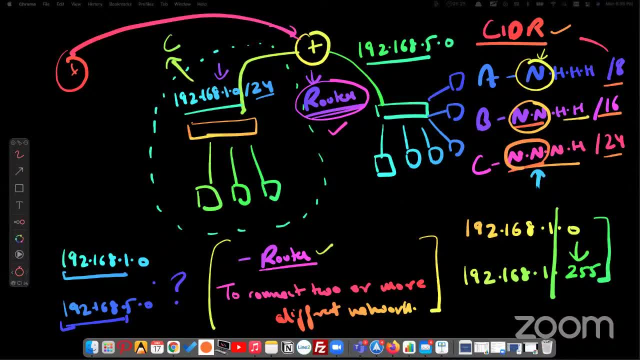 home address. so example, take example. okay, so network is like your home address and host is your name, suppose if anybody wants to send a courier to you, i can't send courier to santanu, i have to share. put your home address yes or no? yes, sir, right, so when the 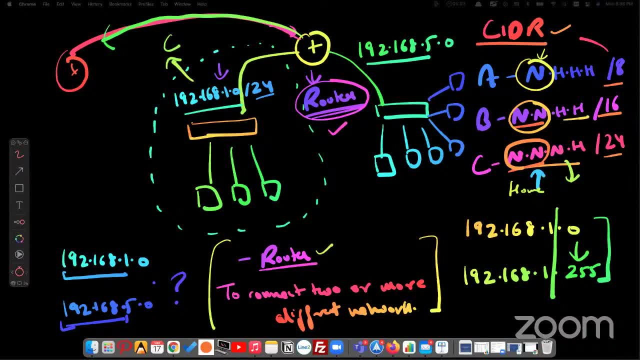 router when this router share information with another router or share information with internet. so this router is not going to share all 50 computers, thousand computer information. the router is going to share only the network part to another router, got it. so your router will only share the network part to another router to the whole world. 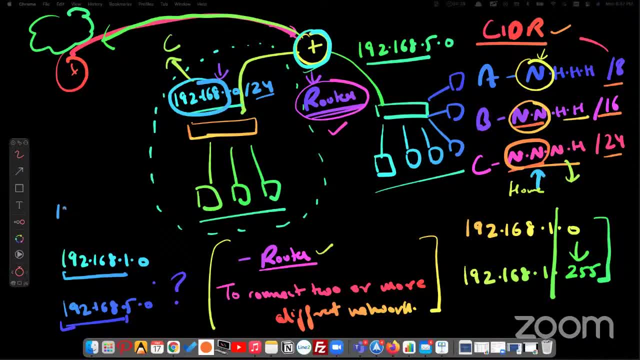 okay, suppose your ip is your computer. ip is 192 168.1.1. tell me what is your network id. this is your network, yes or no? yes, sir, so your router is going to share this information to another router like this. so router is not going to share this information to another router like. 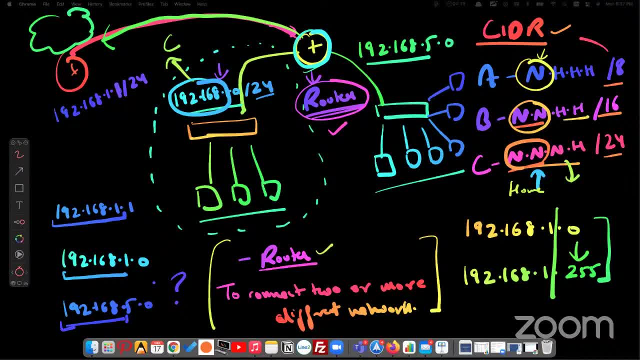 this. so router is not going to store 1.1, 1.2, 1.3, because these are your, like, all family numbers, family members name. we are going to only put the home address in our routing table. i told you right. so we have a global internet table, global routing table. 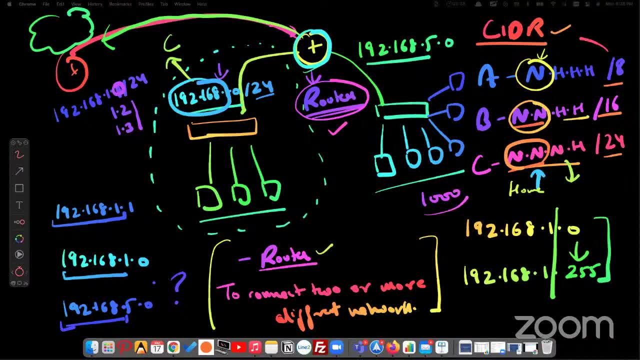 so if we are going to put a thousand, billions of ip addresses are assigned to you, all users in this world. so if all routers are going to put all the ip addresses, then it is going to have a problem, right? so just understand in this way that we 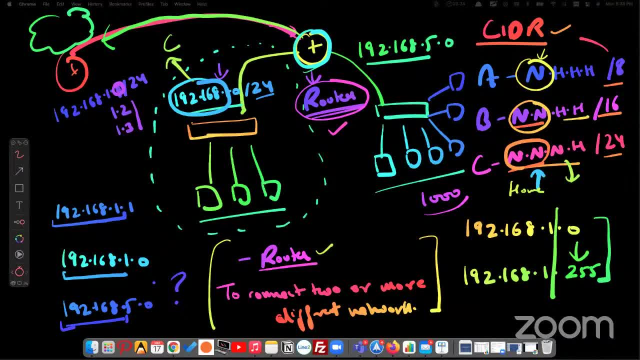 like billions of population. when your courier guy come to you, they can't. they don't come to you. they actually come to your network. they actually come to your home or office address. right, because it is easy. if you take the name and roam around the streets, bro, how far will you reach? 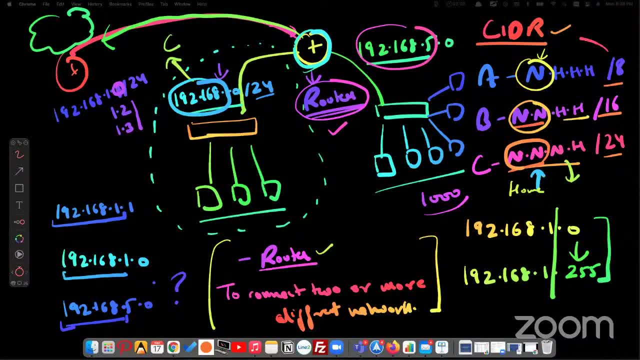 yeah, so understand. network address tells, like all routers, router share the direction that okay, go from this side, go from this side, and router checks: okay, home address is there so it delivers to your switch and switch will broadcast: who is 190 to 168 1.1, and your computer say: i am 192 168, 1.1. this is. 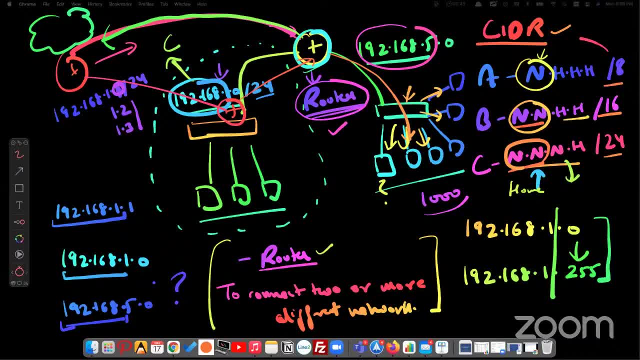 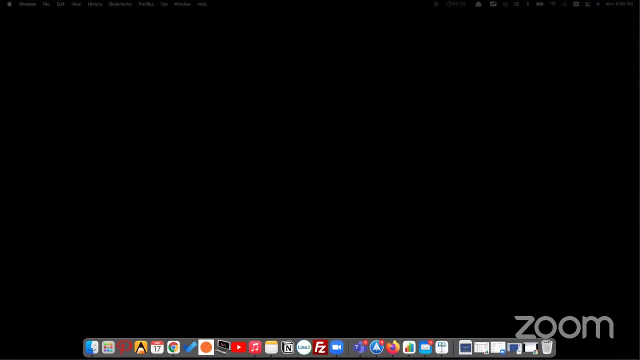 how it works. small devices also have a routing isp connection. okay, so let's come back to our sync. so now you understand: whenever you give an ip, whenever you assign any ip like 192 168 1.1, like 192 168 1.2, so all these ip addresses have 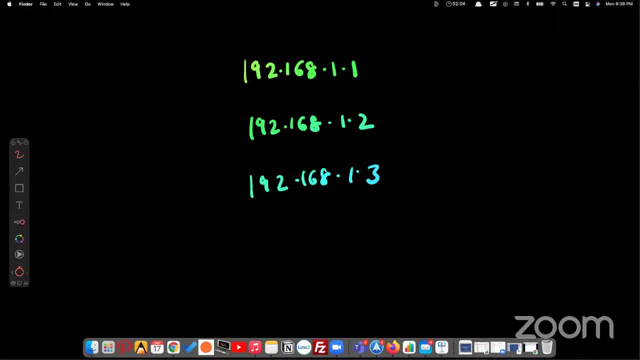 their home address, or called house of ips, which is just remove the host ip and you get your network id right and put zero here. that is network id of all users, yes or no? yes, sir, yes, sir, yes. very simple. so when router is going to share information to any other router, or maybe to internet, 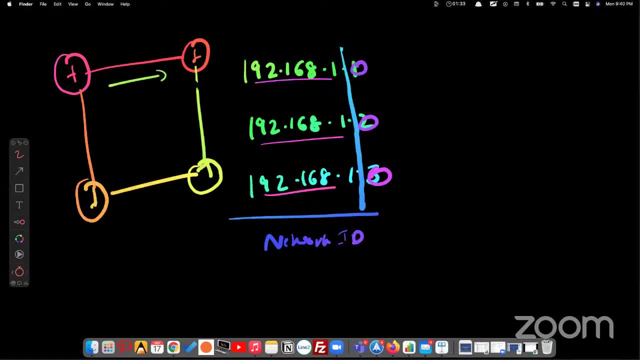 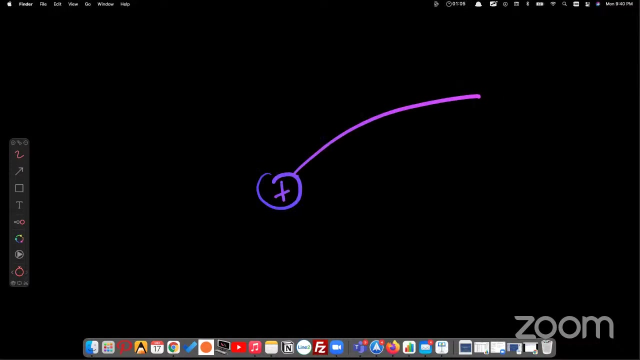 so all router- you know this is like. all routers- share their network id with each other. so all routers are sharing their network parts, not their host ids. what it? yes, sir, now it's clear. so this is why network id is important. i hope now you may got it why we use network ids: because all routers only share network ids with. 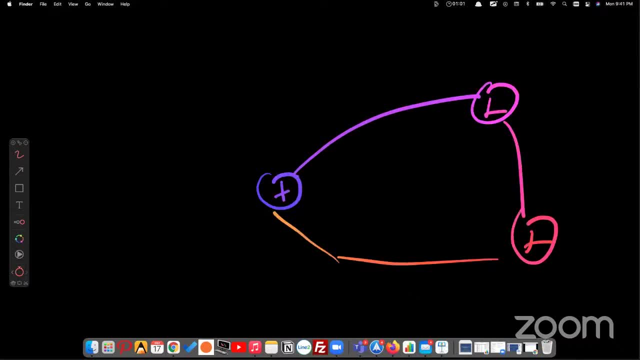 each other. okay, yes, sir, clear, yes, sir, okay, good, okay, and i want to ask you that if you have any problem, or maybe want to post something into the chat room and you have any question, anything you want to discuss, you can text me directly in chat or maybe send to the facebook group. just let us get to it. 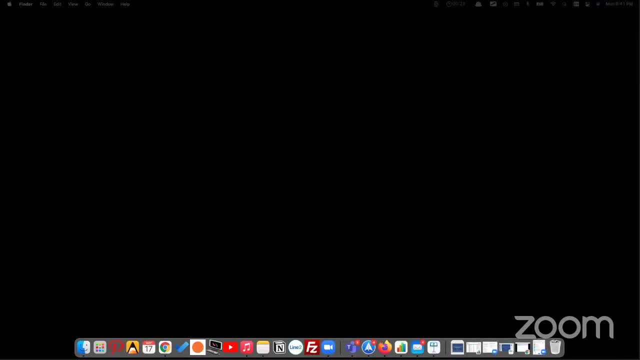 and or you can also use the chat room to ask for any more questions. if you have any question, please do not hesitate to send me a reply. i will be happy to reply to that. thank you for watching this video. if you have any question, please do not hesitate to write in the comments and we will hear from you and we will see you in the next video. 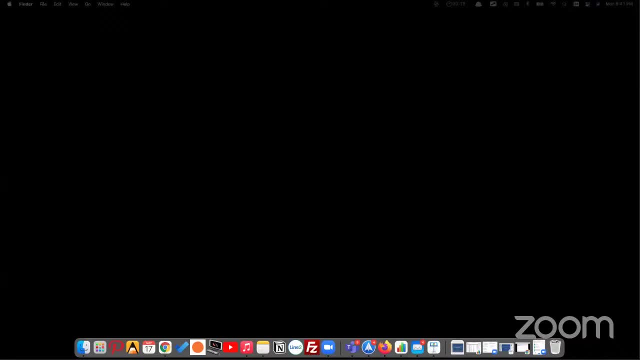 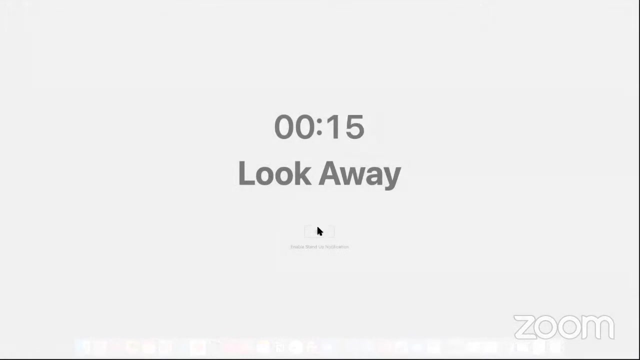 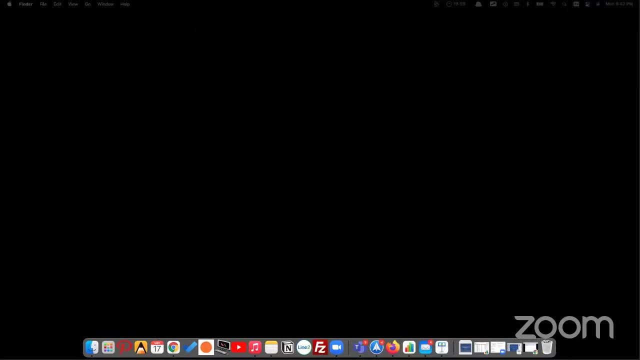 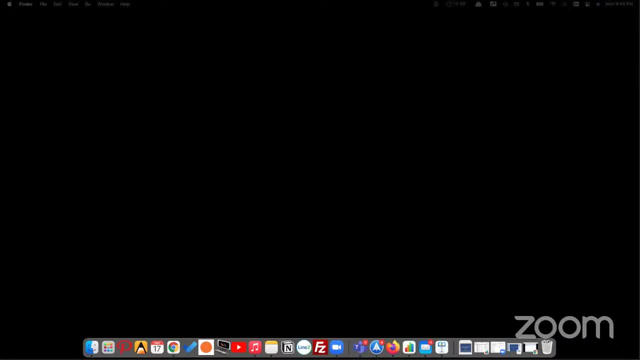 you, you, you. okay, i'm back. so, guys. so let's understand what is subnet mask? more so, i told you subnet mask represents network bits. yes, represents network bits, because your computers need extra information that computers belong to which network. uh, nothing wrong. i was on break for two, three minutes. 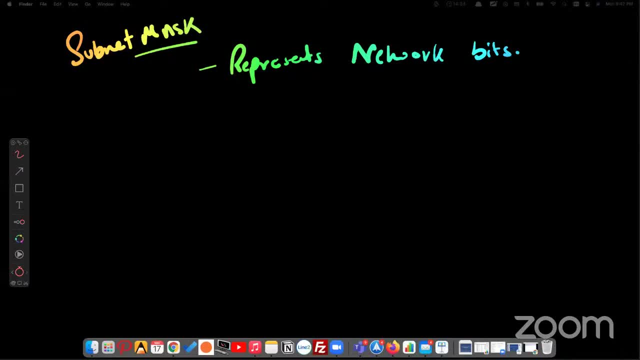 okay, so represent network bits. okay, so i'll explain you something. okay, so slash 8 was 255.0.0. how? how we got 255? because if you calculate the to the power of hours, so if you plus all the values, what you get, you get 255, right. so this means eight. eight means eight bits: one, two, three, four, five, six, seven, eight. 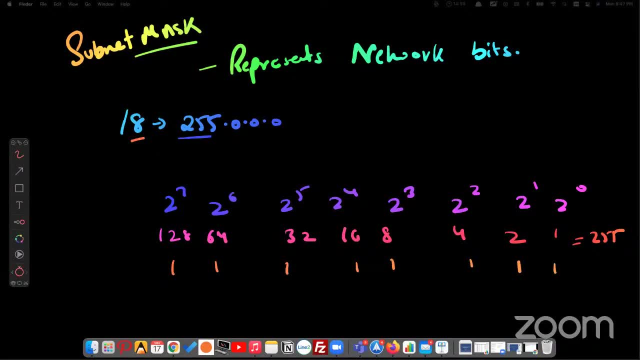 so eight means 255. but what will be the value for slash nine? so obviously, how to calculate for nine. what is the subnet mass of the network bits of slash nine? so slash eight, slash nine means how many network bits. so what is slash nine? so it means when two computers communicate with each other. 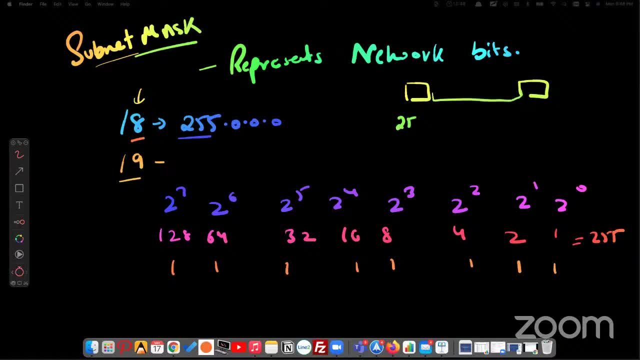 right if you give any ip, but if you give 255.0 something slash eight. so first let's get the subnet mask for slash nine. so what will be the slash nine? oh, so, obviously in the subnet mask we go this side. but let me see how do i do this. 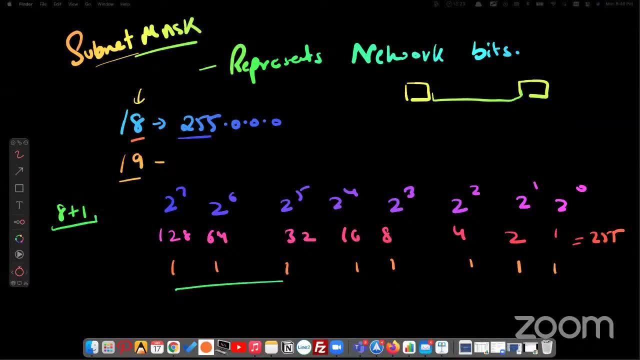 now all right. when you set up the subnet to slash nine, you just have to get guys, so it just há cloud, or however it is called. so on my table we have subnet allora and and 128, so on another side let i just add um. okay, so save distribution to add Sebastian here. 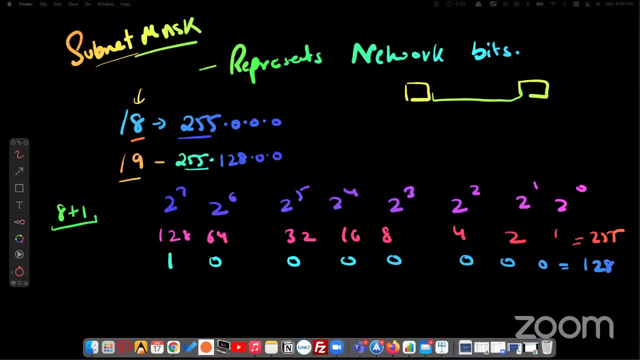 dot zero, dot zero. very simple, right. and if i give any value for slash 10, let's suppose eight plus two, eight plus two. so it means eight means two, five, five. but two values, two means one, one. so you calculate. you get what? one ninety two dot zero, dot zero. so let's not calculate, because 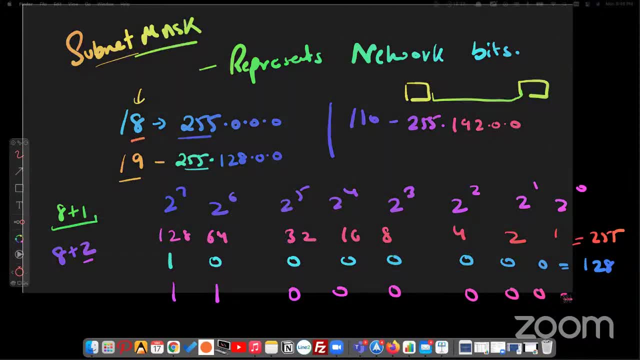 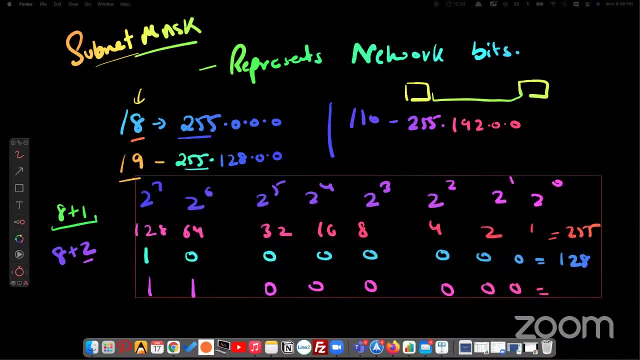 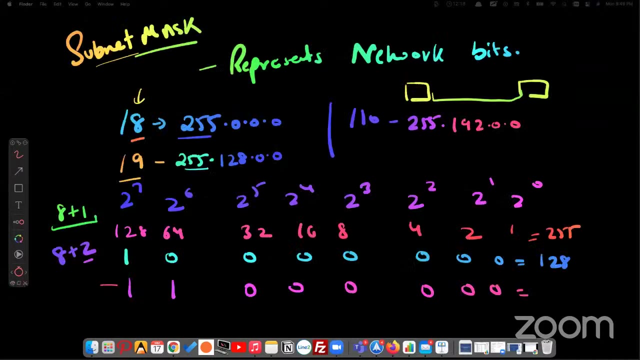 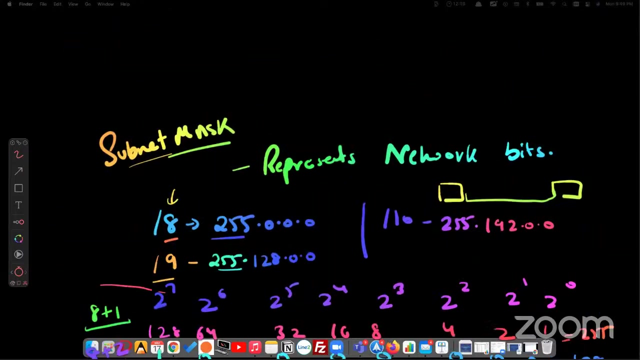 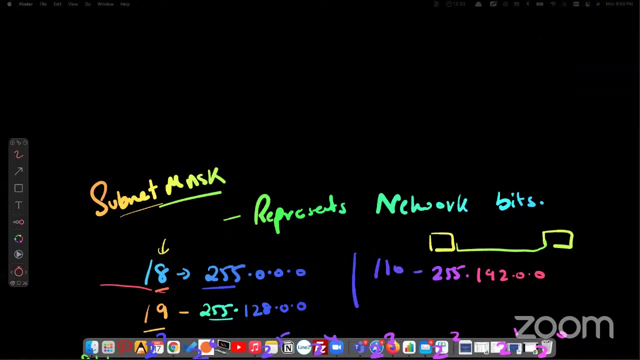 it's a little complex formula, but i wanted you to explain how we calculate, so i'll tell you the shortcut. you don't have to learn or write this. so there is a shortcut. okay, so, shortcut, okay, okay. so, guys, shortcut is for one bit. always add 128. 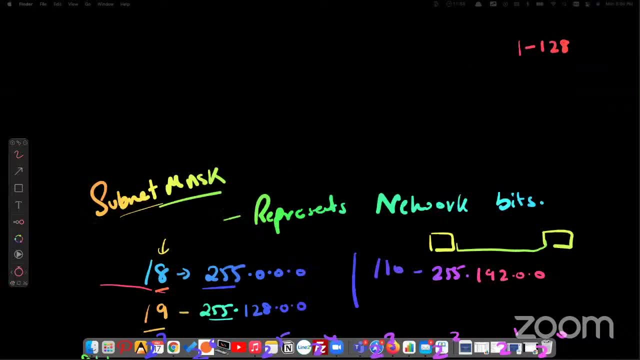 for one bit, always add 128. whenever you get two bits extra, you get 192, three bits. if you plus first three numbers, two to four, four, two, forty. please note down this, it is going to help you. okay, just i am adding the values. first value 128, 128 plus 64, 192. 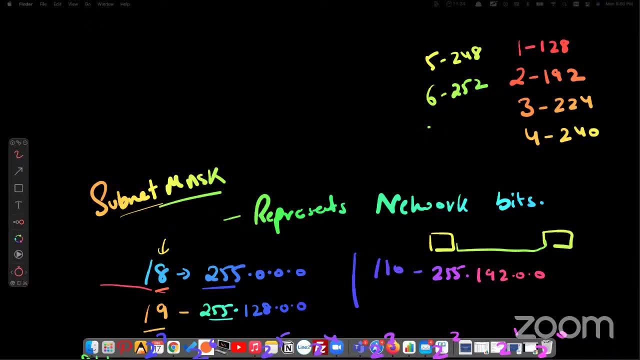 128, 64, 32 is 2, 2, 2, 4.. so this is the value you will be getting right. so now you calculate very simple. suppose slash 12, so 12. how you make 12? uh, 8 plus 4, 8 plus 4, right, 8 plus 4.. so 8 means 2, 5, 5. 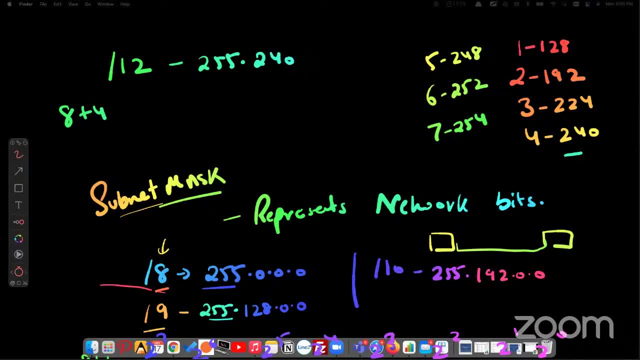 and 4 means 240 dot 0.0. very simple. slash 15, tell me, for 16, 8 plus 7 is 15.. 8 means 2, 5, 5 And 7 means 254.0.0.. Very simple. 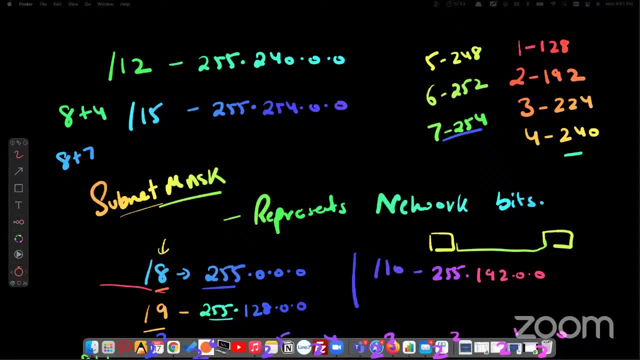 Yes, Ajit, you are correct, They are in the same network If we give slash 20.. So 20 means I will tell you. now Do 20.. 8 plus 8, 16.. 8 plus 8, 16.. 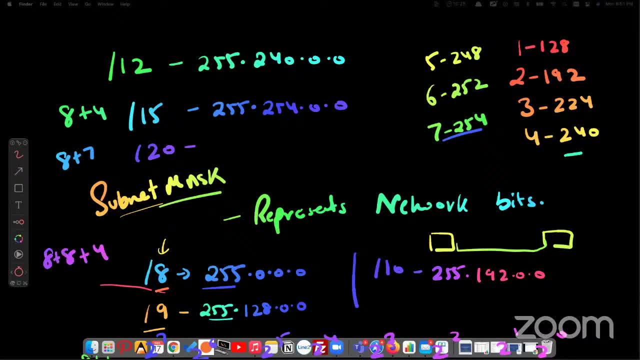 8 plus 8, 16.. 16 plus 4.. So it means 2.. Whenever you see 8,, it means 255,, 255.. And 4 means 240.. Very simple, Let's calculate for 18.. 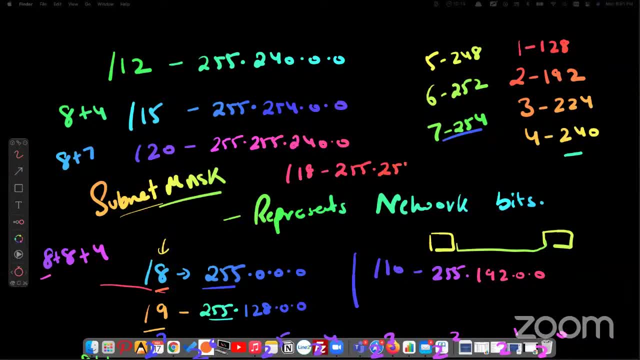 So 255.. 255, 16.. 16 plus 2, 190.. 2.0.. Yes, Nainjyothi, Did you understand everyone? Yes, guys, this is very important And you have to learn this formula if you don't know how to calculate. 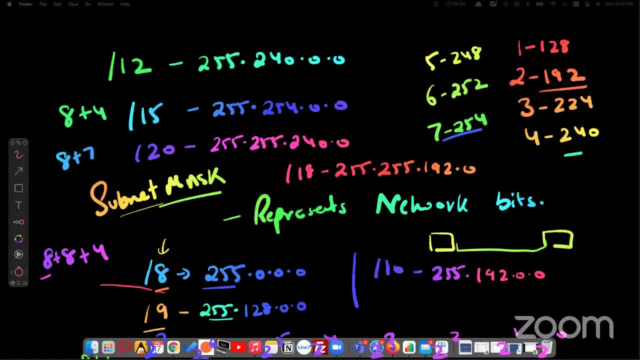 Even I have given you the information how to calculate. Yes, sir, Yes, sir, Yes, Nainjyothi, Yes, sir, Yes, sir, Sir. I have a question. sir, Yes, Sir, I mean from the default value that network ID is increased. 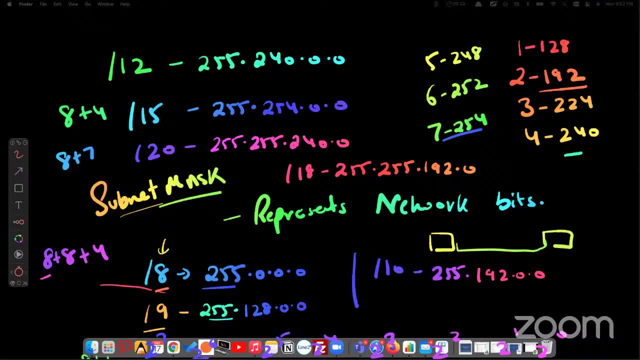 Yes, sir, Yes, sir, Yes, sir, Yes, I will tell you why we use subnetting, But now understand how to remove subnet mask. Sir, can we make slash 8 to slash 7, sir? No, no, no, no. 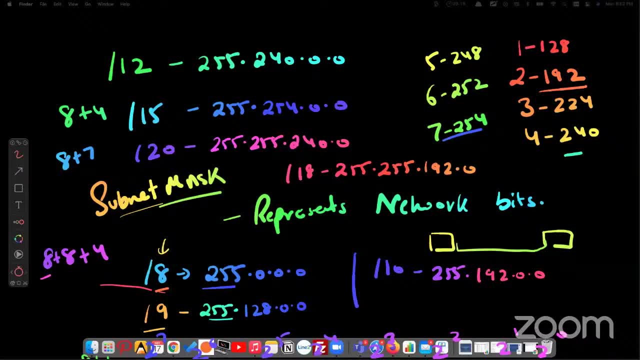 We should not use. You can't go less than 8. Because the first number actually represents your network, Right? So you can't go less than 8.. Yes, sir, Yes sir, So let's go further, Okay. 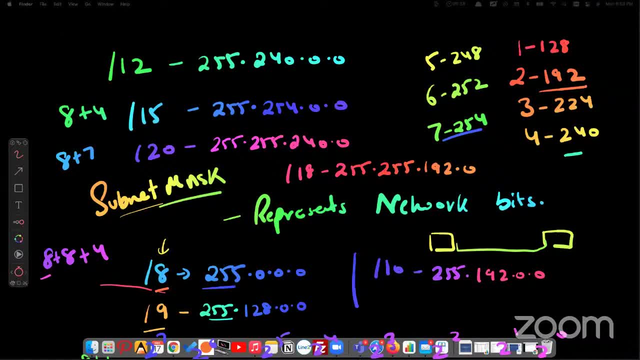 So, guys, this is highly important. Please take screenshot, or even the class is getting recorded for you, Don't worry, But this is very important, Just write this. So why? I'm telling you? Because this is the first step to learn submitting. 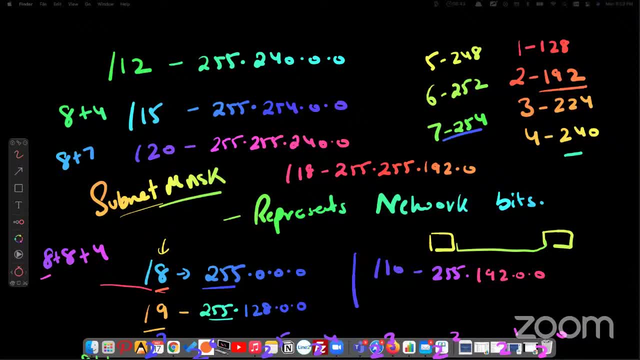 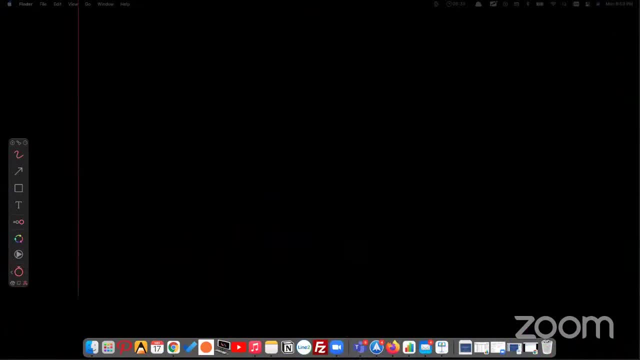 You should know slash 15 is called 254254.. Zero like this. Okay, So let's do more practice. Let's do one more practice quickly. Subnetting is all about practice, Right, But you need better strategy. So if I give you slash 25, just divide into parts: 8 plus 8 plus 8, 24 plus 1.. 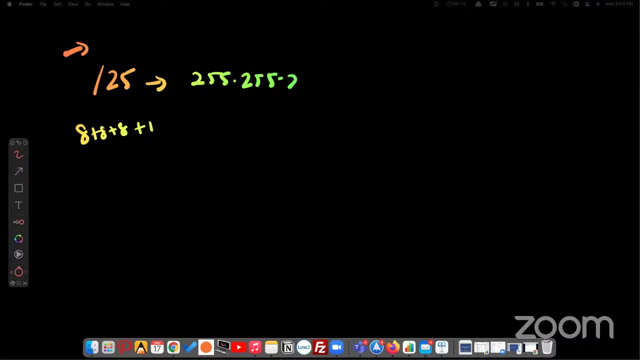 Tell me your answer: 255255255, 1, 28.. Yes, 128.. Yes, Slash 27.. 255255255, 24, 24 plus 3.. Got it? Yes, sir, 8 plus 8 plus 8 plus 3 slash 30.. 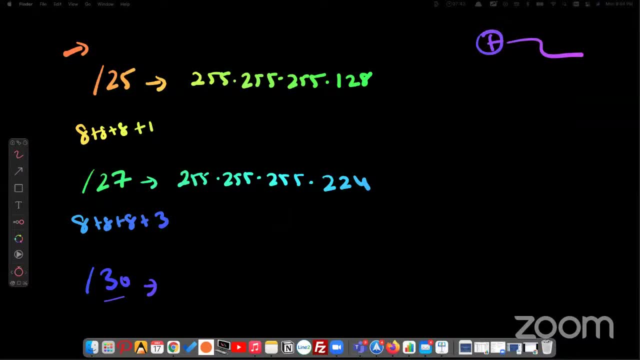 Where we use slash 30, just for your information. I'm kind of lost. Yes, yes, Tell me, How are you getting 224 for that last octet? Because there was a shortcut Like for one bit. you get 128. 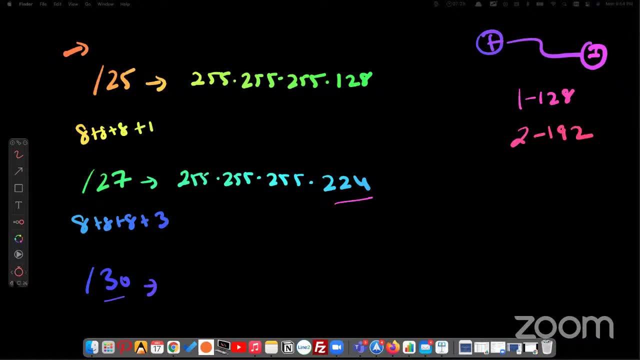 For two, you get 192.. So how I calculated this? So every octet, four octets you have right. So every octet you have to the powers: Yes, correct, Yes, Yeah, So if we talk about slash eight, so it means you have eight octets. 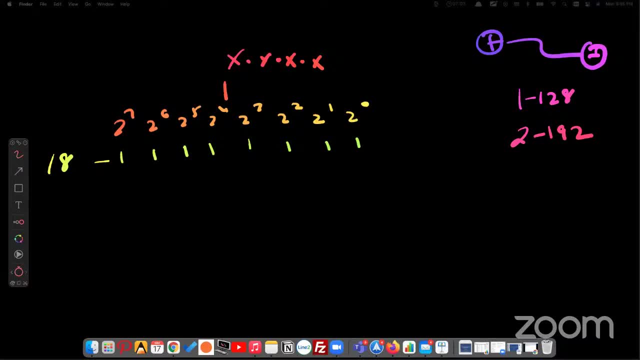 Yes. So if we talk about slash eight, so it means you have eight octets. So if you calculate once, this is, And if you plus all the values, their corresponding values. if you plus all the values, you get what? 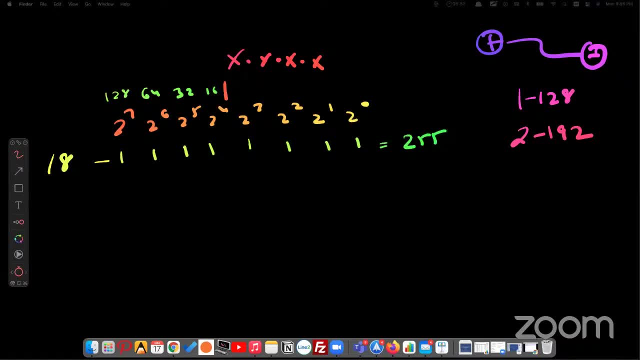 255, right. So in the second octet, because this octet is completed, eight bits is completed. But when you have nine you have to jump on the another octet, because eight is completed. Now, in another octet you have same values, but you will take only one here. 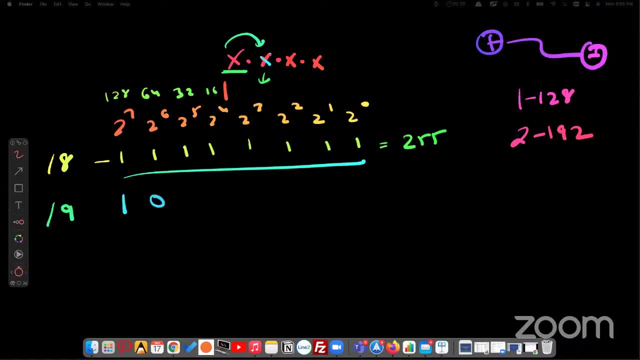 Eight, Eight plus one, nine, And if you calculate, what do you get? 128.. Yes, Yes. So this is why I have written: one is equal to 128.. Now another: if you take 10, for 10,, what do you have to take? 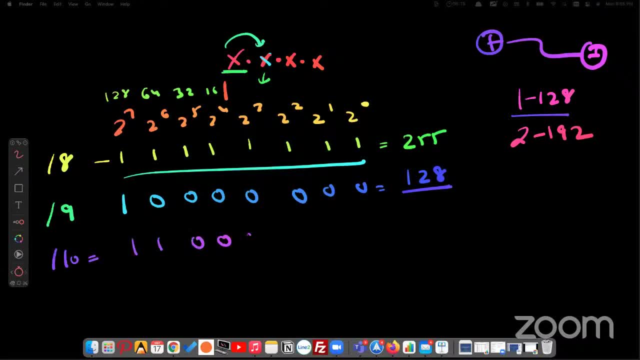 You have to take two bits more, right? Yes, So for two bits. if you plus this two bit, 128, 64- is 192.. 192.. Yeah, Yeah, Yeah. So now three bits. if you take three bits, if you plus 128, 64, 32, you get 224. 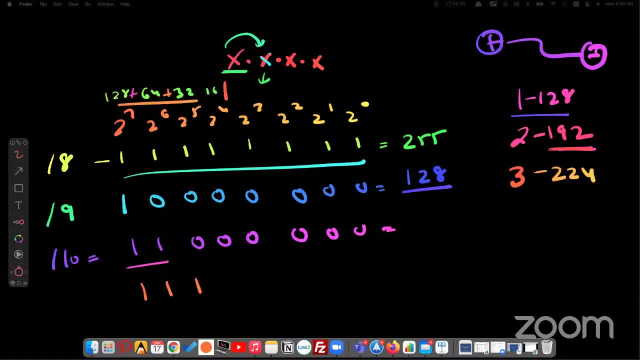 That's what we're trying to draw and the type of character, because we plus, we add when we say we want 11, this is my slash value. I want to write a subnet mask. How I'm going to write. first, this is my eight bits, right. 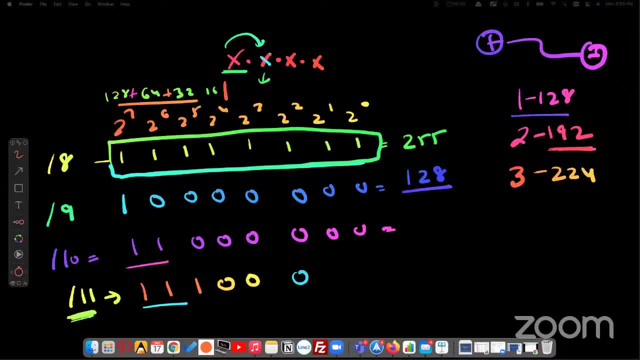 This is it. I'm going to write extra three here And if you plus, If you plus the first eight, you get 255, and for remaining three, you get 224, 128, 64, 32.. You want more clarity, or it's clear? 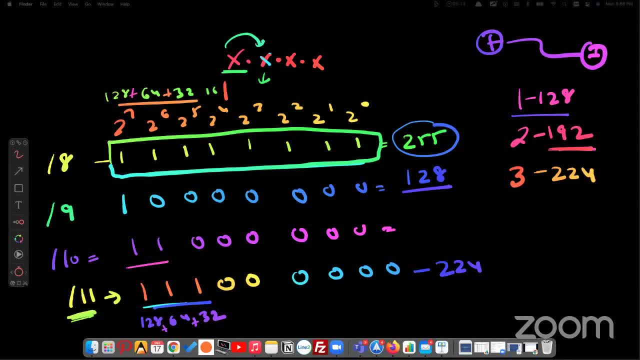 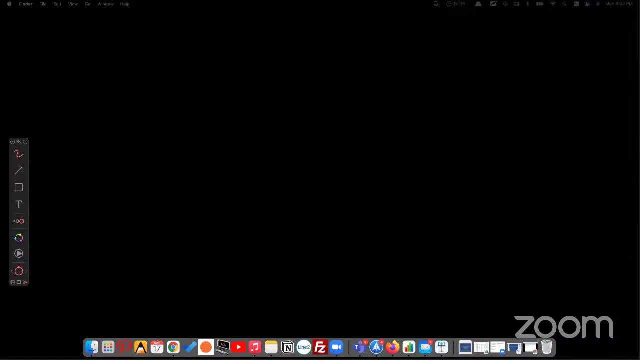 Um, I think I need more clarity. Okay, So just calculate. Okay, So the another way to understand this. So I have to write all four octets. This is the last option I have, So please focus to. so all four octets will be written like this: to the bar of seven. 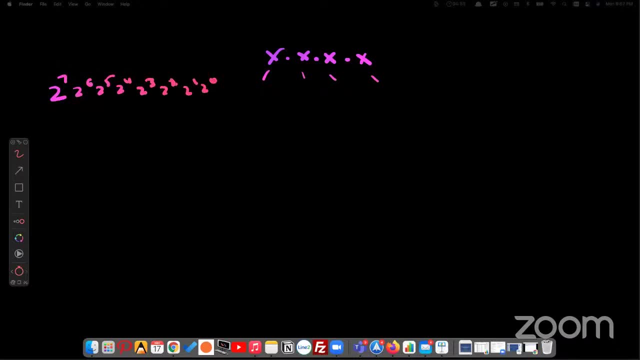 No matter what to clear. First octet written. second, one same, And uh, I guess Okay, Second is clear. Third octet- Same, I think you know, because eight bits is represented like this only. I hope that makes sense. but why can't I play hockey? 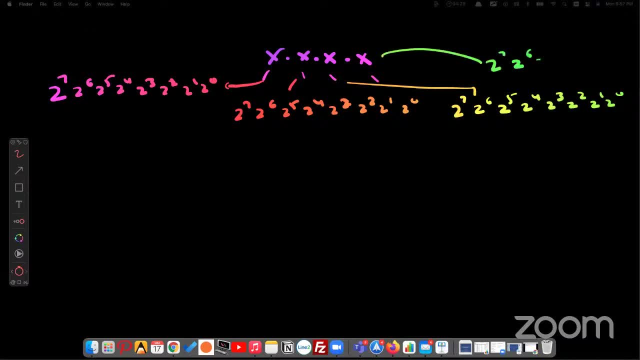 Yeah, The power too. Yeah, So all octets are like this: Clear, Yeah, Okay. So if I talk about slash eight, it means you need to write one one eight times and rest All octets will be just the hockey player. 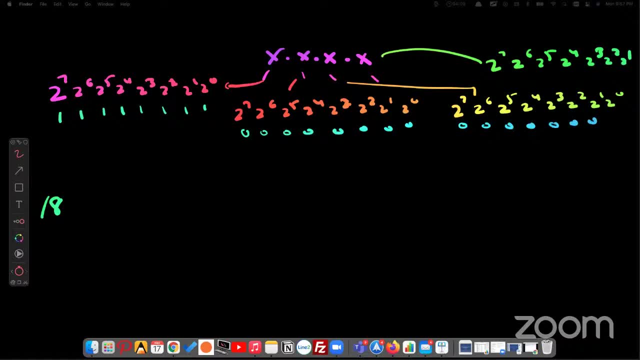 Right, Yes, And if I talk about slash 10, 10 minutes, 10 bits, this, eight minutes, eight bits. And if I talk about 10 slash 10, what does 10 means eight, and you have to take nine and 10 from here. 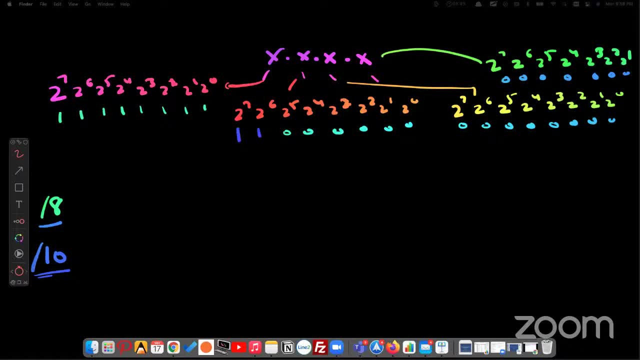 Yes or no From second octet: Yes. So if you plus this value, what do you get? Two five, five. Yes. And if you plus this value, what do you get? Two five, five. And if you plus this value, what do you get? 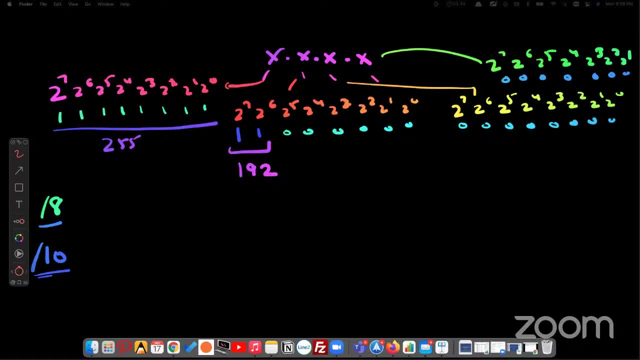 192.. The way that you feel part of the community by by being engaged. Yes, Third octet is zero. Fourth octet is zero. So slash 10 is a two, five, five one, 92.0.0.. 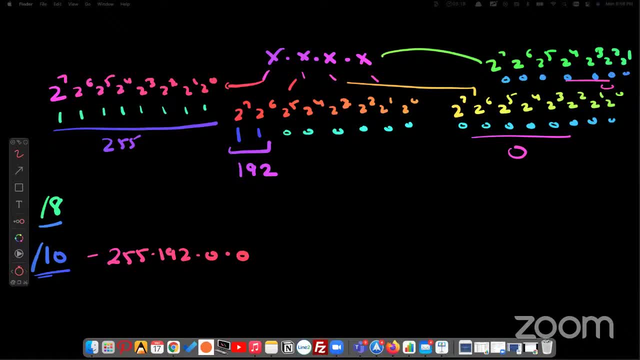 Yeah, I think I see how that works. Yeah, So now, if I talk about slash 11,, 11 means eight is already set, Eight is already set. I need one extra. I want to borrow one more. So if you plus this, eight is two, five, five, always. and if you plus three, you get one, 28,, 64,, uh, uh, 32, so that is two, 24.. 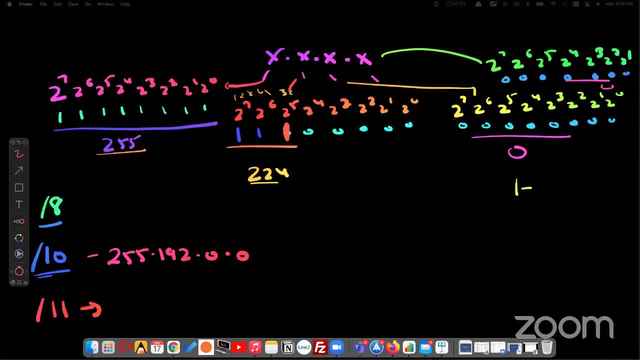 So you don't have to write a very big formula. This is a shortcut. for one bit, We always get one- 28. for two bits, We always get one, 92.. If we plus three bits, we always get two to four. If we plus four bits, we get always. 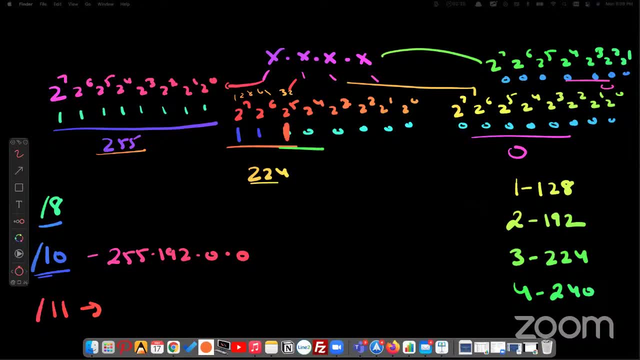 Two 40.. Yeah, If you plus five bits, we always get two 48. for six bits, We get two 52. for seven bits, We get two 54.. So this is what we get If you plus eight. you already know the answer. 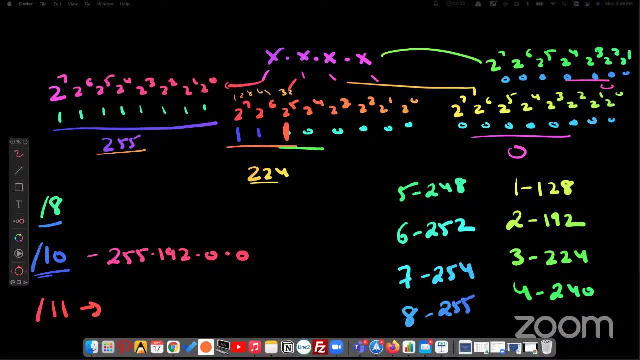 What? 55. Yes, Got it now. Yes, Okay. So, guys, now you're like a, what we call that homework in schools. right, I want you to write all values from eight to 30. Okay, Okay. 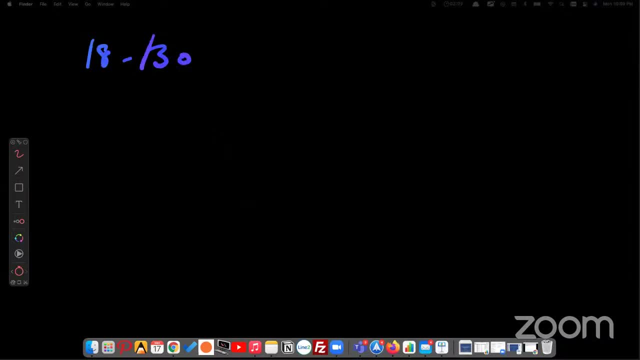 You can also get the chart also from Google if it checks a slash values or something like that. but please try to just write down from your end: slash subnet mask. You can just type subnet mask on Google, just type subnet mask and on the images: 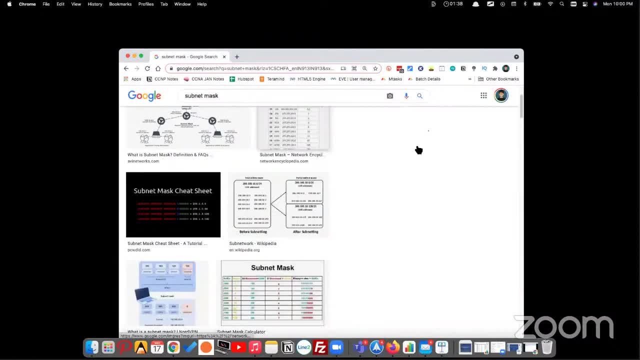 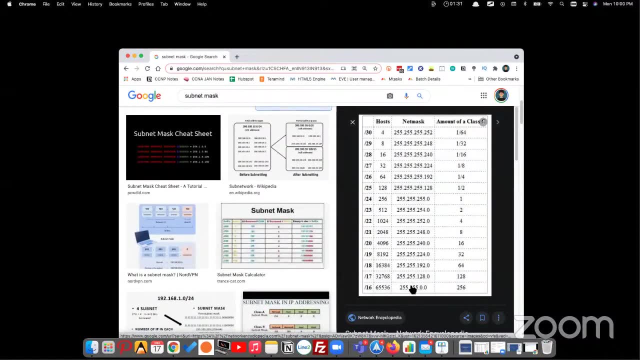 So you can see there is a very big chart, right. So this is All values. You can see, 16 is two times two five five, Okay, And the 17 is two five, five, two, five, five, 16, 16 plus one one extra bit is added one: 28.. 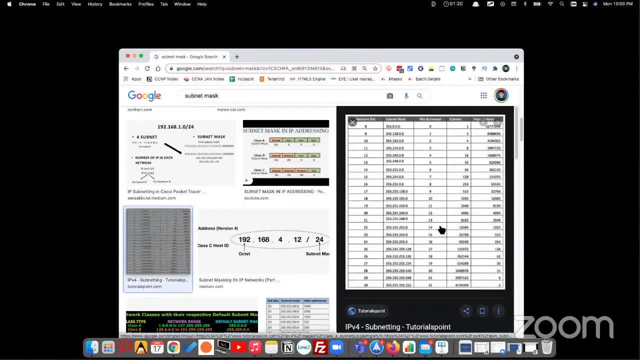 Okay, So you can just check this one. So that is a simple one, Okay. So, guys, I'm going to share you some notes, what I have written on my screen, and whatever is this, This image. I'm going to share that with you. 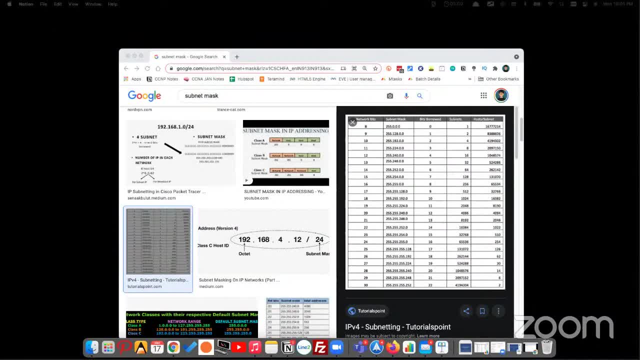 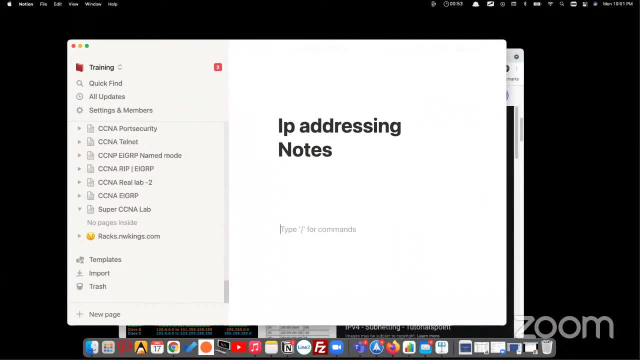 Okay, So this is IP addressing, So this is uh, okay, So I'm going to add this note, So please bookmark this for a few days. So this will be the same link You have to check the notes, Okay. 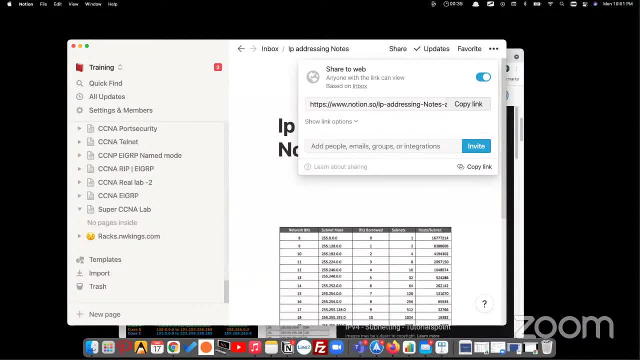 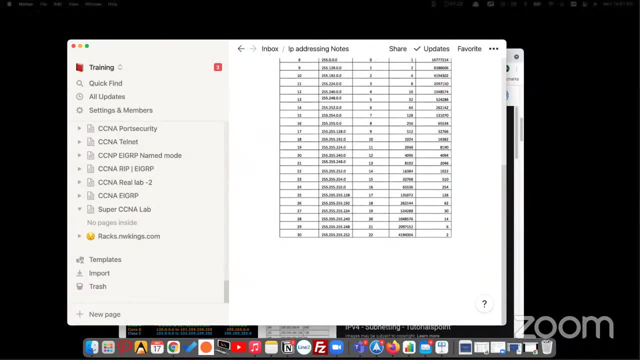 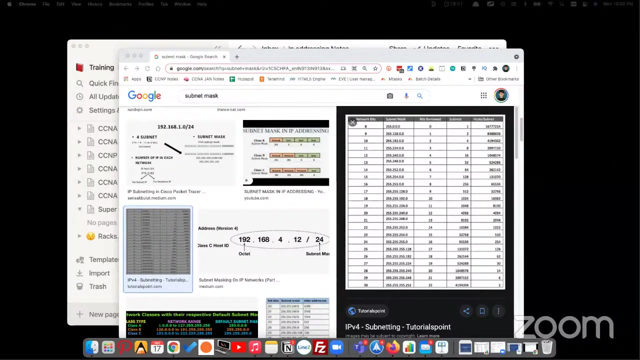 Please bookmark this link And I'm going to upload this into our portal, Okay, So Just hold on, Let me give you something IP addressing, if I have. Oh, Oh, Oh, Oh, Give me one minute. Hello sir, yes, yes, but love you. 8 to 30 sub maximum subnet, I mean. so this is IPv4 and 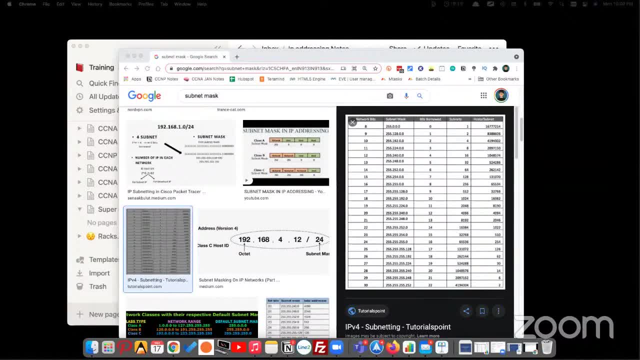 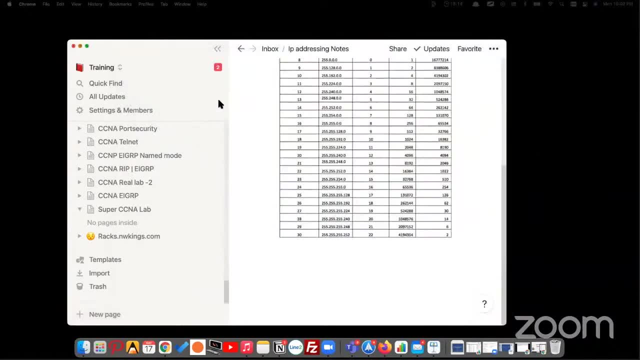 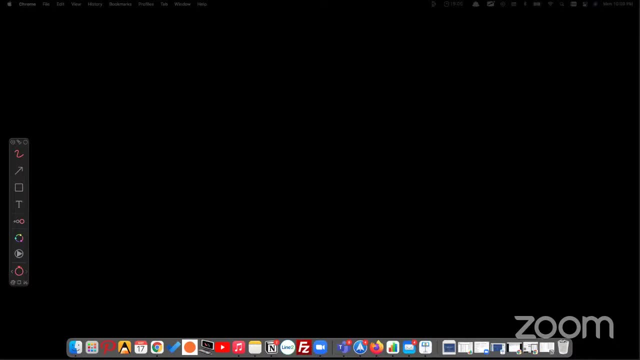 you will be getting that only Okay. so just you have to remember why it's important, because I'm going to train you tomorrow. Very simple Suppose like: if you so, tell me when you use Class C how much IP addresses you get. 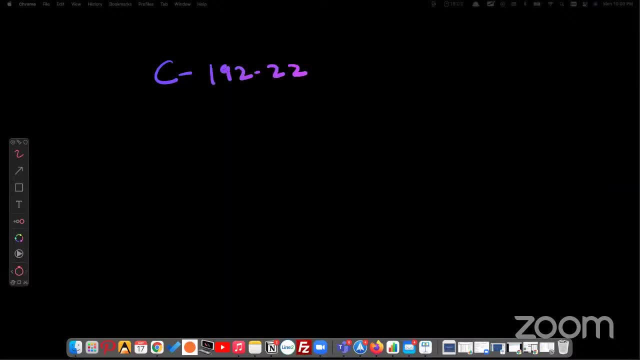 So when you use Class C 192 to 283,, yes, so we had three network bit, one host. So one host means 8 bit to the power of eight is how much IP you give from Class C 256.. But now you don't want to use 250 IP addresses. 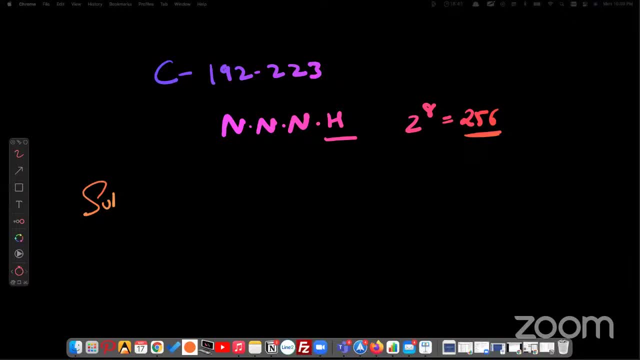 You want to save IP address. So we are going to learn subnetting. So that is to reduce the wastage. why we use subnetting? why every company is using subnetting? to reduce the wastage, to reduce the wastage of IP. Okay, tell me if you have 10 servers. 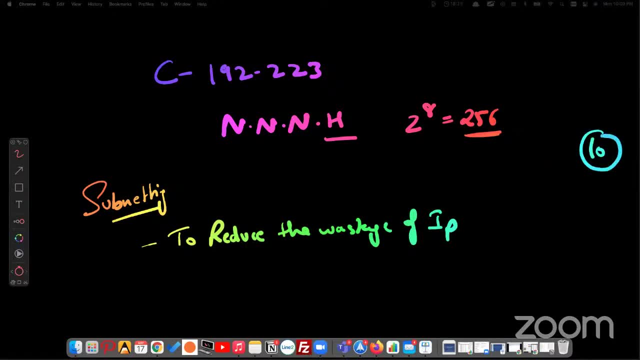 if you have 10 servers in India or maybe in any country. okay, suppose we have 10 servers, but do you guys are going to buy 256 IP? You are recording, Yes, Requirement is only 10.. Are you going to buy 256 IP? 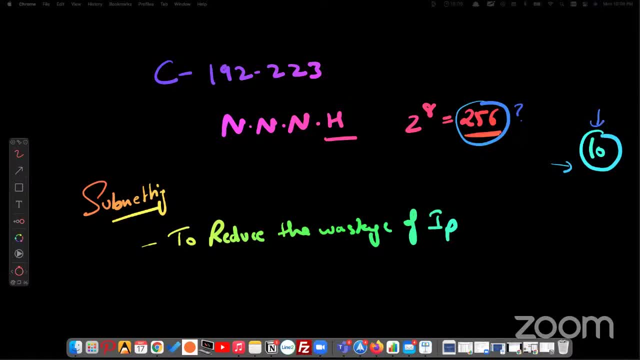 No, Right, So that is not a good thing. So you will directly buy 10 IPs or whatever you require. So the same pattern when we use subnetting. when we talk about public IPs- okay, I'll explain public and private IP also tomorrow. 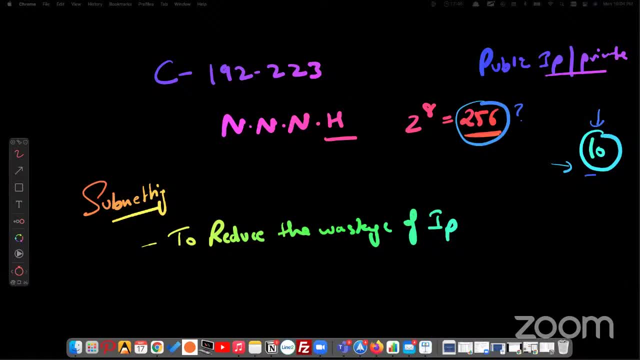 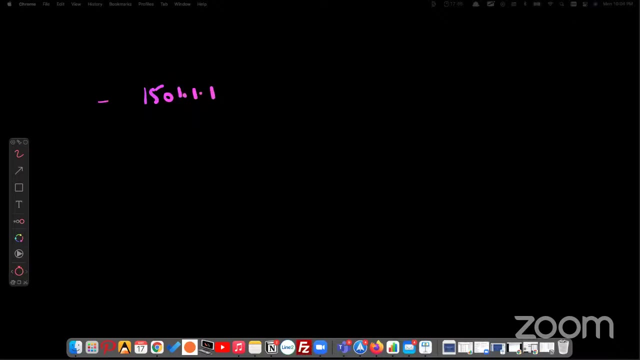 But what you have to do now or today. so just whatever, I'm telling you that please learn the subnetting. Okay, Three things. First of all, whenever I write any IP- suppose 150.1.1.1.. So you should quickly understand: this is class B, 129.1.1.1. tell me which class B class B. 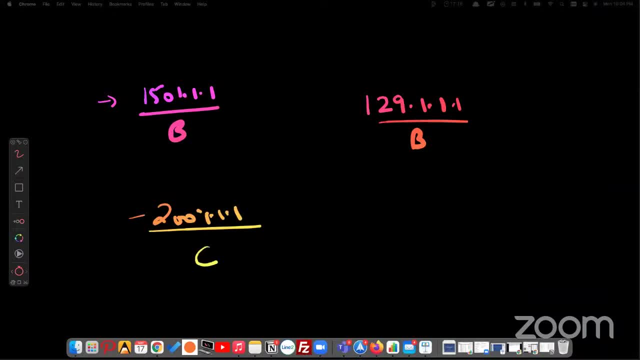 So 200.1.1.1, which IP C? Okay, 17.1.1.1.1.. Class A. So you should make sure that you practice that much. you will be able to identify the IP address and how you identify. just see the first part. 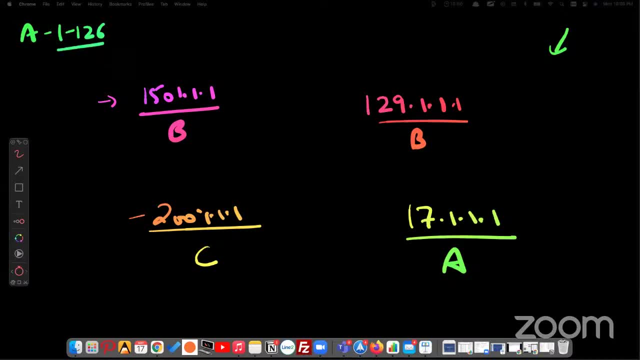 Okay, Only check the first part and you will be able to identify. this belongs to A, B or C. Okay, Got it. Hello sir. Yes, Yes, Sir, Do you have a specific range, A specific range for the public IP assign, or is it any class? 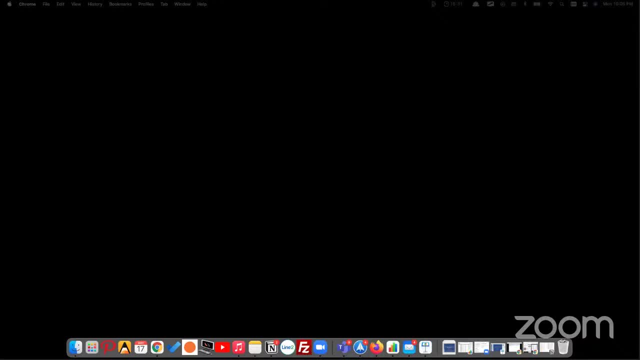 I'll explain tomorrow. Okay, Sub Sing, i'm going to share some notes of submitting. okay means it's just a practice material. let me check if i have, or maybe i'll share once i'll get. okay, i'll check my emails and i'll share with you. okay, on on your email id. okay, 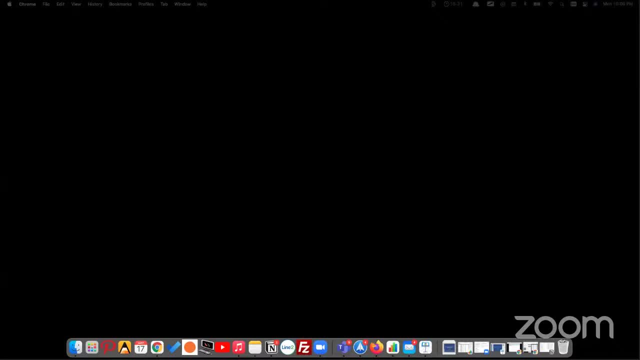 okay, tomorrow the same time in 830. okay, sir, thank you. yeah, how was the session? means you guys got to understand things, or not? yes, and this uh recording will be available on your portal where you have enrolled learnnwkingscom, okay. okay, so we will get any ppt for for this, okay, yeah. yeah, i'll be sharing all material, don't. 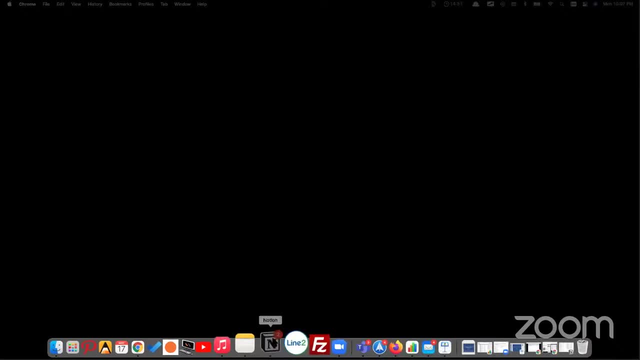 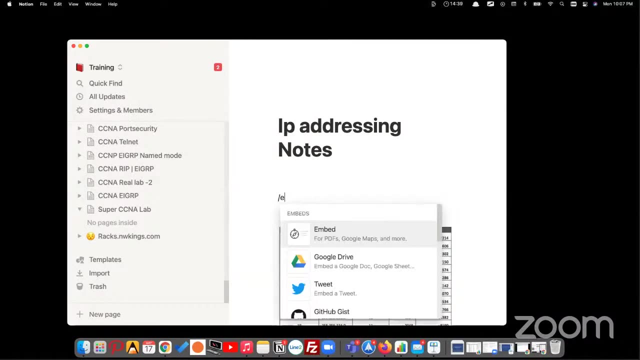 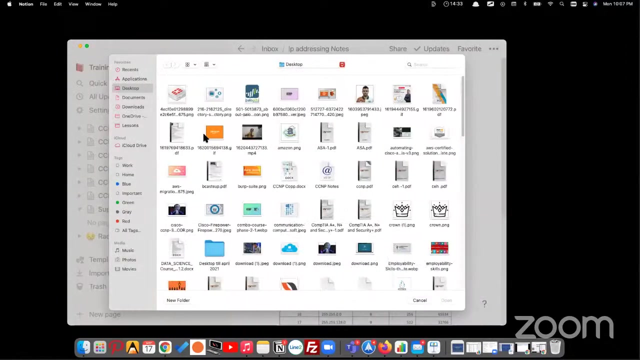 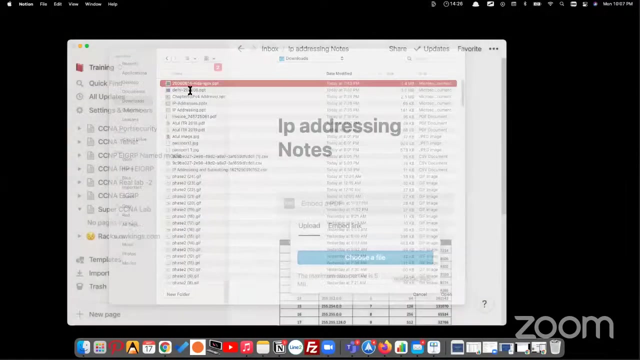 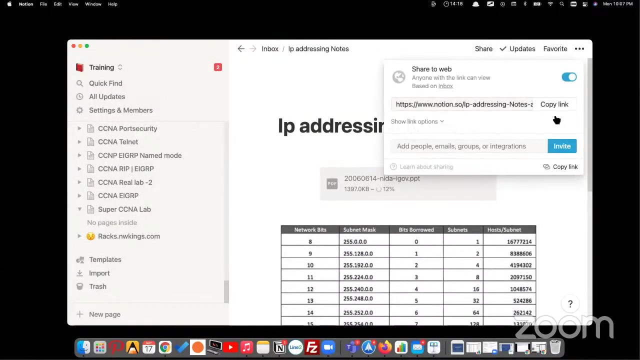 worry. okay, that ppt also and this notes i have already shared. i'm going to share that ppt here only, uh, if i can, uh, just hold on pdf right, it's a pdf, so this pdf is uh, so i have uploaded that. please open that link again, okay. 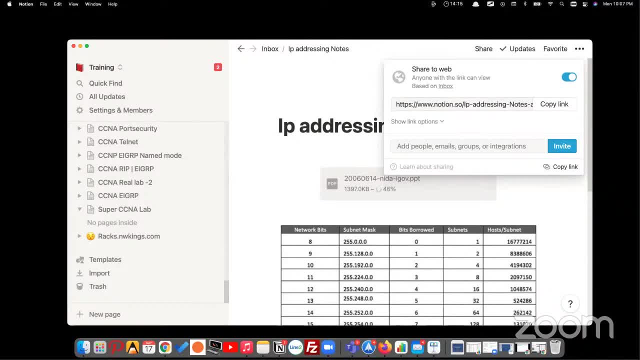 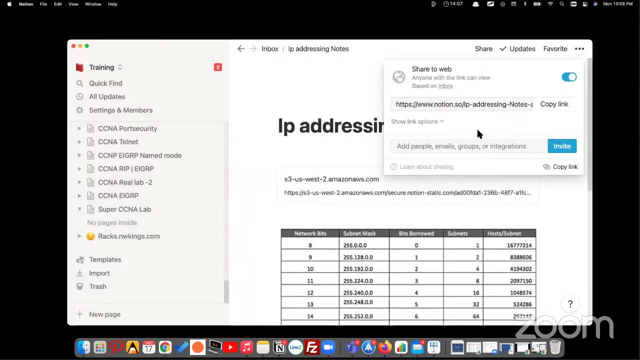 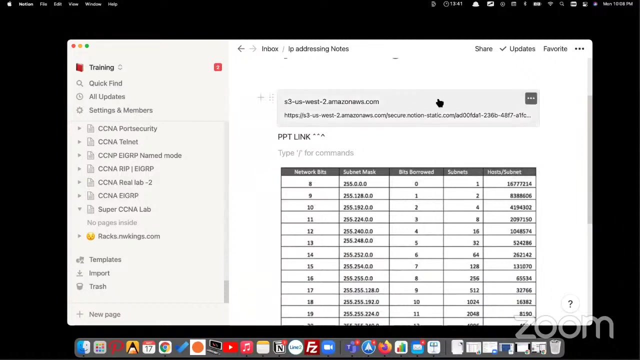 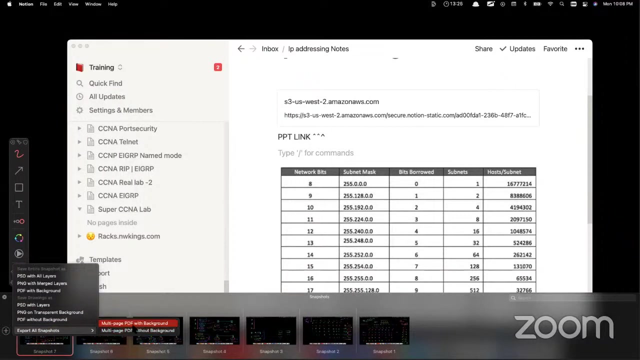 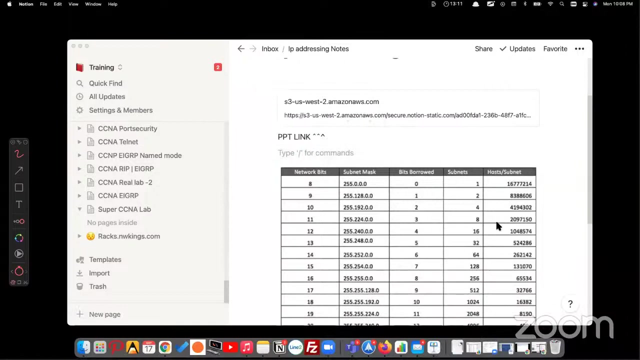 so i have uploaded and you'll be getting soon here. okay, just click here and download this ppt and just, uh, i'm going to share few things. where was that snapshots day one ip addressing? okay, so the notes will be shared with you. don't worry about that thing. that is our usb. 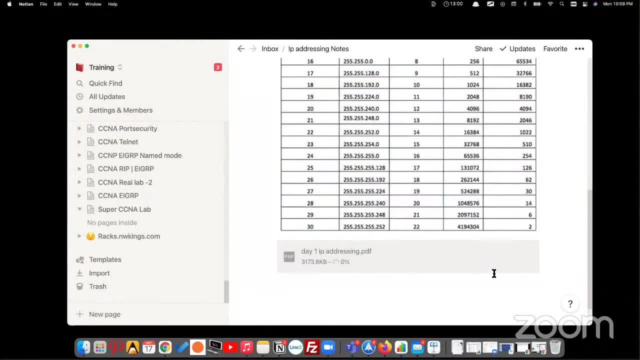 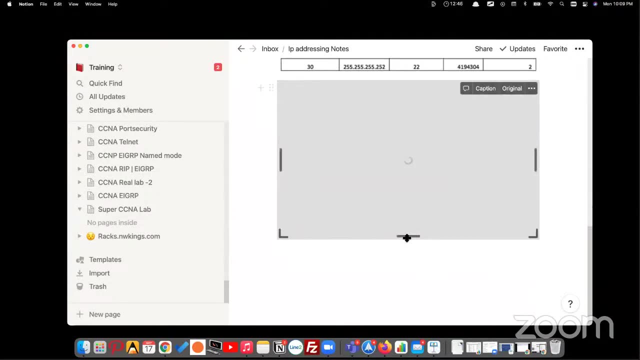 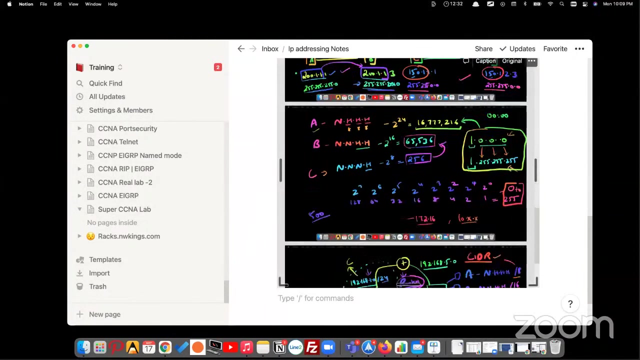 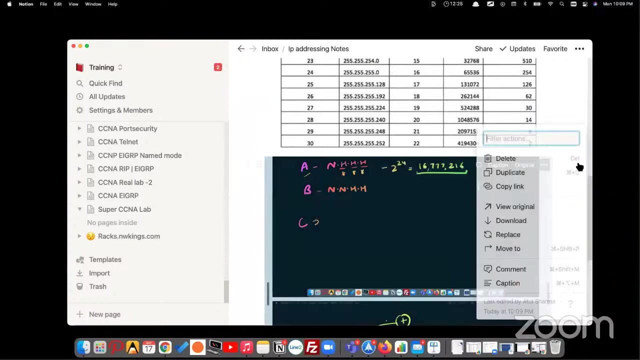 day one, day one. yes, so here you go. okay, so today i have written on my screen, right, so all the notes you will be able to see here got it. yes, thank you. yeah, so you can also download. if you want, just right click or somewhere and you can also download this download. 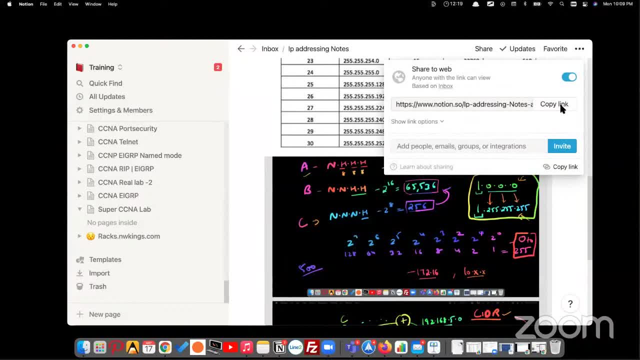 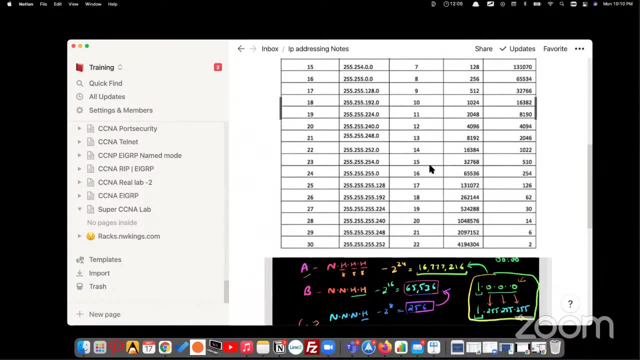 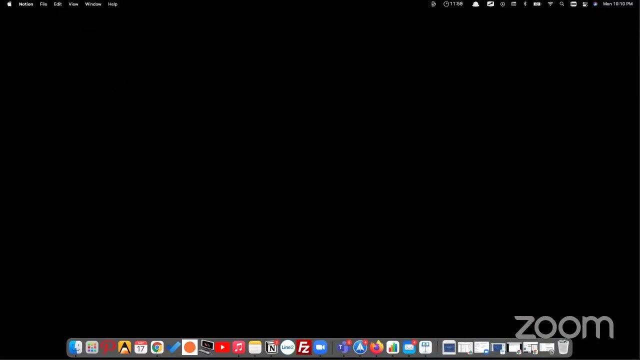 okay. so again, last time, again, i'm sharing this link and i'll try to capture. so just just learn: subnet mask today, okay. so make sure you understand tomorrow this don't cram, don't cram, okay. so. so do one thing, just write. just take notebook and write the phillips like 8, 9, 10, 11, 12, like this, and try to. 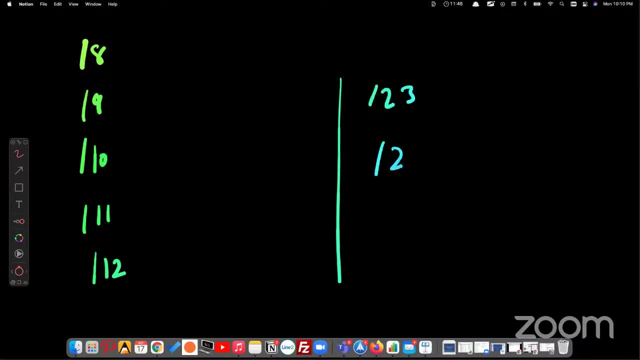 do it to yourself and do randomly also like 23, 21, 20 and match with your chart. okay, the chart i have shared. okay, okay, okay, guys, see you tomorrow, bye-bye, thanks.